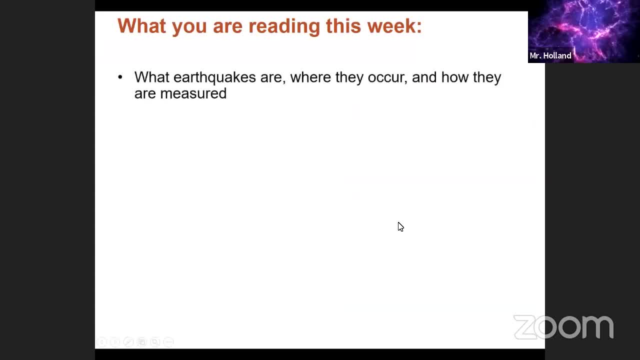 What you're reading this week. the first section you'll be reading about covers earthquakes. I leave a little bullet or a dot in your book in order for you to insert the information: What earthquakes are, where they occur and how they are measured. 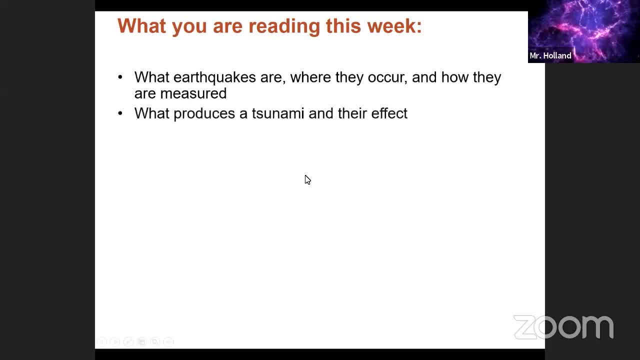 The next section what produces a tsunami and the effect of a tsunami, Three types of volcanoes and how they differ from each other. And the fourth and final section deals with hurricanes: How they form, How they progress, How they die. Tyler, why don't you write right now? 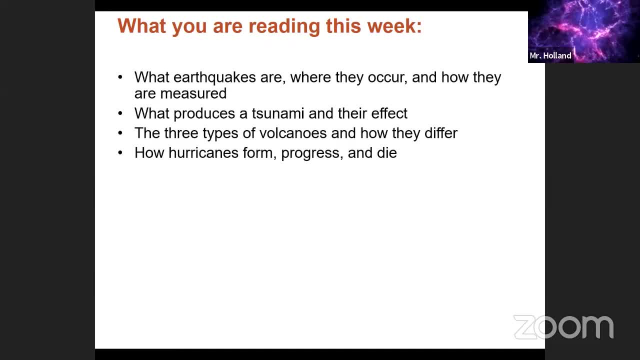 Those are the four topics we'll be looking at in this chapter on natural disasters: Earthquakes, tsunamis, volcanoes and finally, hurricanes. For earthquakes to start us out with: typically, these earthquakes occur at plate boundaries. The plate boundaries are what we worked with and learned about in the last few minutes. 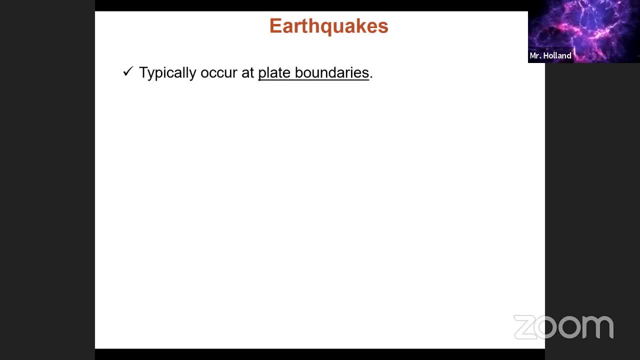 Overwhelmingly. the earthquakes are found on these boundaries because typically this is where two different plates are coming together and there's movement. When the movement occurs, it releases energy and creates an earthquake. The energy is stored as a stress in the rocks. 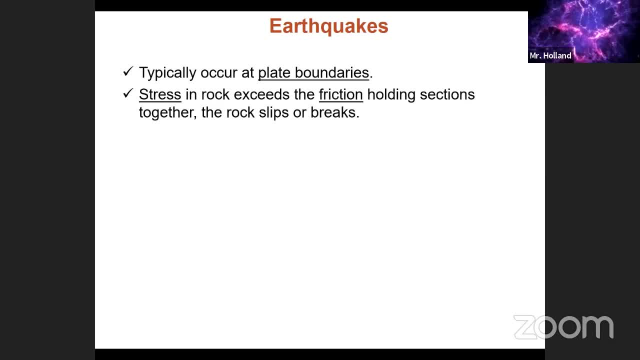 You have the convection currents down in the asthenosphere constantly convecting and moving, making the plate as a whole want to move. Portions of the plate are moving throughout the entire plate except for the edges. The edges are stuck together because of friction. 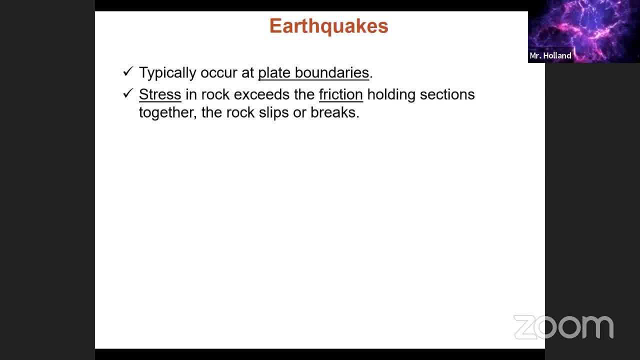 One plate is stuck to the other plate. Eventually that friction breaks loose and the rock either breaks or slips, and that slipping of the two plates is what releases the energy causing an earthquake. Sometimes that slip is only a small distance, several centimeters. 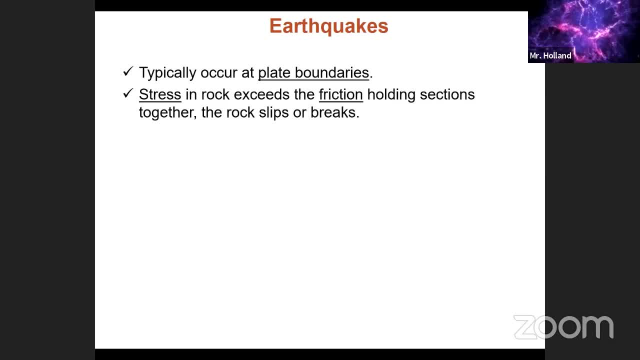 Sometimes it's more than a meter. The greater the slip, the more energy released and the bigger the earthquake that we would experience. The energy stored in an earthquake's rock is called elastic energy. It is released in the form of seismic waves. 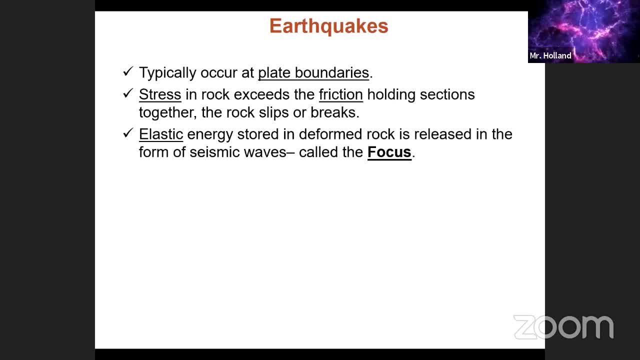 from the place in the ground where the earthquake actually happens, called the focus. The focus is the location deep within the earth where the rocks actually break. Sometimes it's a few hundred feet down, other times it's several miles down. The deeper it is, the less impact we feel on the surface, the less shaking 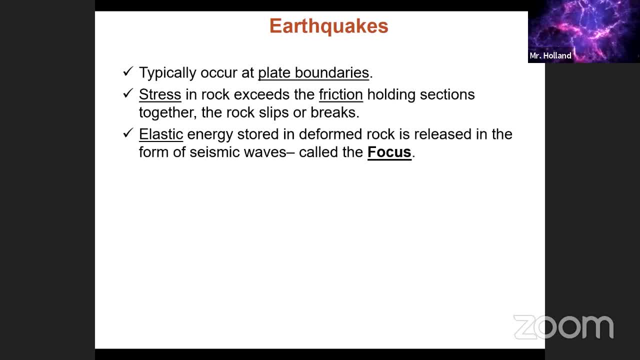 The closer to the surface, the more shaking we feel. The epicenter is the location on the surface of the earth directly above the focus where the earthquake occurred. So when we talk about the location of the earthquake, we're more interested in on the ground: where did it happen? 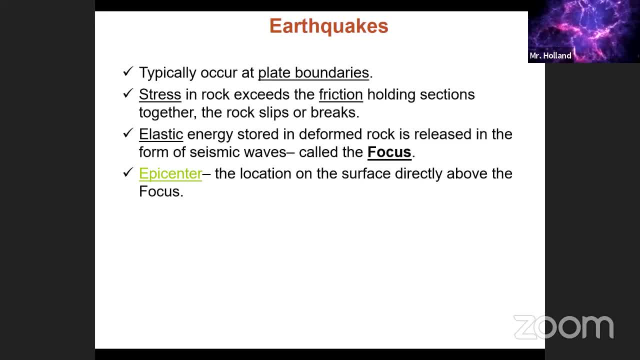 not deep within the earth where the rocks break. Geologists want to know the focus. people want to know the epicenter to locate the earthquake. This little video talks about how an epicenter is located. It's at the base of the Earth's center of the photographs. 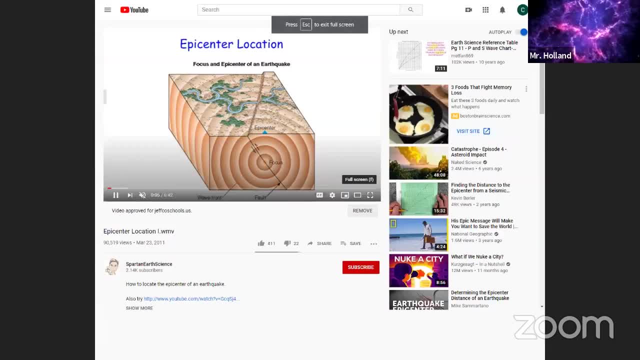 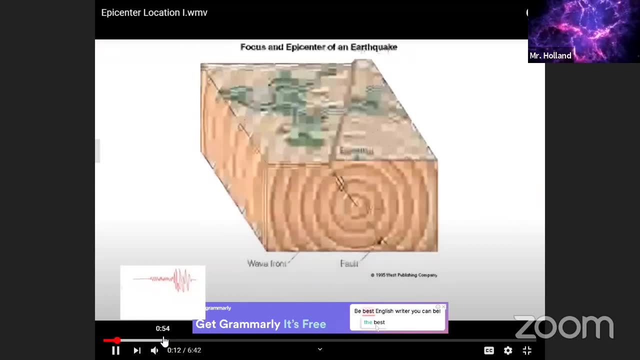 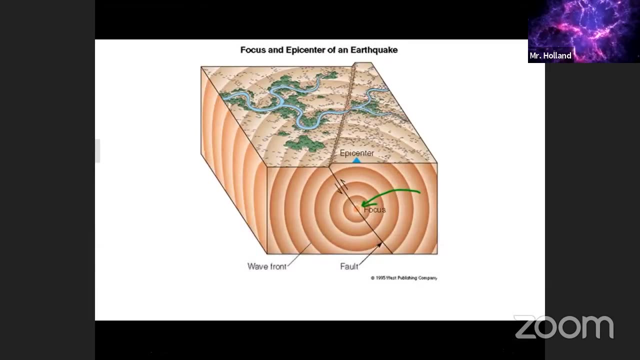 Let's move it up. That's cool. Then look for a near-uh— That's cool. Then that's the point where the rock— to focus on others— In the epicenter. you might try to focus directly above the focus, That's, see the center of what point on the earth's surface directly above the focus. 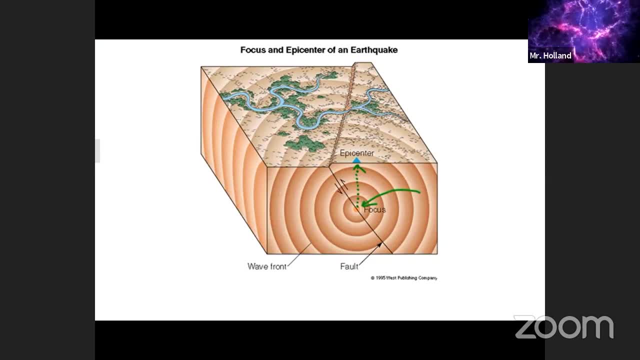 That's probably, you know, working up getting some quite deep scene Miles and miles down below the ground. we're going to try and see if we can figure out where the center is, where on the Earth or the surface is the point of the Earth. 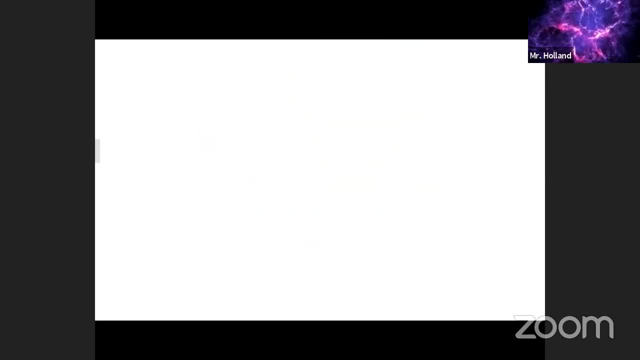 If we can do that, remember we could have seismogram readings where nothing happened. nothing happened and then all of a sudden you get some waves, And that first wave you get there, and the second wave after that is the S wave. 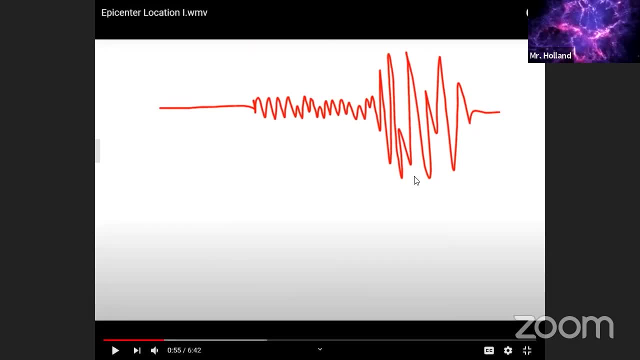 Let's say that this state And waves come into a seismic station. We have one right up the road in Golden. Those waves hit the seismic station. There's a sensor in the ground transferred up into the building and it has big drums of paper that are constantly recording what's going on in the ground around it. 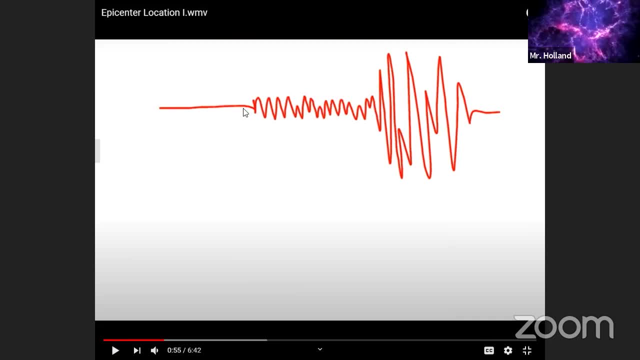 Typically it's just a baseline line that's being produced, But when an earthquake, wave or shaking the ground happens, it makes that line begin to zigzag up and down. That, right there, would indicate the beginning of an earthquake. The arrival of the P wave, the primary wave, is the first wave to get there. 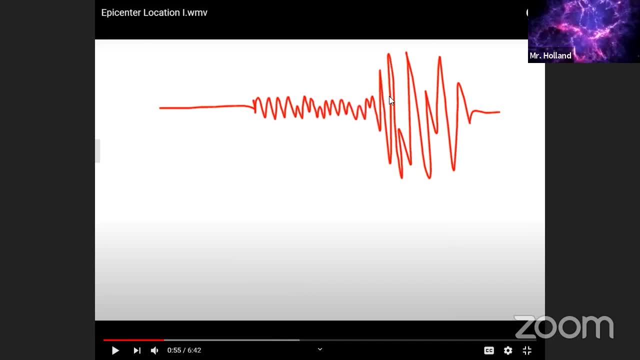 It begins to dissipate a little bit and then it starts up again. This is the second wave coming in, called the secondary wave. The abbreviated is S wave. This difference in time between the arrival of the P wave and the S wave is called lag time. 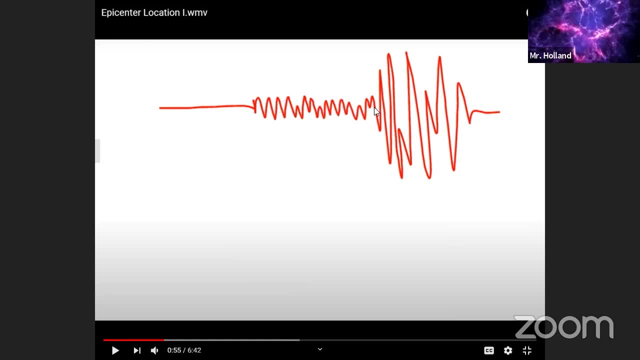 And the lag time is what we have to figure out in order to tell how far away the earthquake was, And that's what this video is going to be talking about. It's the same thing with the second wave, but this station is in the rock dust. 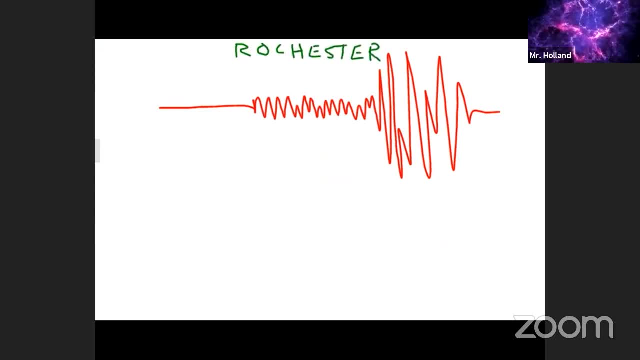 Remember, this is not where an earthquake happened, but this is where the seismic wave started. So the rock dust is then peeling and shaking it off. The body wave, the P wave, the primary wave, the first wave to get there, is there, and the S wave or the secondary wave would come after that, because they're a little bit slower. 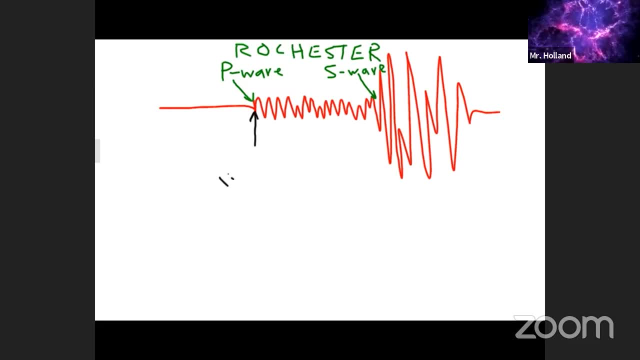 And let's say we have some time down here to figure out what the P wave is back there And exactly what that means. And the second wave is the P wave and the S wave is the primary wave. one o'clock, so one hour, zero minutes, zero seconds, and then the S-wave showed up, and it showed up four minutes after the field, so the S-wave got there at 1-0-4 in zero seconds. so we see that there is a four-minute difference and one of the key points is: what's the difference between the P and the S-wave? there's a four-minute difference between the P and the S-wave and we, as we have been able to do in the past, 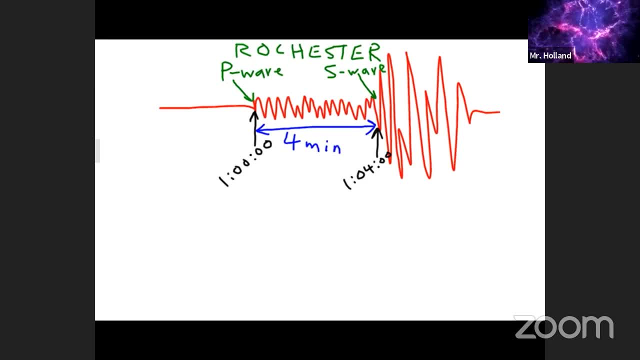 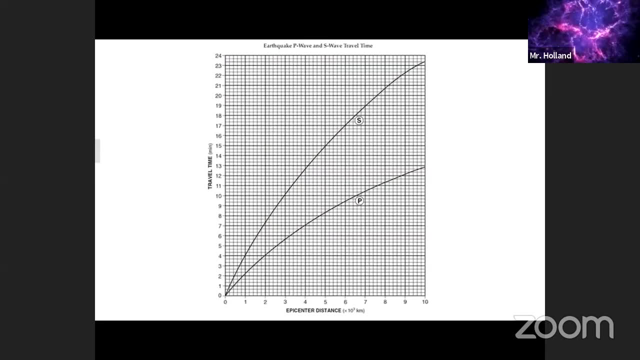 to figure out how far away we are, like we're not just using table 11 of our reference table. we're using table 11 of our reference table, and what we've done before to find a four-minute difference between the P-wave and the S-wave is we've used these graphs. 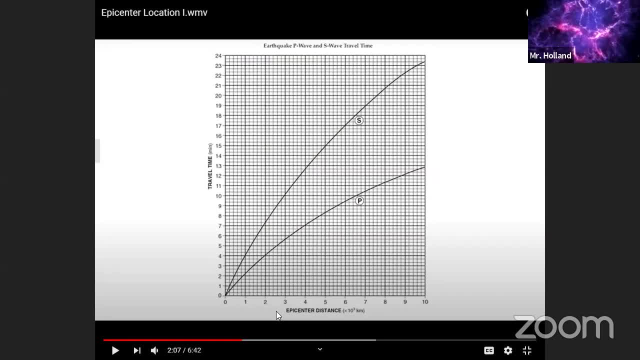 This graph right here is what is utilized to find the distances to the epicenter, which is the independent variable. What we do is we find the time in which the P-wave arrives and the S-wave arrives, and the difference in time is called that lag time. The lag time is this distance between the two curves. 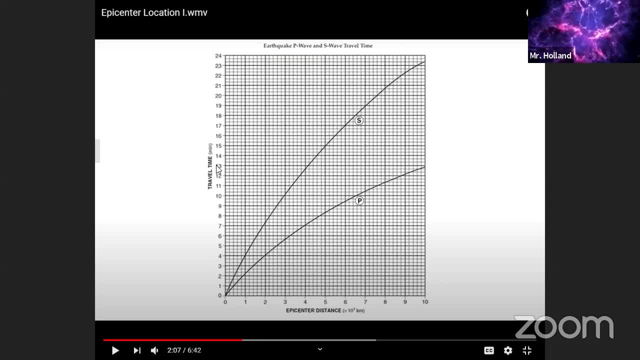 We match up the distance in between the two curves representing minutes of time to exactly what they should be and where that matches up to the exact difference in time. it tells us the distance to the earthquake. For example, in the beginning both waves leave the earthquake at exactly the same time. 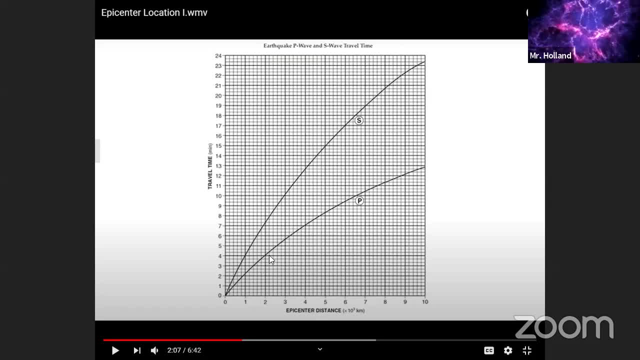 The P-wave travels farther faster, so it gets there quicker. The S-wave is slower, comes in a little bit later. The further away the wave is, or the earthquake is, from the seismic station, the greater this lag time between the two waves Start out very close and get farther and farther and farther. 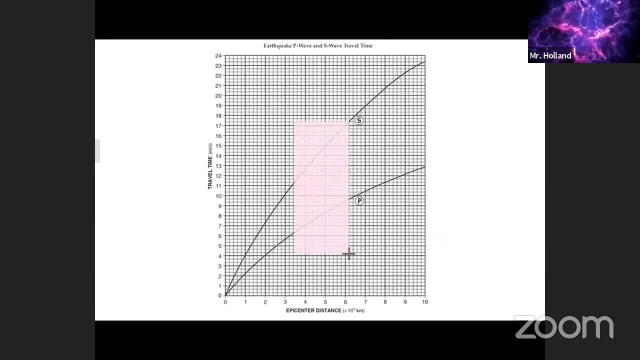 And what we want to do is we want to find out where there's four minutes. So we're going to mark on a scrap paper the S-wave and then the P-wave at zero time, And then, four minutes later, is the S-wave. 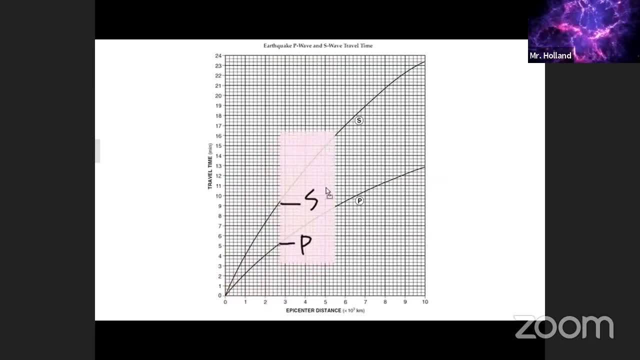 And our next step is to slide this until I find the P-wave and the S-wave And at the difference of four minutes there, look at that right there. So right here I see the P-wave and the S-wave have a difference of four minutes. 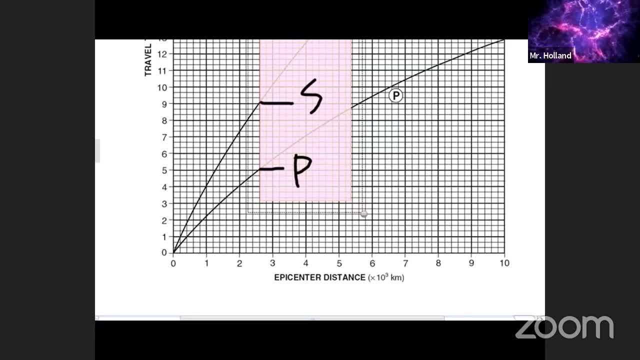 So here I see that P marked lined up with the P-wave line and I see the S marked up with the S-wave line, which means the earthquake is zero time this far away could be right this two, two thousand, three thousand kilometers. so in between there, there. 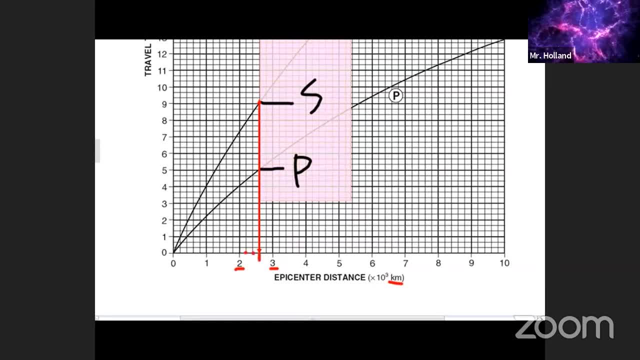 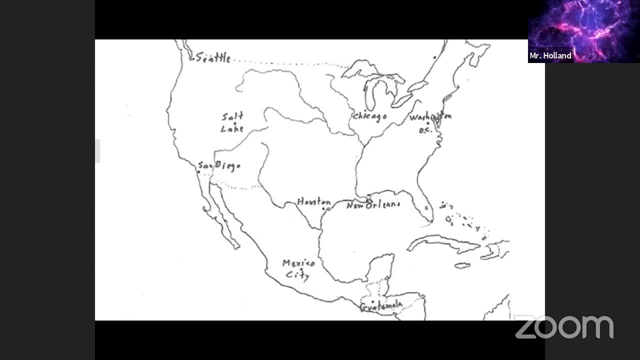 was two thousand two hundred two thousand four hundred. this much right here, two thousand six hundred kilometers away from russia. so here, here, i am, here at the event and here we are, in russia, here, and we know the earth was 3 600 kilometers away from the rock sector and there's a scale down. 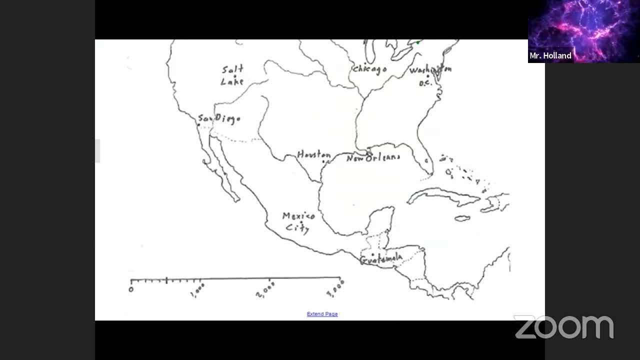 here at the bottom so we could use the scale to figure out where or how far away the earthquake was. not that the problem is: we don't know in what direction that earth was occurred. you know two thousand six hundred kilometers away, but whether two thousand percent of the front is. 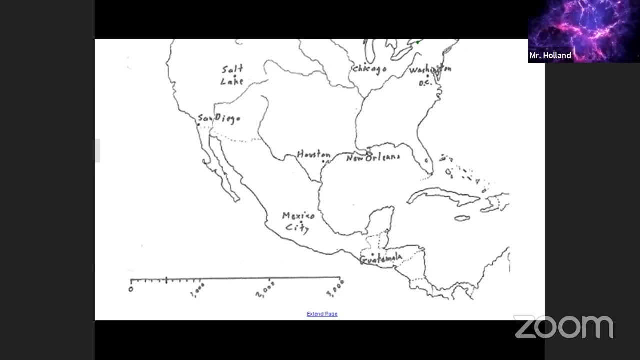 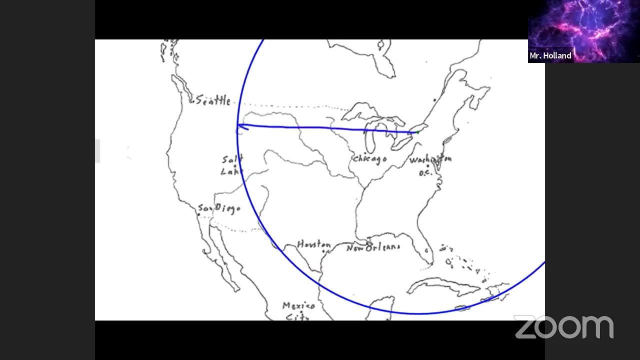 related to the north or to the south, but we're not saying what direction. so what we can do is we can draw a circle around my perspective with a radius of two thousand six hundred kilometers. we know that it will at least be somewhere on that surface. so the next thing we're going to do is we're going to call up some of our friends elsewhere. 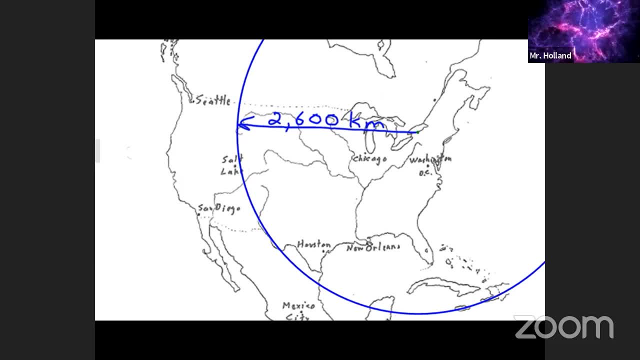 and see if they could also draw a circle here. so we call up our friends: over and now let's keep staying here. so we call up our friends and say, well, what was your size of that station like? and they said, oh well, you know we had a. 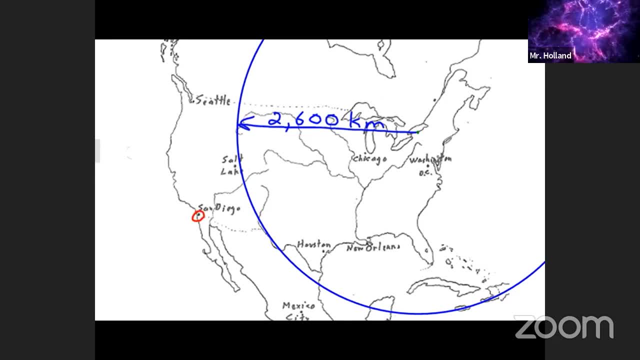 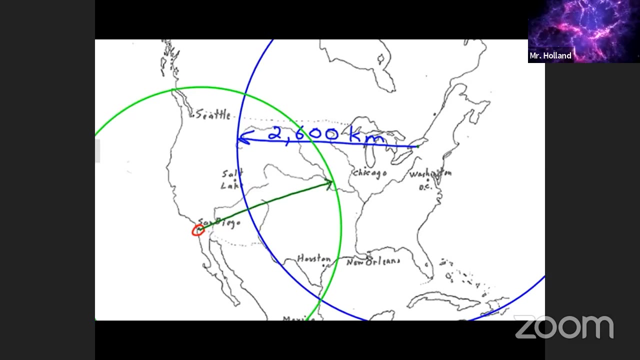 size reference of this time difference is maybe three minutes and ten seconds, and we calculated that to be two thousand one hundred kilometers away. so we're using that circle on san diego and so here's a circle around san diego, that is, uh, three thousand one hundred kilometers. 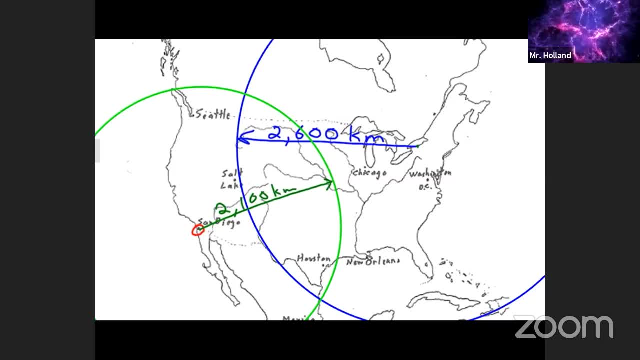 away from san diego. so now we know the earth's place has to be somewhere on the green line and it also has to be somewhere on the blue line, so the earthquake's going to be either right there or the earth's place can be like that. so i'm not talking about inside the circle, it's. 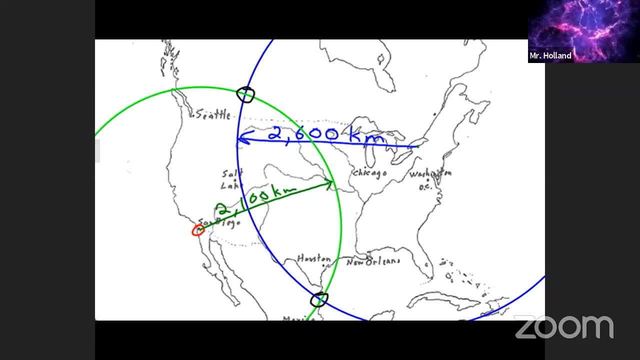 got to be on directly on the circle. so we need one more station, one more location. that has a size of that statement, so we can figure out where this is going to be. let's give our friends up in juneau a call up here in juneau. 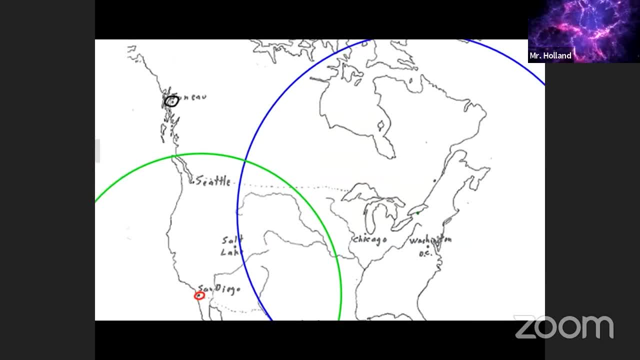 juneau, alaska, and we'll say, all right, hey guys, you got it. did you get the keywords in the episode from the airport? yeah, we did. you know what was your time difference to give us this kind of effect calculated with this? and our friends in juneau say that maybe it was- uh, you know- 1 500. 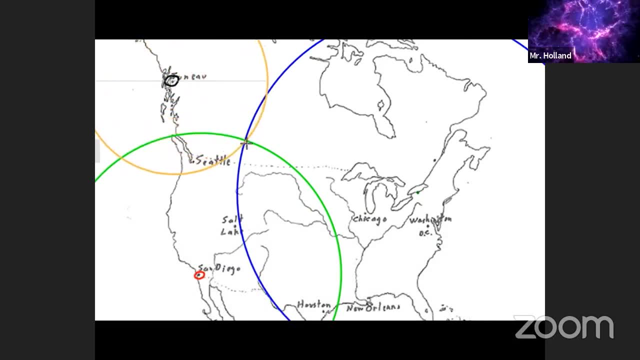 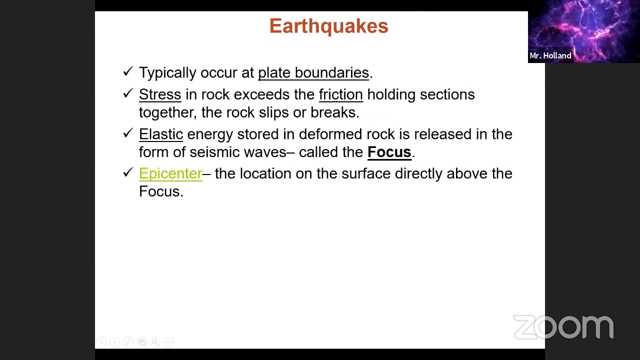 and when we measure that what will happen is, those circles will all meet in one area, and that's the point where the earthquake happened. this had to be 2 600 kilometers away from rochester, and it was. it also had to be two thousand one hundred kilometers away from san diego, and we see that. 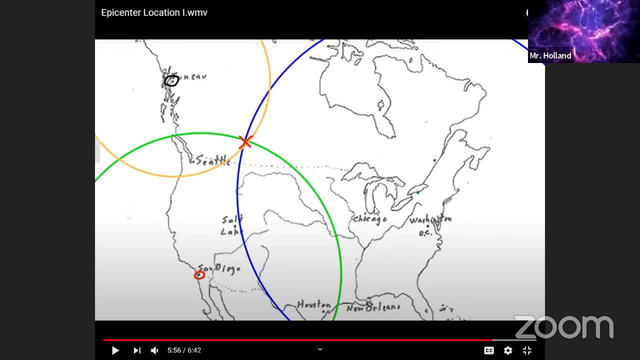 this is what we call the epicenter. when you have three places to locate it. triangulating your position can be done if you know the distances, and the only place where all the distances from each sizing station are correct is right here in this region. the more precisely you make your measurement. 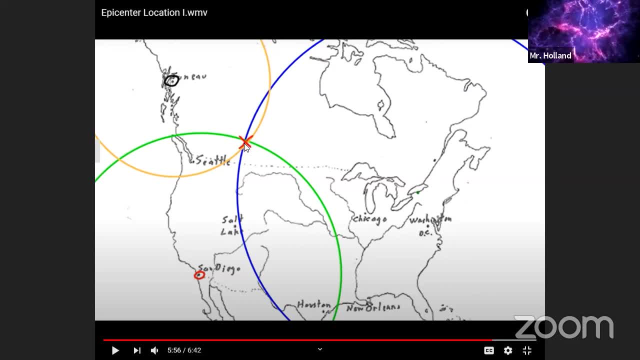 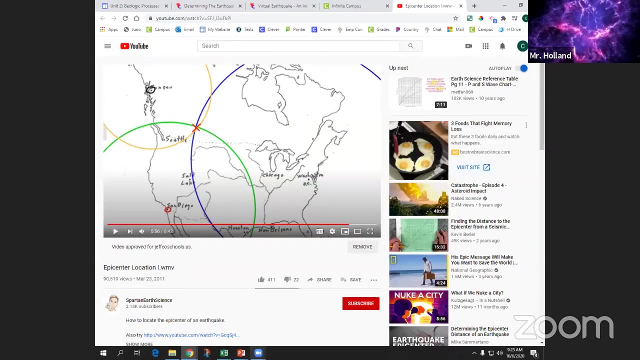 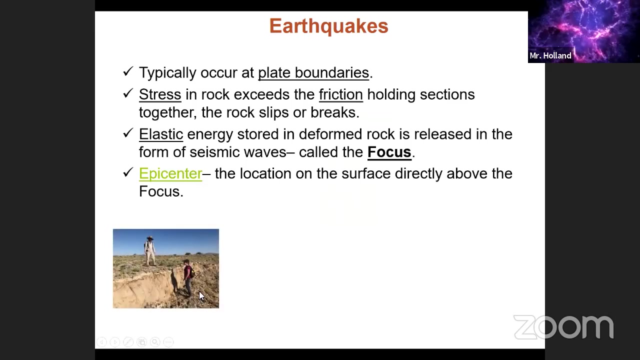 the more it narrows down that region to a smaller and smaller point. questions about that epicenter location at this point. we'll go into a much more detail with the tutorial on thursday. let's exit out of that. this earthquake right here occurred in the mojave desert in california. 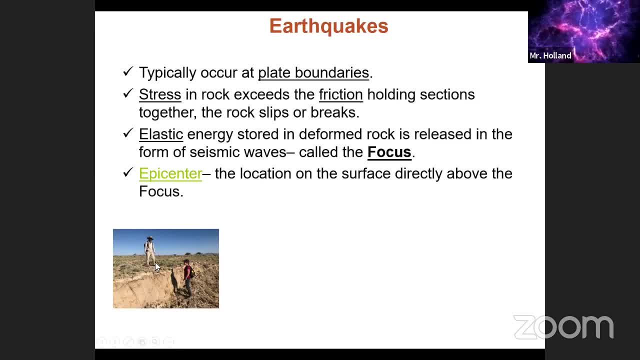 2019. it was july 5th, so just last year. the earthquakes themselves do not have to cause a side-to-side movement. this one caused an up and down movement. one side moved up, one side moved down, and the difference of displacement was about one meter, a little bit more than a meter. 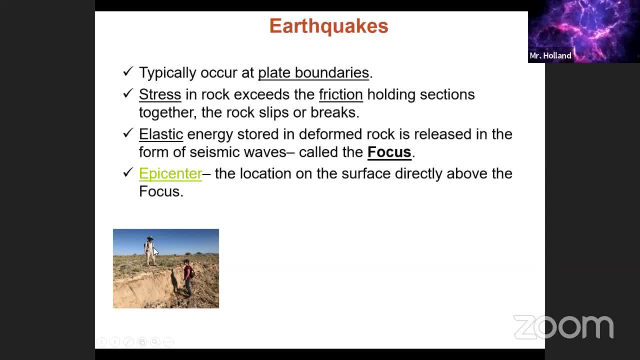 and you can see the person standing on one side of the fault here and the other side of the fault here. this her earthquake came up to be about. it was a 7.1 of magnitude. it also caused much road damage in the area, because the roads are just laid down on top. 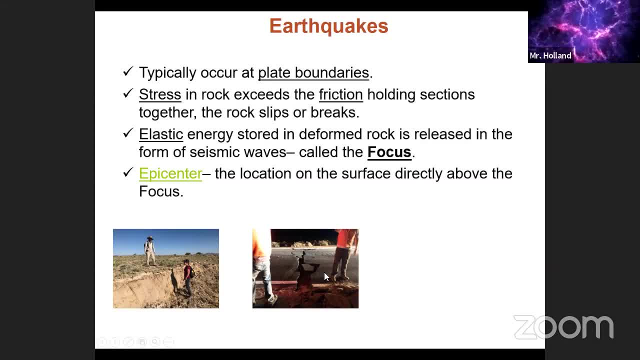 of the sand. when the sand moves, it causes the roads that don't move so well to just break and crumple. that's what we had happening here this right. here is a picture taken from space of this 2019 earthquake. it shows a couple kilometer. 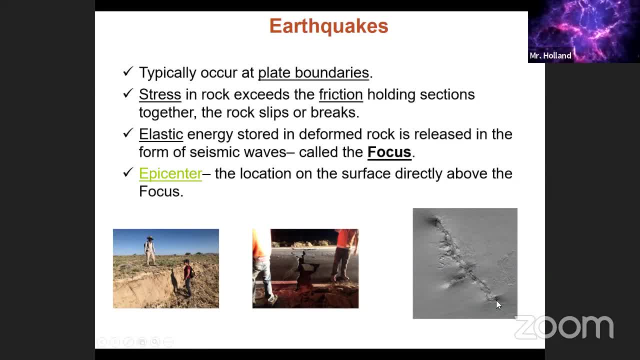 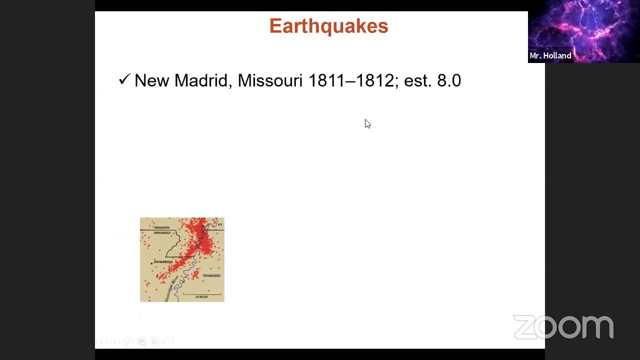 long scar that was created on the surface of the earth in the mojave desert or this occurred. there are three major earthquakes that you should be aware of historically. 1811 to 1812, it was the new madrid missouri earthquake, estimated to be an 8.0. at this time we did not have any way of. 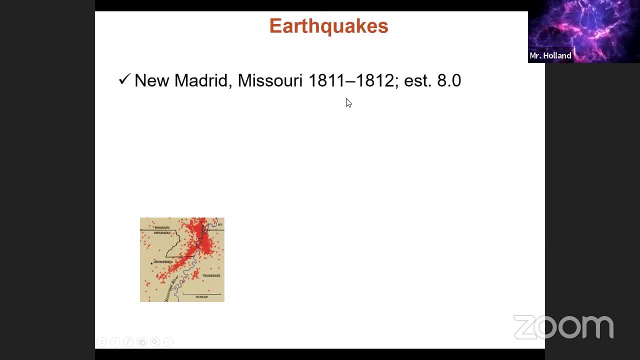 measuring the earthquake's intensity or magnitude. so we decided to. we're just going out and etching the earth versus theadoe to estimate it based on what the people were saying at the time, what they experienced, the testimonials. It was a rare magnitude or high magnitude earthquake, because it happened. 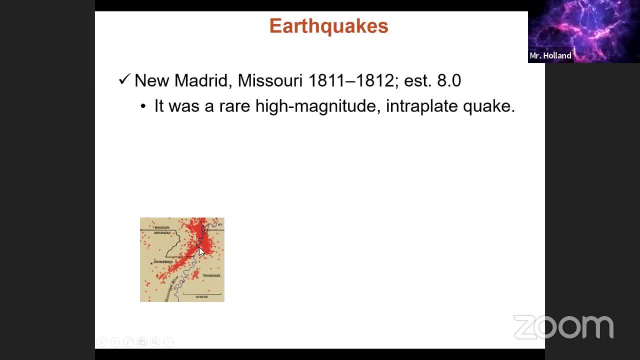 in the middle of the plate in Missouri. You can see all these red dots here. These were aftershocks and foreshocks of the earthquake that occurred. But in the middle of the North American plate- Missouri, Arkansas- you can see in here Tennessee, on the side That's. 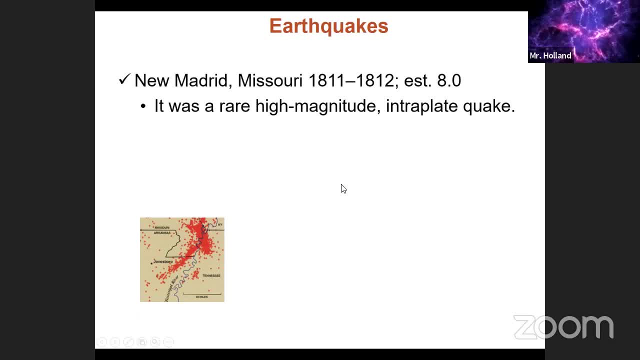 rare, because typically earthquakes happen at the boundaries and this is not a boundary. However, the whole plate is moving, but the edges are locked in place until they jump past each other, So that creates a huge amount of stress. Sometimes that stress has to be. 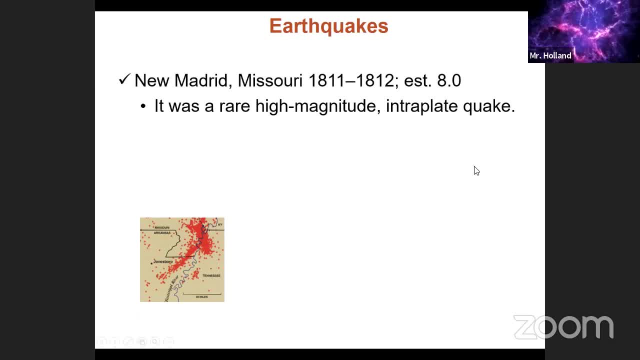 alleviated and it happens in the middle of the plate, and this is one of those times. It caused 150,000 acres of forest to be destroyed. The next earthquake that's kind of famous is the 1906 one. We did have our first measurement scale at this time, called the. 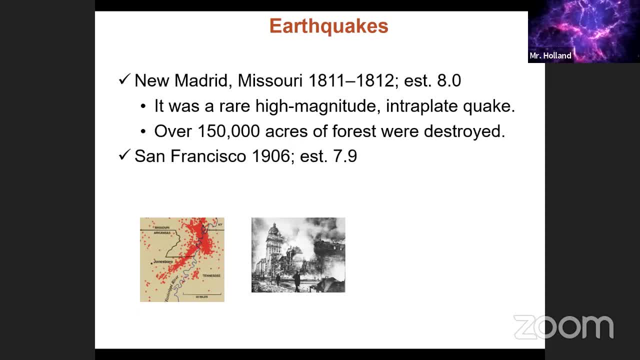 Mercalli scale of measuring earthquakes and they estimated from that that the earthquake is about a 7.9.. This is a picture of it down below here. In earthquakes the shaking of the ground causes a lot of damage, but also it causes other things to happen. For example, at the time 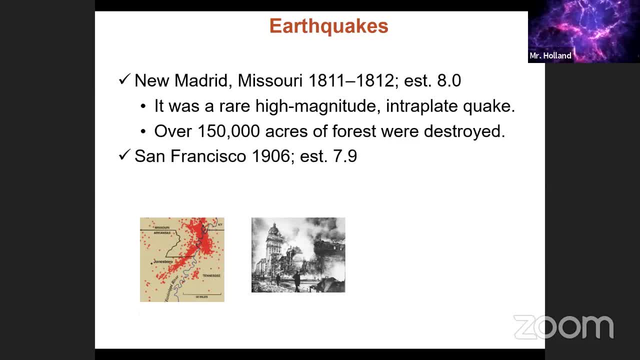 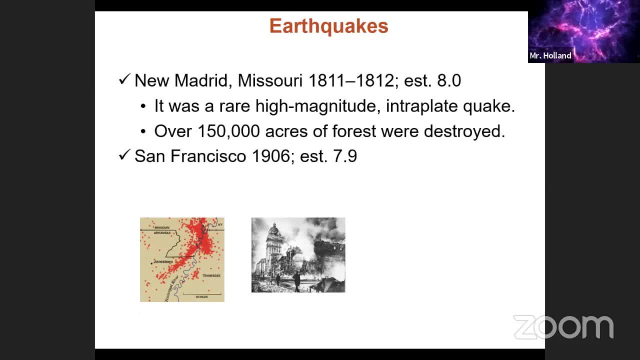 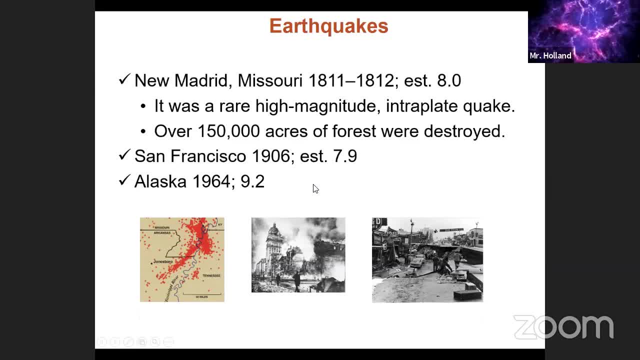 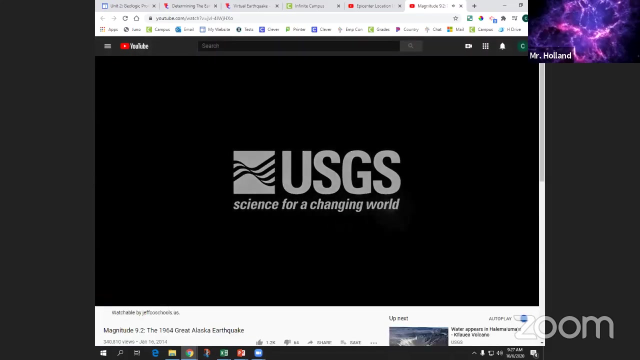 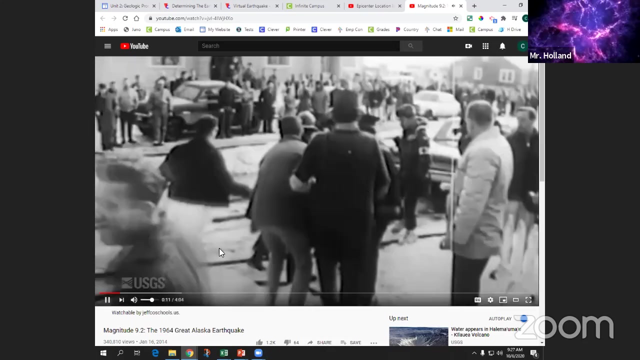 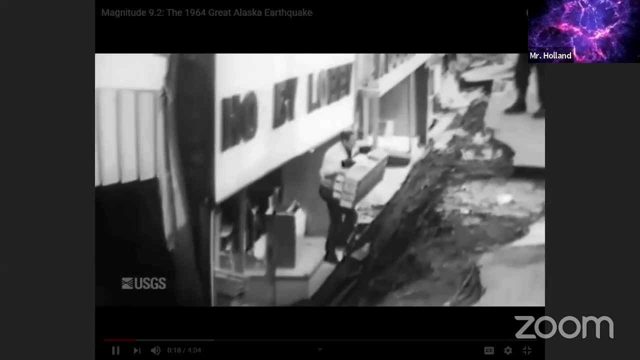 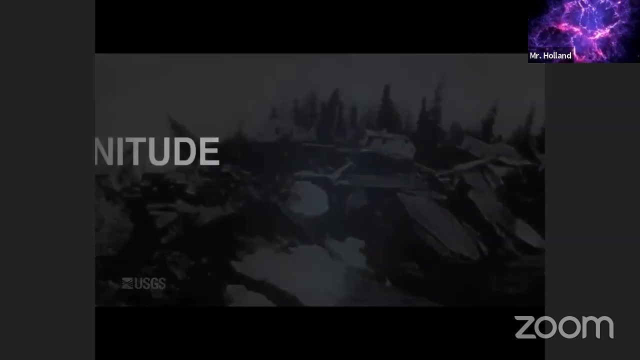 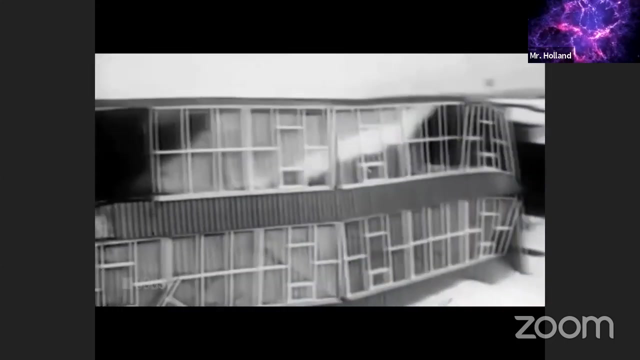 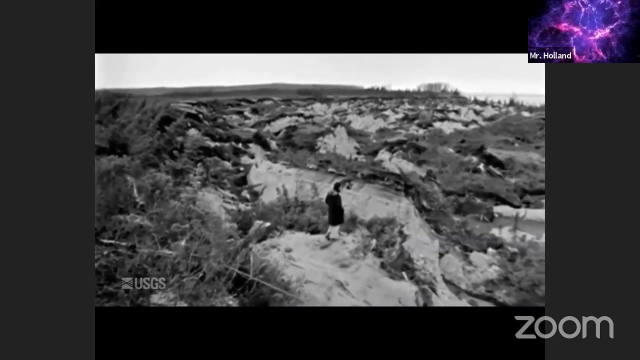 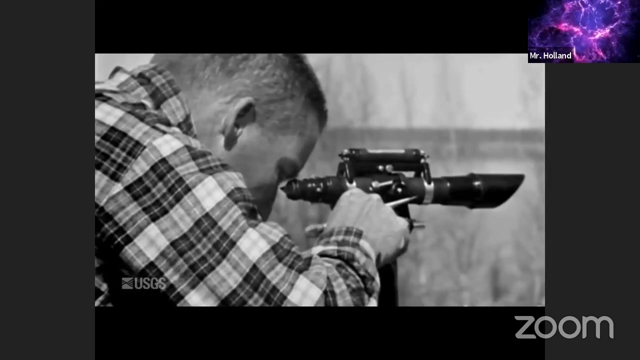 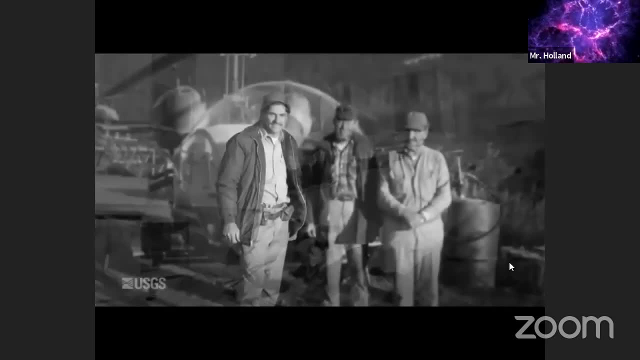 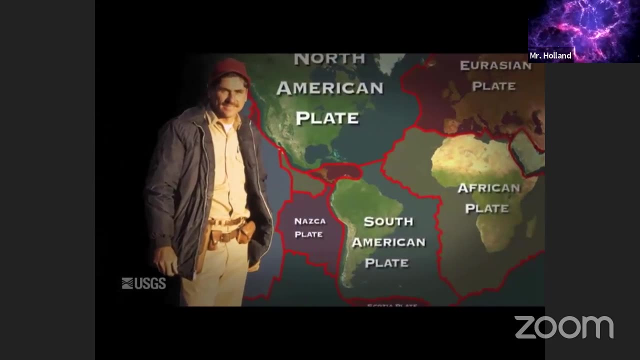 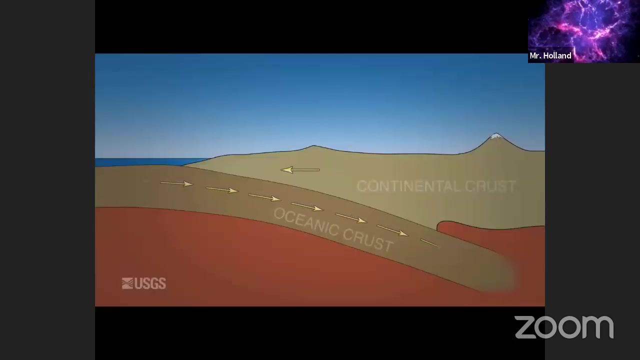 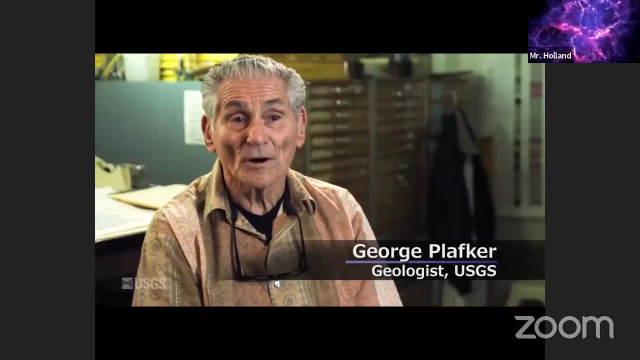 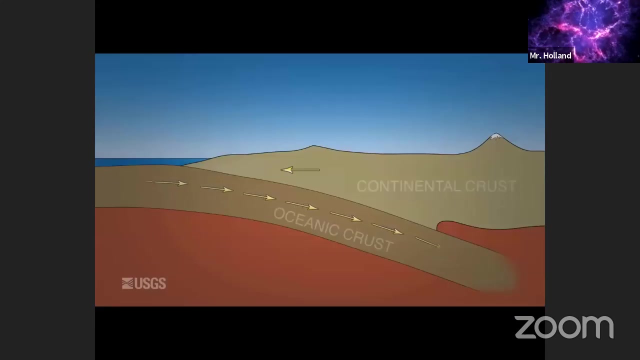 The oceanic crust is being pushed underneath that part of Southern Alaska at a very low angle and there was slip on the interface between the oceanic crust and the overlying continental crust. These two crusts are converging at the dramatic rate of an inch and a half each year. 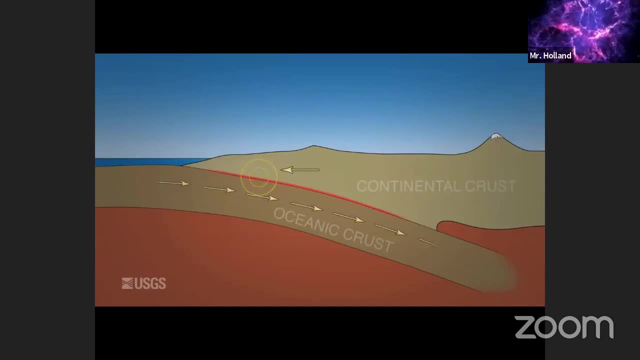 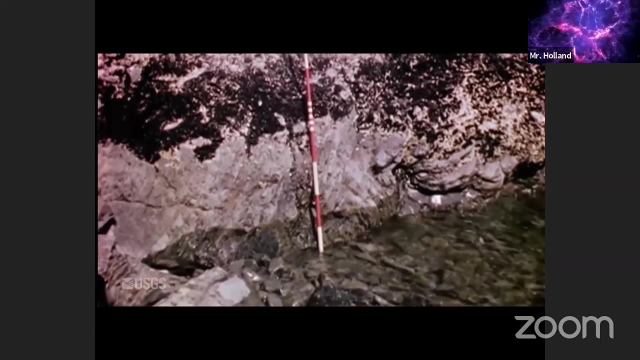 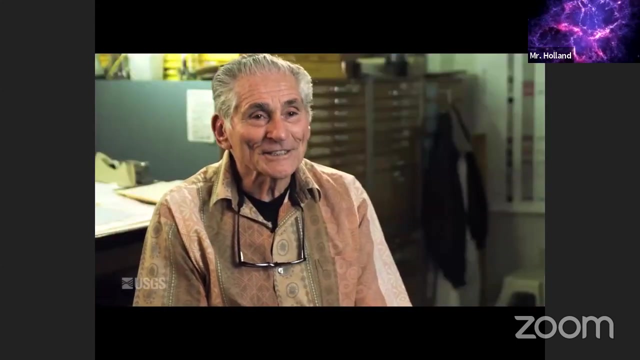 Periodic slip between the crust produces great plates, which doctor called megacrust earth plates. Scientists now recognize the distinctive patterns of uplift and downdrop at the earth's surface. What is with these plates? One of the obvious things that everybody wants to know when you have an earthquake like this. 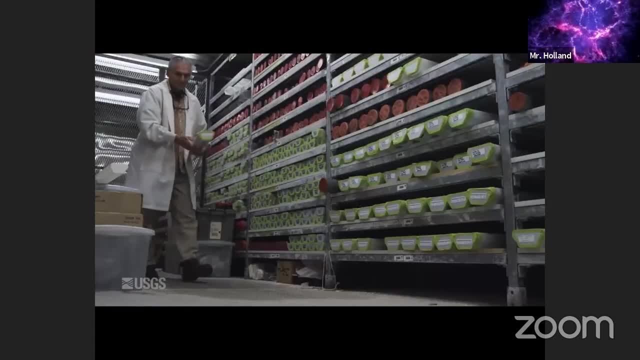 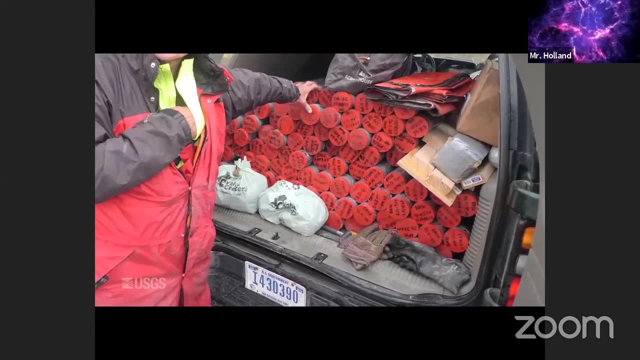 is: how frequently do they occur? Do you have one tomorrow or thousands of years? By drilling 50 feet into the earth and taking core samples, discovered nine megacrust earthquakes that have occurred in South Central Alaska over the past 50-500 years. 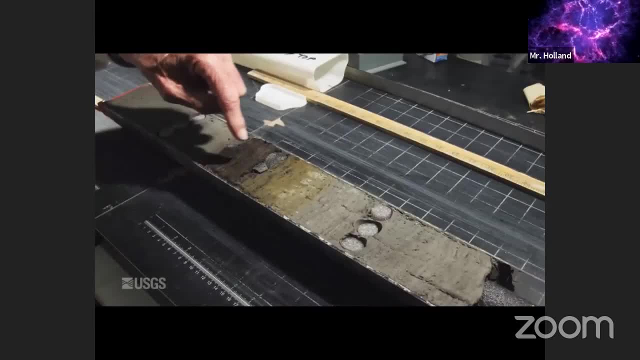 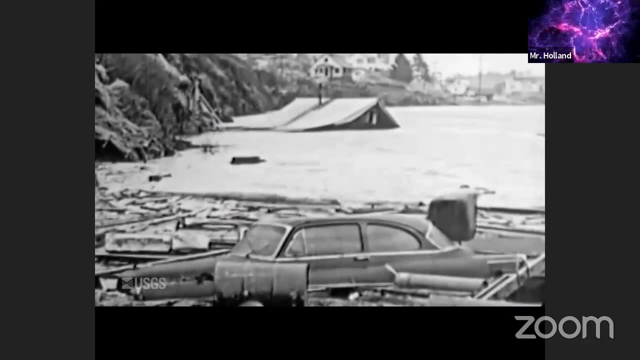 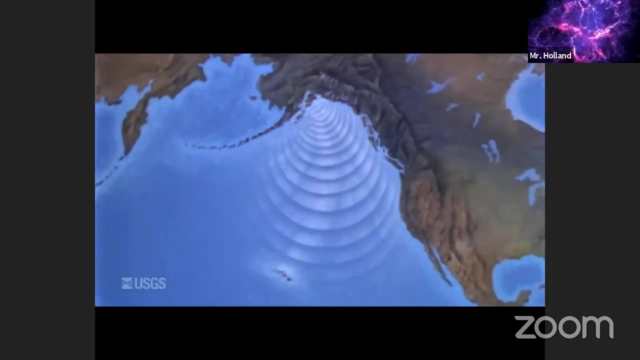 The average time span between these earthquakes is 630 years. The 1964 Great Alaska earthquake was accompanied by massive tsunamis. Within minutes, one created a wave 20 stories high in Parkland. Some traveled across the Pacific, leaving havoc in coastal Oregon, California and 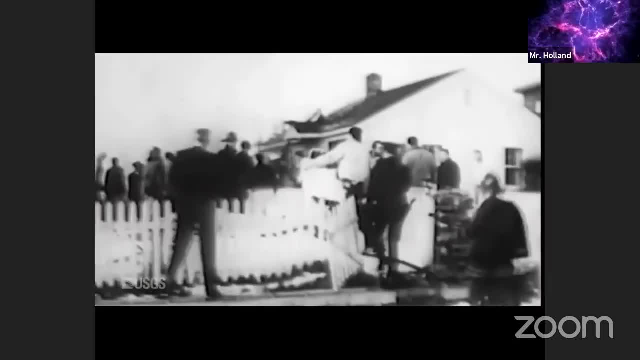 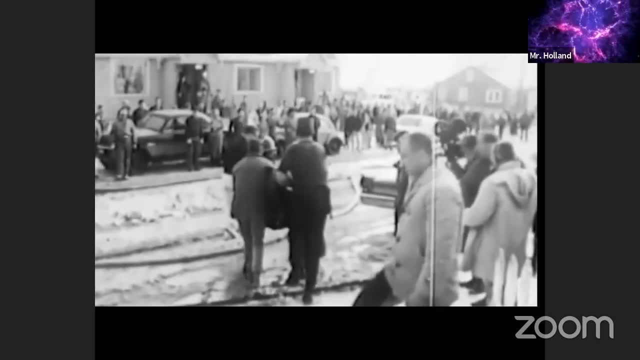 Hawaii. The widespread damage and loss of life from this earthquake led to a determination to use science to save lives in the future. South Central Alaska. here is the infrastructure center of the state and it's also by far the largest population center in the state. 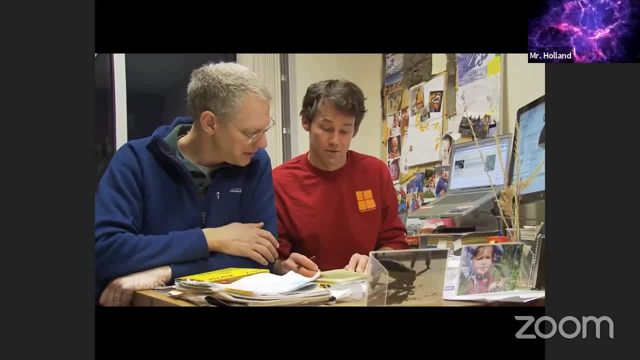 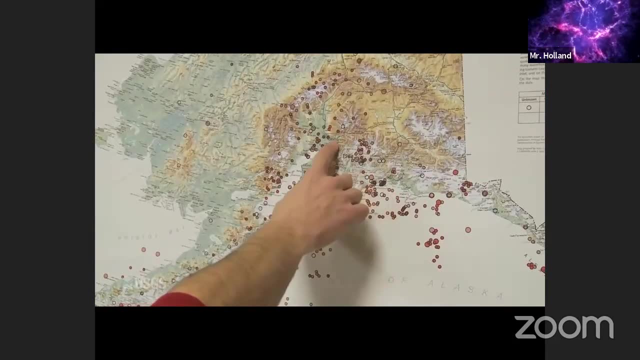 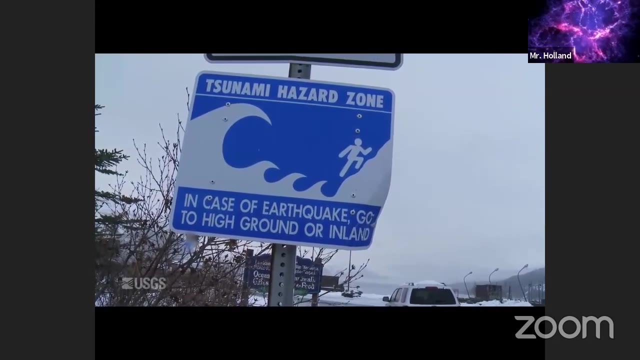 And the work that we do involves the fundamental characterizing of the earthquake hazards, knowing which faults are active, which faults improve earthquakes, understanding how often earthquakes occur, And another part is understanding the local tsunami hazards. Regacies from the 1964 Great Alaska earthquake and tsunami include the USGS Earthquake. 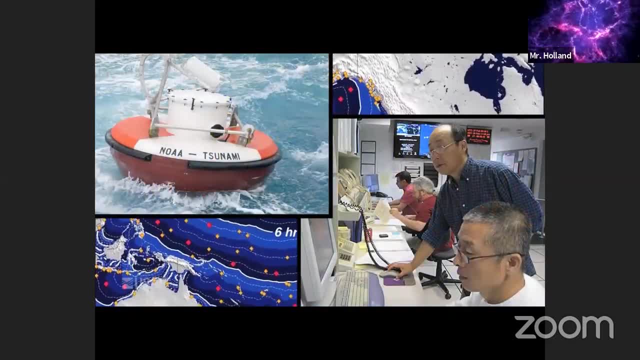 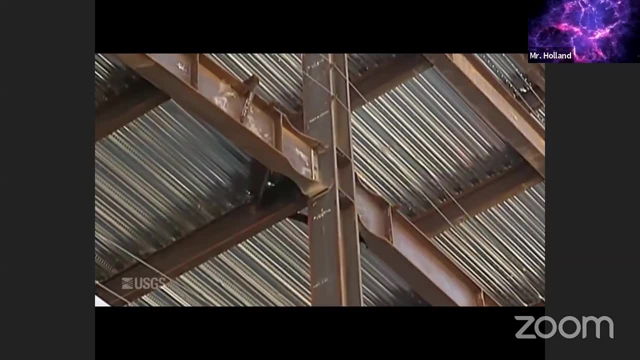 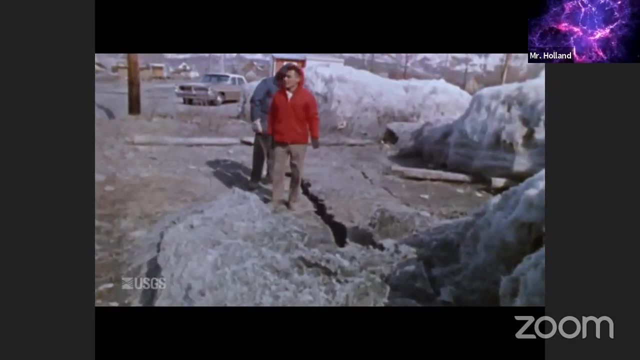 Hazard Program, NOAA Ground-to-Clock Tsunami Warning Centers, the Advanced National Seismic System, resulting in seismic hazard maps and improved building tags. All together, these programs can help predict strong ground motions from future earthquakes and minimize risks. For one example, scientists learned that boundaries were so unstable and at such risk for earthquakes. 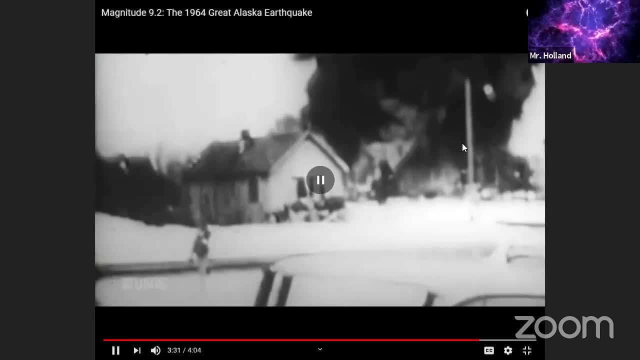 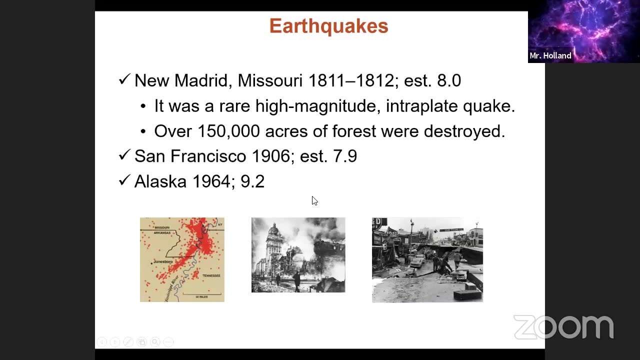 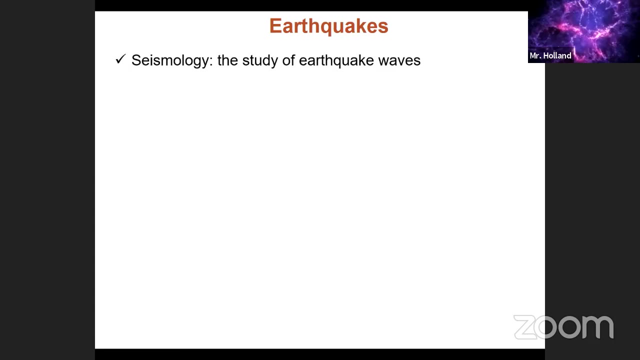 that the town was moved. Let me go ahead and stop that one there. When we study earthquakes, we're studying something called seismic hazards. We're studying something called seismology. Ology is the study of seismic, and seismic waves is the size part of it. 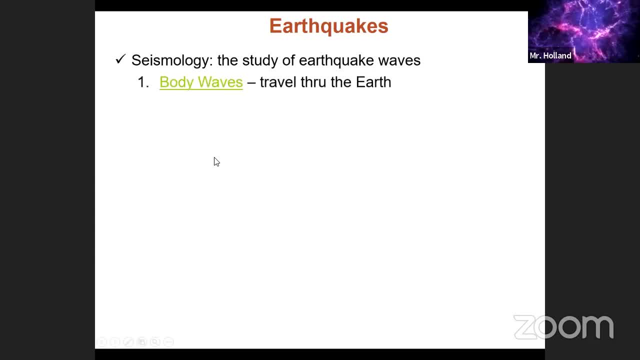 Seismology, So we're studying earthquake waves. There are two types of earthquake waves. The first type is called a body wave. Body waves are the ones they were talking about in that first video, the SMP waves. They are able to travel through the earth and they get to distant locations in seismic. 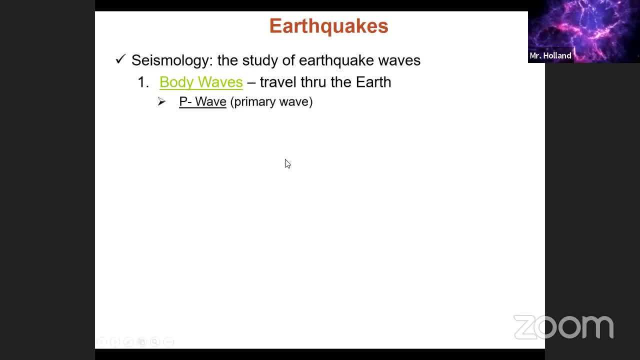 stations. The P wave is the first one to arrive because it's fastest. It's the primary wave. This is what we call a longitudinal wave. It causes the ground to move forward and backward as the energy wave moves forward through the ground. So if you were to look at a picture of this, it would have the ground being compressed. 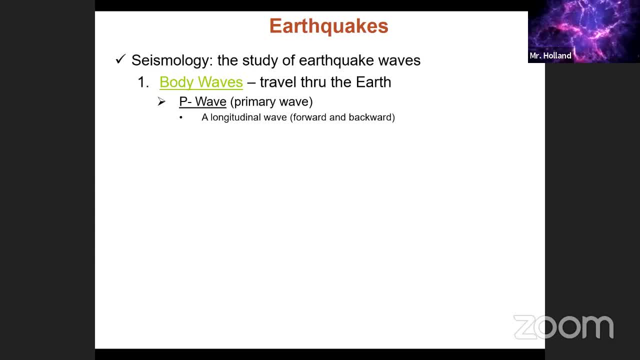 on the front edge of the wave and stretched on the back edge of the wave, so that compressed and stretched is what takes place in the rock as the wave moves through the ground. Called longitudinal, This one could go through anything: Solids, liquids or gases. 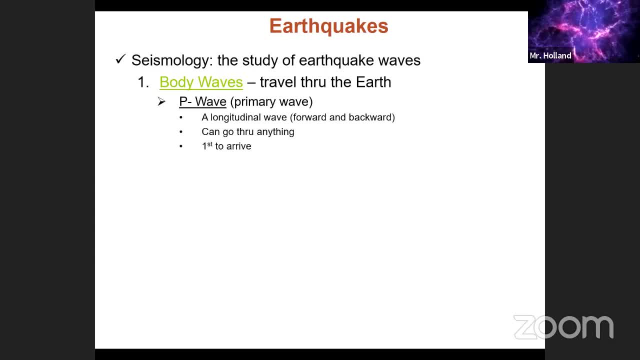 They don't stop it. And again, it is fastest. so it's first to arrive at seismic stations. The next one is the S wave, called the secondary wave. It arrives second. It is a transverse wave. This means it's a side to side wave. 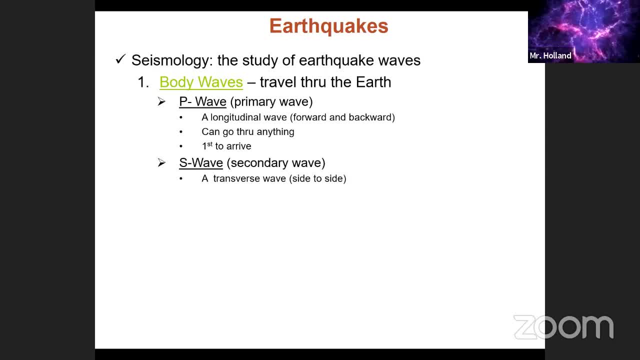 It makes the rock and the ground shift side to side. Since it's not all moving forwards and backwards, it has a greater distance to move. Therefore, it's going to take longer to get to different locations. That longer travel time is why it comes in second. 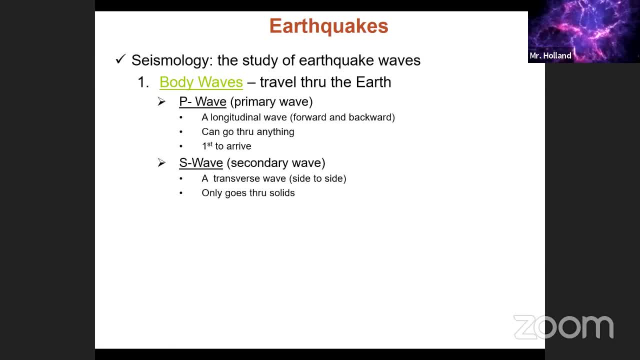 This one also went through solids. So when we look through the earth to find this one coming through the liquid outer core in regions of our earth stopped the wave and we see nothing coming through the other side of it. So the S waves don't make it to the other side. 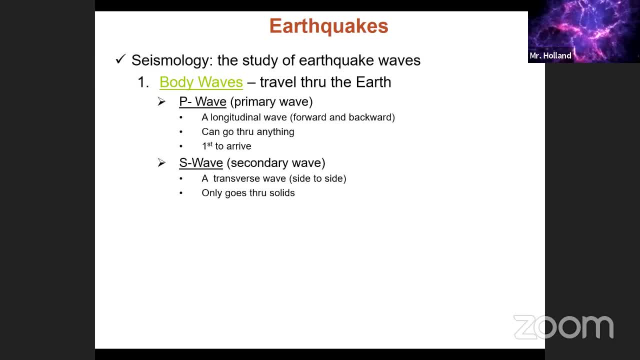 P waves do The S waves don't. That's how we knew that there was liquid in the earth, And by tracking these waves we could tell where that liquid was located. Again, the second wave to arrive is why we call it secondary wave. 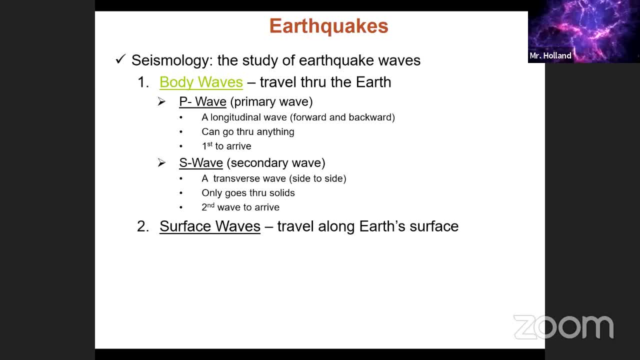 The other type of wave is called the surface wave. A surface wave does just that: Travels only on the surface of the earth. It's kind of an interference of the other waves, S and P, and it manifests itself on the top of the earth. 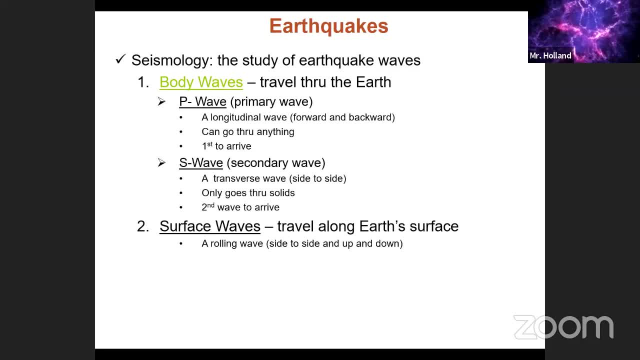 It's a rolling wave. It causes a side to side motion, like the transverse wave, up and down motion and a forwards and backwards motion. It's all of it put together Creates a huge amount of shaking, And this is where the damage comes from: in the buildings. 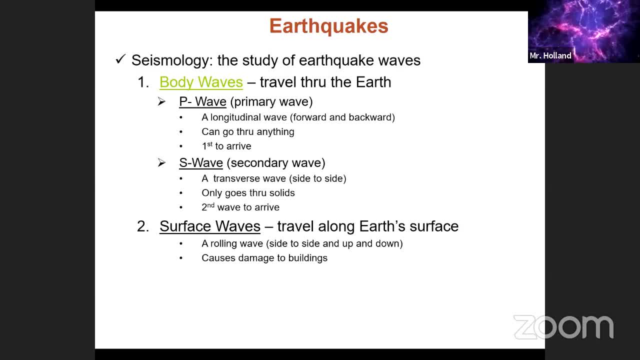 Buildings aren't meant to move in these ways. In California, they designed the structures to withstand a certain amount of shaking, And I forget what the number is. I think it was like 7.0 or 8.0 earthquake, But if it gets bigger than that, buildings are going to start to crumble and come down. 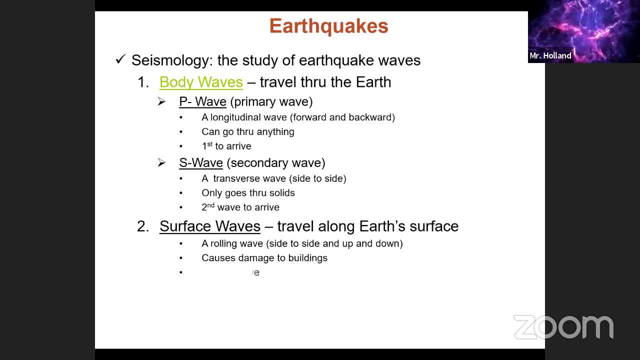 They just can't withstand that movement. These are the slowest waves. They are the last ones to arrive at a distant location. I was out in Palm Springs for two years, which was the desert Mojave Desert of Southern California, And while I was out there they had a couple of big earthquakes. 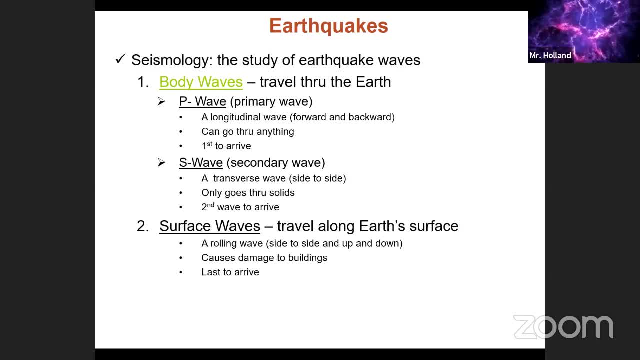 One was the Northridge earthquake back in 1994, I think it was. There was a 6.4 earthquake that happened in Northridge, a suburb of Los Angeles. Palm Springs is about 100 miles away from LA, But when it happened in the middle of the night it caused Palm Springs to shake just like you did in LA. 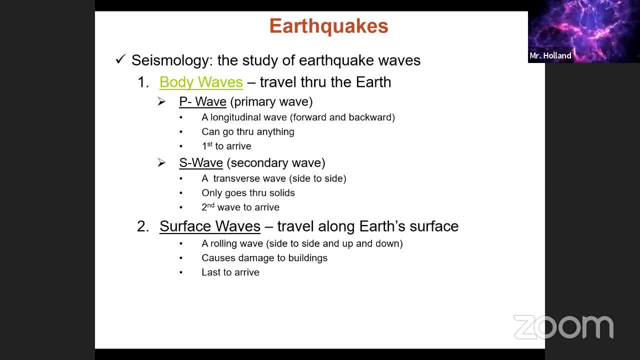 The shaking was just much less. The people described the shaking because some of them are just up at all times of the night Out in the desert. when you see an earthquake coming, it actually looks like a wave of water, like on a beach. 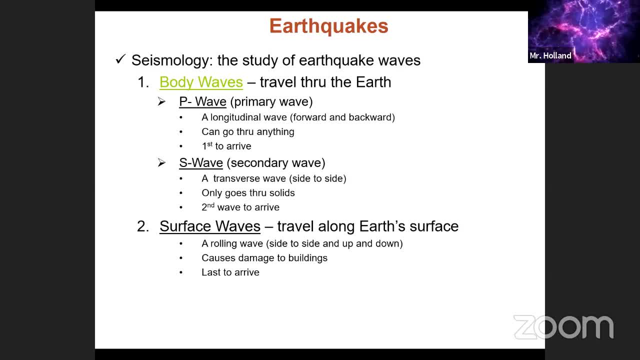 Not the big waves that crash down, but the smaller waves that come in. They described the Northridge one as about a foot-tall wave of sand. So you're looking across there in the moonlight and you see this wave of sand coming at you about a foot tall. 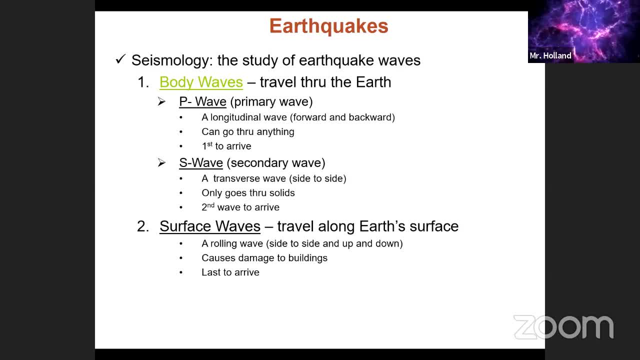 On the backside of the wave is a dust cloud being created because, as the sand is waved up, it picks the dust up And you can see it. You can see the dust coming up into the air. When that wave hits you, it actually makes you raise up one foot into the air. 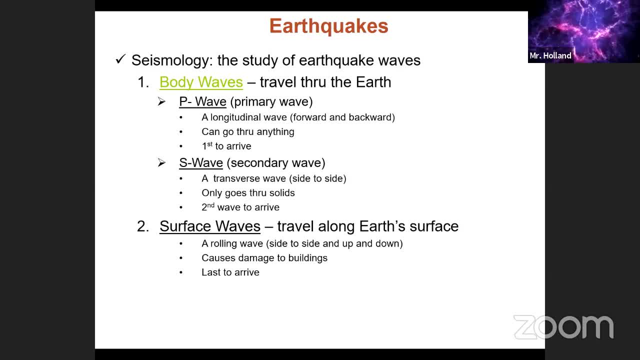 As you're standing on that wave at the top, the crest, and you fall back down to a natural level of the ground, So you feel that as it goes through. At the time I wasn't outside, I was in my apartment. 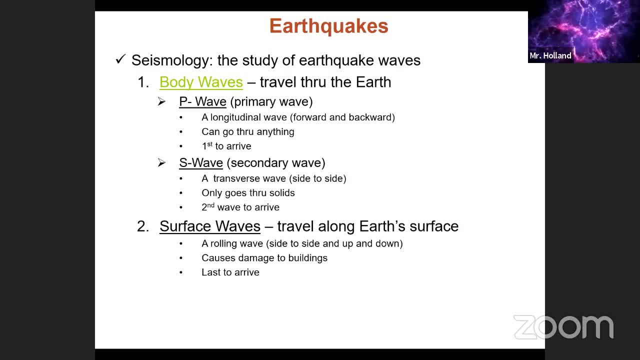 And the apartments don't move nearly as much as the ground does. So the ground moves like that. The apartments move less because they're solid structures. In my apartment, when I was in there, the wave moved me about two to three inches. 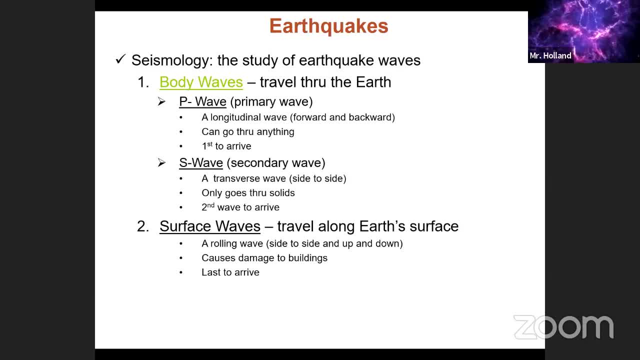 I stood, went up, came down as it went through the building. It's a weird feeling. You know the buildings aren't supposed to move like that, But somehow they build into the structure that withstands a certain amount of that type of movement. 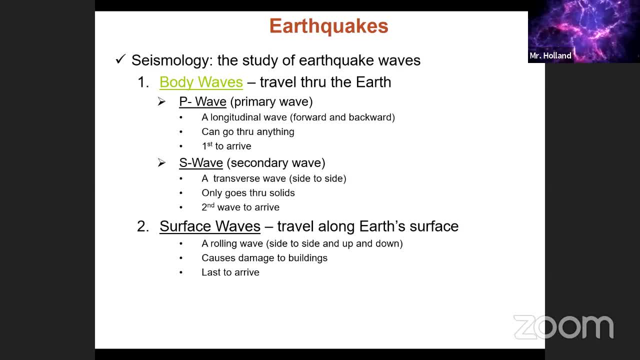 Questions for earthquakes. All right, The size of the ground. this is what one looks like As a wave comes in from a baseline. it begins to shake the needle up and down. The wave begins to decrease after the P wave gets there. 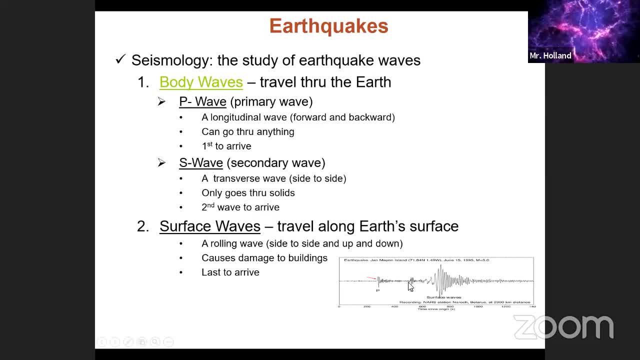 Eventually, depending on where you're at, the S wave comes in And it begins to shake the needle up and down again. Shortly after the S wave comes in, then the surface waves come in And they're the ones that cause the big shaking of the needle. 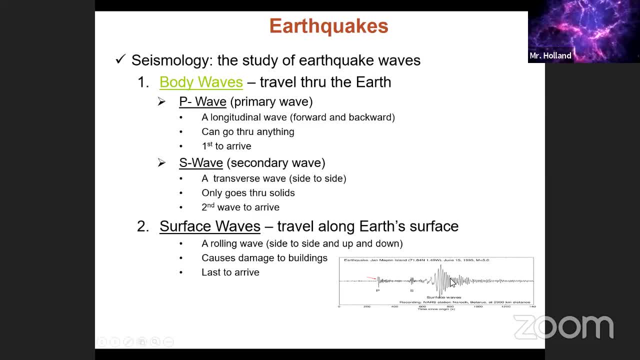 Because they're closest to the ground, where the ground sensors are located. When I was in Palm Springs, at the school I was at, we had an earthquake device sensor that measured when the P wave would hit this rod driven into the ground And it transferred the signal up and rang the bell at the top. 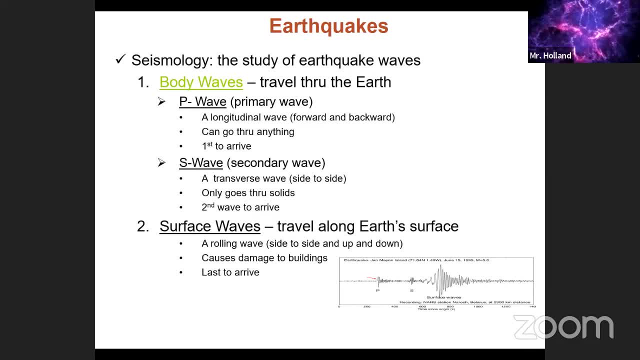 So we would have the alarm kind of like a fire alarm, But it was an earthquake alarm. That way, from the time the P wave got there, the alarm is going off until the surface wave comes in and things start falling apart. We would have time then to theoretically get out of the classroom. 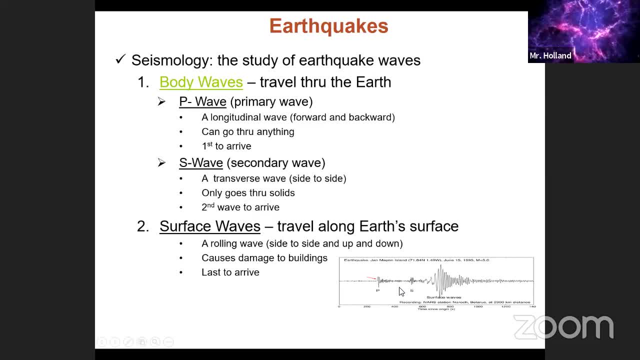 Because in the desert You need time not to get out. When you leave the door of the room, you're outside. It wasn't in the buildings here in the North. It's out there where it's nice and warm. Just escape the classroom to the classroom, to the classroom. 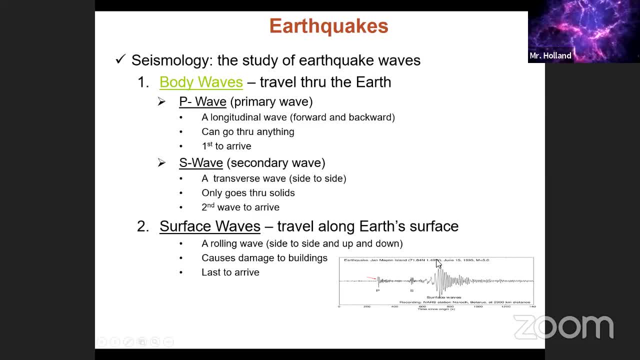 The best place to be would be outside, where nothing is above your head to fall on your head to cause damage and injury. However, if you couldn't get out, the next best place would be to crawl under these tables. They're fairly sturdy structures and as the road falls down it would make the stuff fall off the sides and not right on your head. 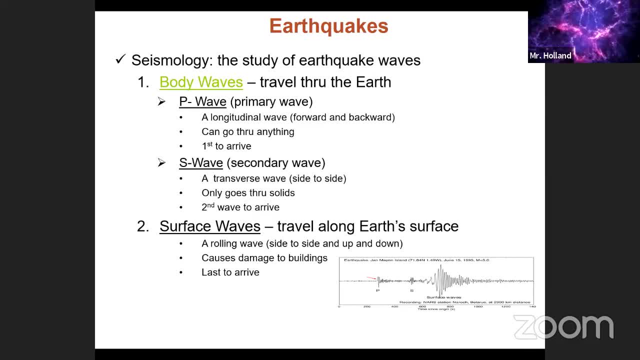 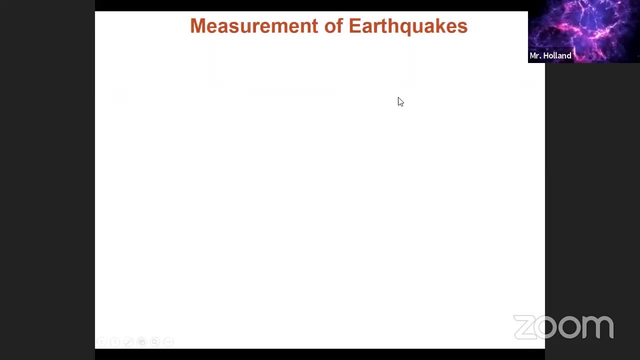 yourself. you go to the table or in the door frames because things fall to the side of the door frames. go ahead and measurement of earthquakes. there are three squares to measure the earthquake. the first one is the moment magnitude scale. this is the one that actually measures the 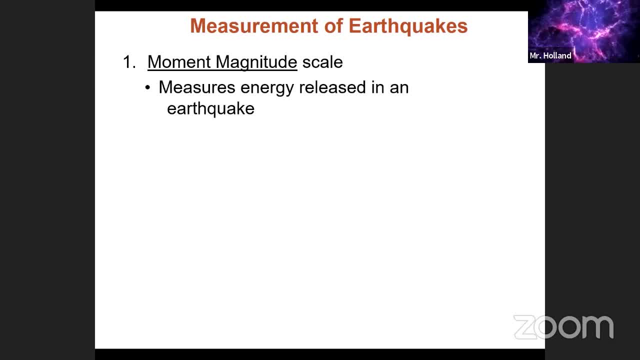 energy released from the earthquake. geologists like this one the most, because they actually go to the earthquake site, the epicenter. they measure the fault line and how much movement literally or physically took place. they put that into a formula, calculation, measuring how deep down the focus was, the type of rock that was there at the time. they always factors that they did. 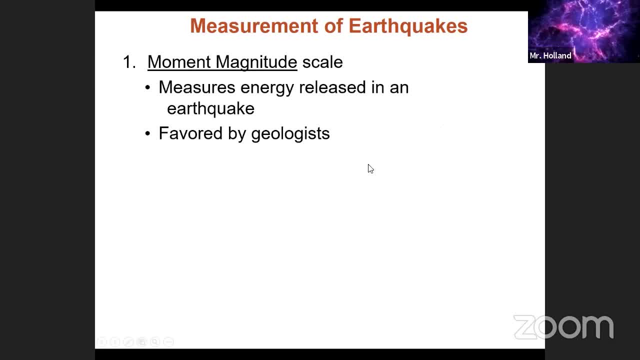 and they could calculate with a pretty good degree of accuracy the amount of energy that was released in that earthquake. that's why geologists like that one. it's more of a numeric measured item. the second one is the Richter scale. the Richter scale was the one that came. 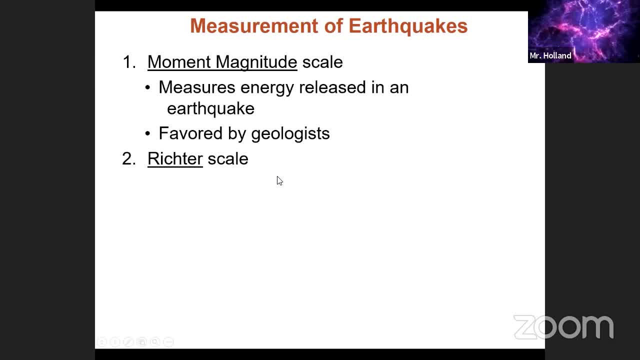 in in the 30s. this one uses the seismograms and measures on the piece of paper the height of the shaking there to figure out the wave intensity. it takes into account the distance away as well, and there's more room for error in the Richter scale. so that's why they steer a little bit clear. 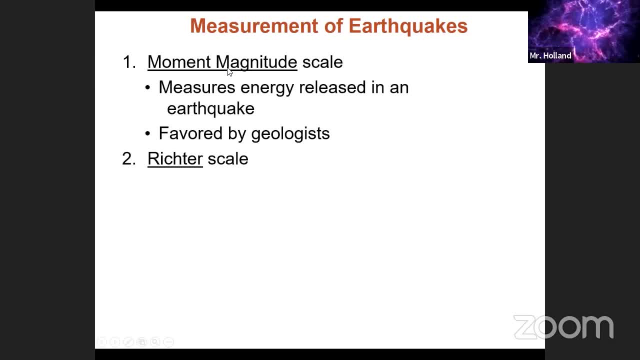 of that if they can. well, the magnitude scale was developed, released in 1979. Richter scale was 1935. and this one again is just making the shaking, measuring the shaking of the ground. that line on the paper media likes this one the best because it's the quickest one to get out to. 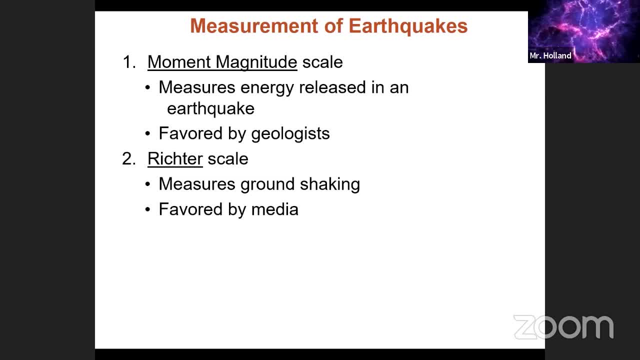 the people. you have that piece of paper instantly. you can measure the line links, the shaking. you put it into a table and it tells you the estimated intensity of that earthquake. the third and final type: this is what was developed by the 1902. it was the Mercalli scale. 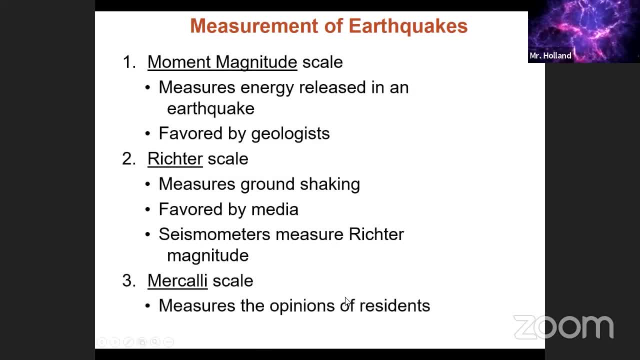 this is the one where they sent postcards to individuals and got their opinions as to what they felt happened during that earthquake. scientists then evaluated the responses and figured out the numeric scale. based on that- any questions about the three scales we have- you guys will be working with the Mercalli scale. 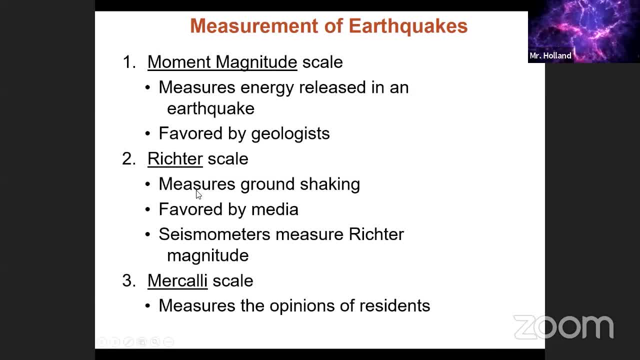 and the Richter scale, which is that tutorial you'll be doing on Thursday. Moment magnitudes we don't do much with, so just be aware that that's the one that the geologists will use. We're going to be working with the other two, All right. next disaster is the tsunami. 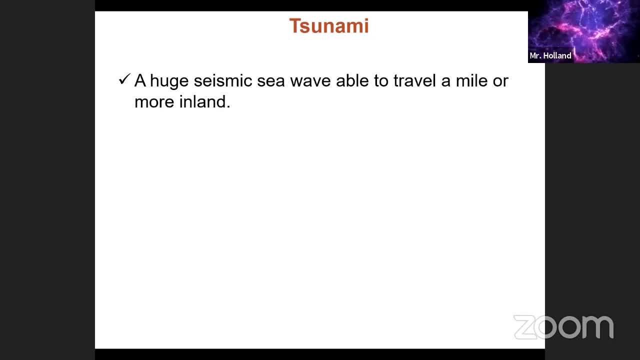 The tsunami is a huge seismic wave that is able to travel up to a mile or a few miles inland. It travels out in the ocean at several hundred miles per hour. There's a video clip that talks about it going to as much as 500 miles per hour, so it's moving at a pretty good rate. 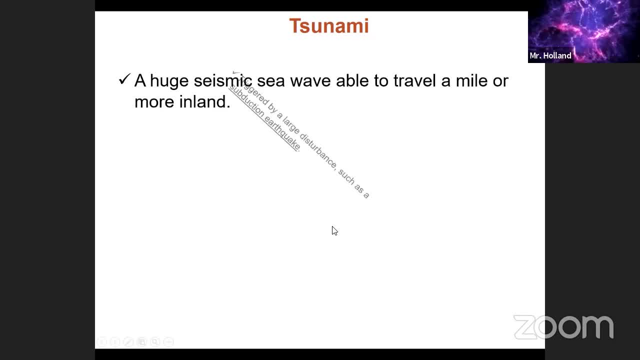 Kind of hard to swim. faster than that, It is triggered by a large disturbance under the water, such as a subduction earthquake, Like in Alaska 1964, we had the Pacific plate being subducted underneath the North American plate. that thrust Subduction that happened there released a huge amount of energy. 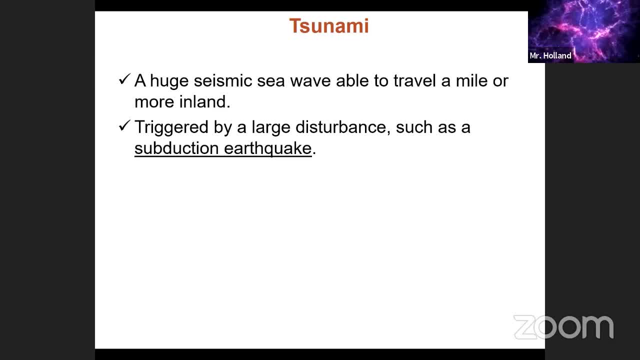 that made an earthquake at 9.2 in magnitude the biggest one ever recorded. It also produced huge tsunami waves. Those underwater disturbances are what caused most tsunamis. This right here was a tsunami that happened in Japan 1911,, no 2011.. 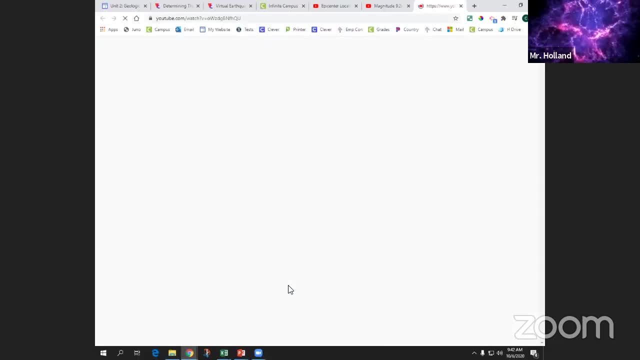 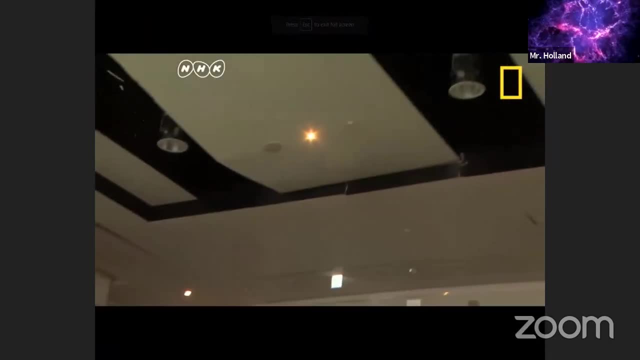 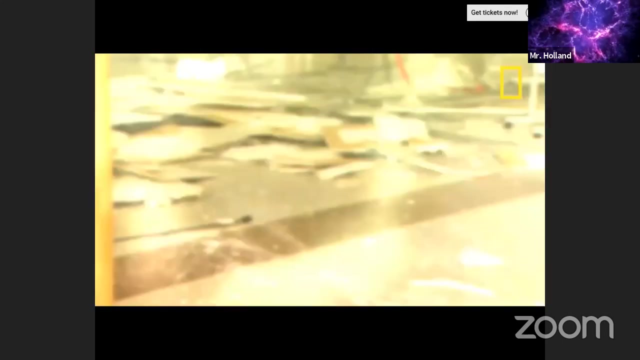 This is years ago. Go ahead and watch a little clip of it All. across northern Japan, they felt it- A violent magnitude 9.0 earthquake on March 11, 2011.. It was centered about 80 miles offshore and tsunami warnings went up immediately. 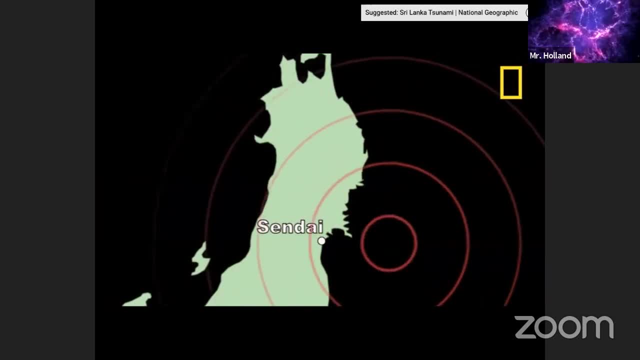 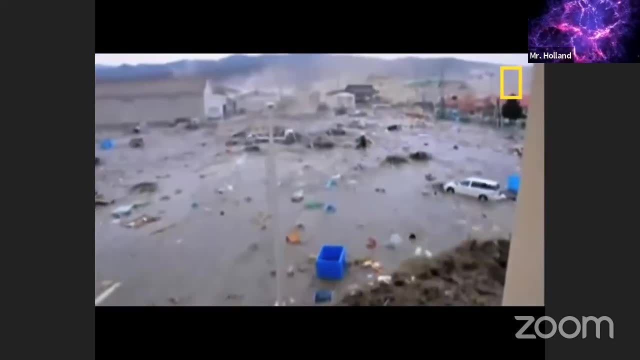 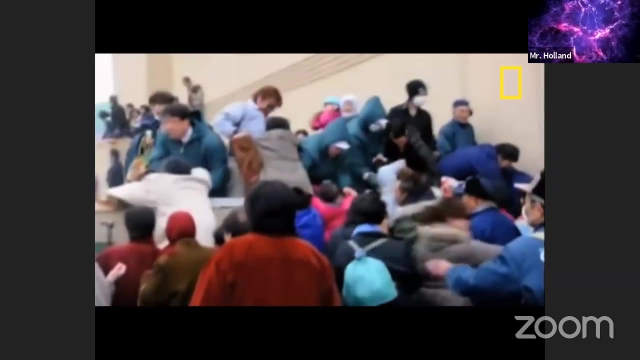 In coastal cities, people knew what to do next: Run to higher ground. It's from these vantage points, on hills and in tall buildings, that incredible footage recounts. In Tecumseh, people recruited your high-rise rooftop and could only watch. in Florida, 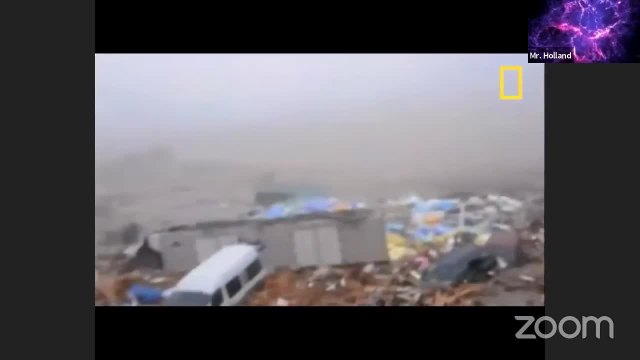 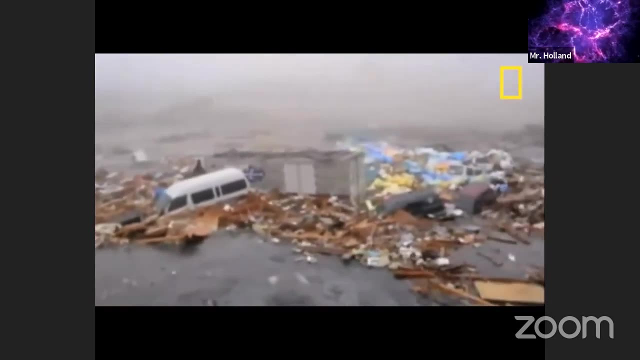 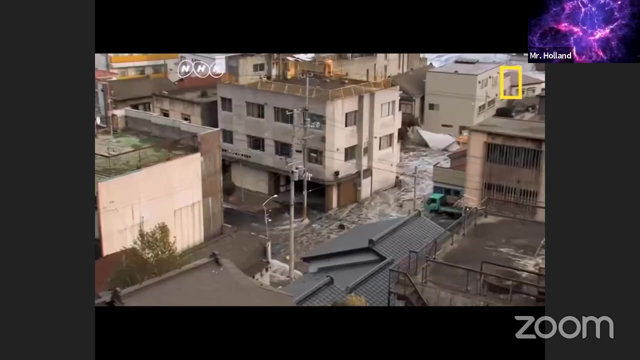 as tsunami waves inundated their city, knocking buildings into rubble and mixing into a kind of tsunami soup filled with vehicles, building parts and concrete, Seawater passed over a sea wall and in the city. This video shows the water rushing over an 18-foot seawall in the Kamaishi City. 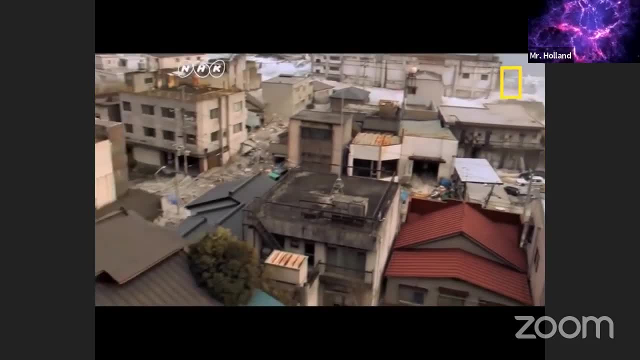 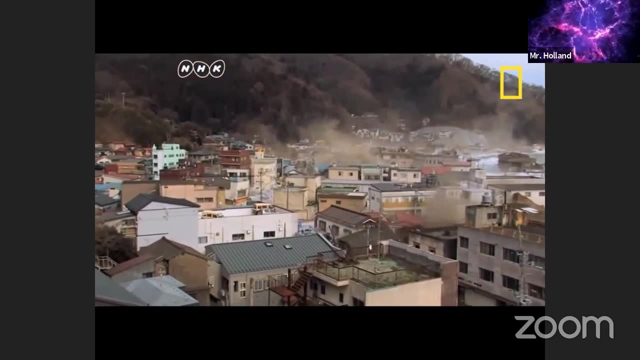 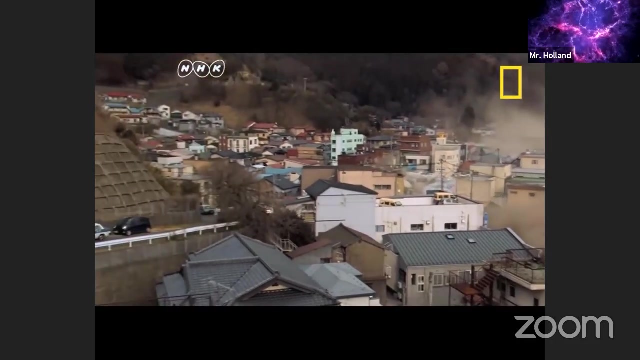 The seawall here was the world's deepest and largest, but not enough for the magnitude of the March 11 disaster. It was the largest place ever known in Japan and one of the five largest reported in the world. More than 28,000 people are confirmed dead or missing. 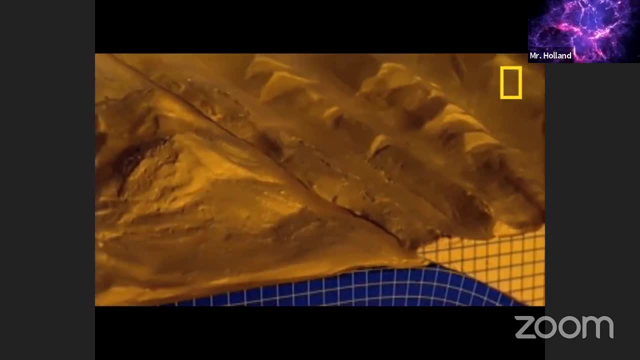 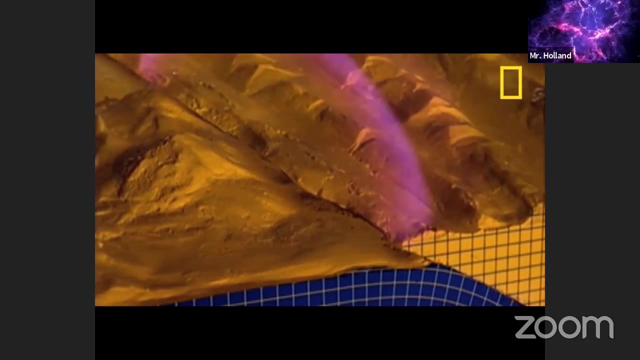 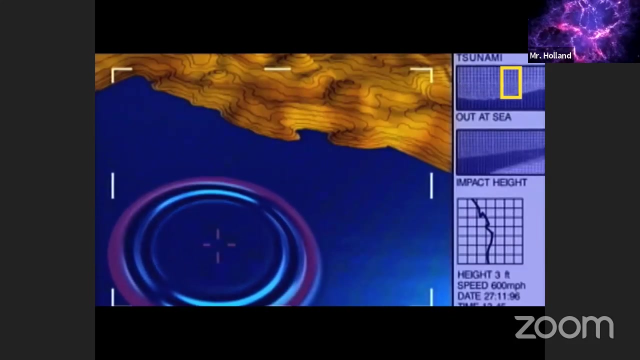 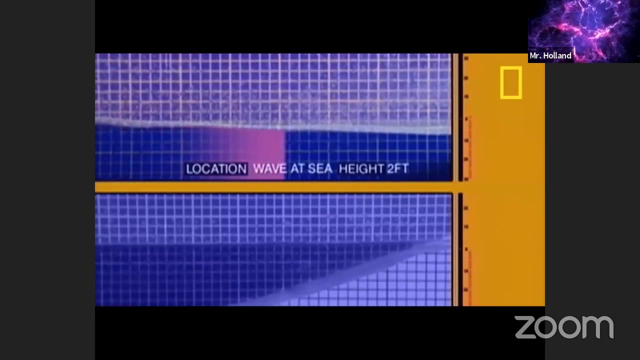 When two tectonic plates split together under the sea, the resulting earthquake sends an enormous burst of energy up through the ocean, displacing enormous quantities of water. With the upward motion, a series of waves expands in all directions. In deep water, these waves travel fast- up to 500 miles an hour- but only reach a height of a few feet. 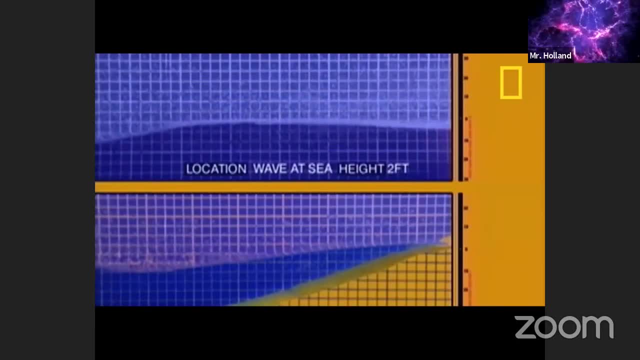 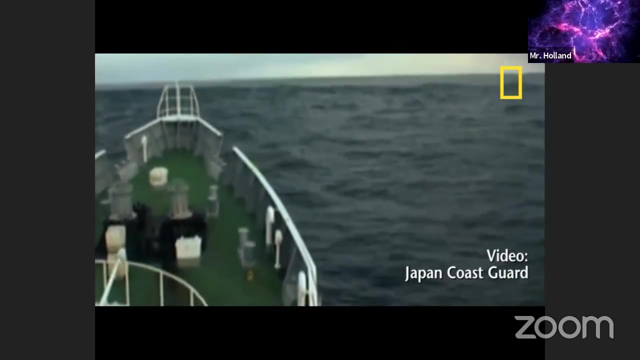 A passing ship might not even notice, But as the waves enter shallow water swiftly, the ocean floor lowers the waves' speed but loses their height. This video is from a Japan Coast Guard ship confronting a tsunami wave in shallow water on March 11.. 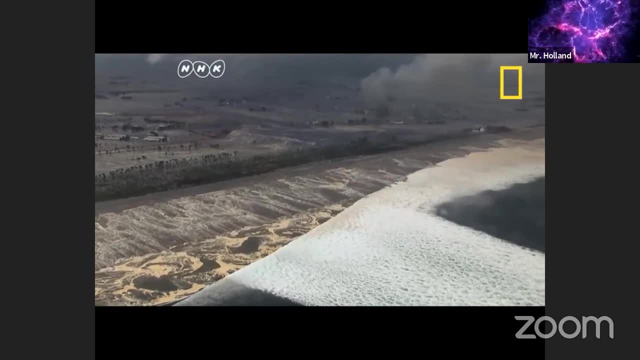 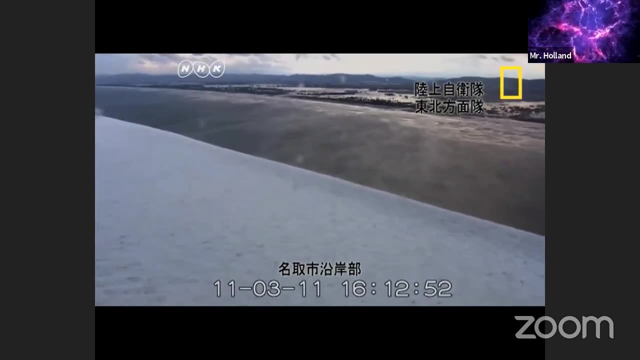 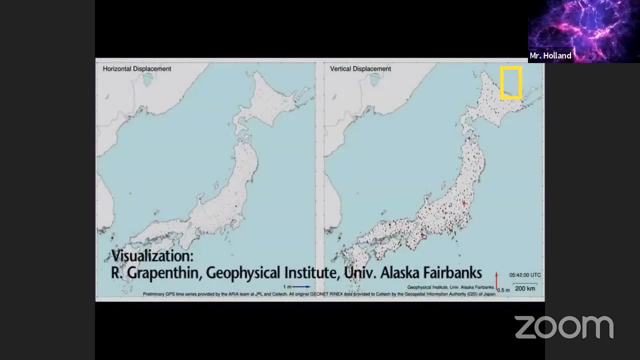 And a rare view from the air Video of a tsunami wave approaching the foyer In Japan. some tsunami waves reach as far as 3 miles in the ocean. Japan may be the most seismologically studied country in the world and, with more than 1,200 high-precision GPS stations, 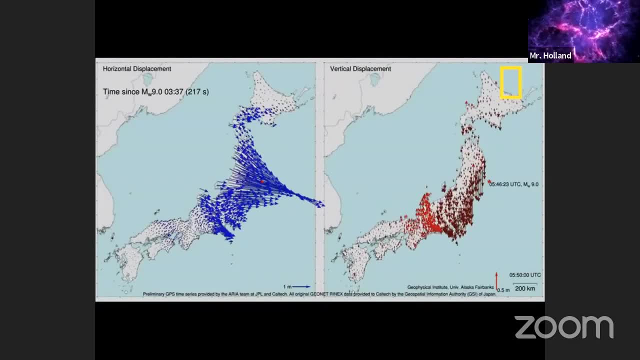 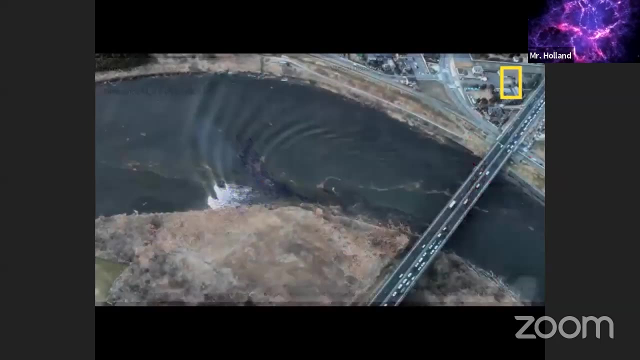 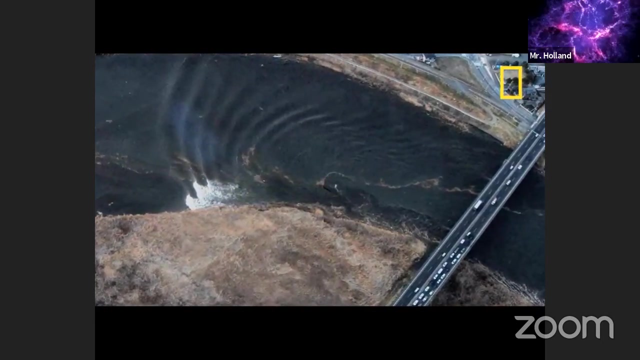 a geophysicist at the University of Alaska, used the data to create a visualization of the March 11 disaster. The waves of displacement that you see were moving as fast as 5 miles per second. In this photo, the ripples of tsunami waves are seen moving upstream in the Manaka River at Kitakyumaka City. 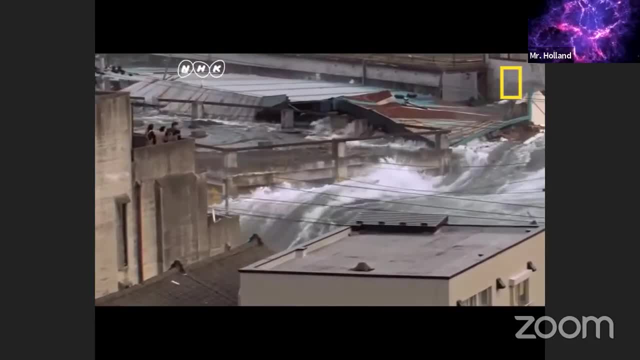 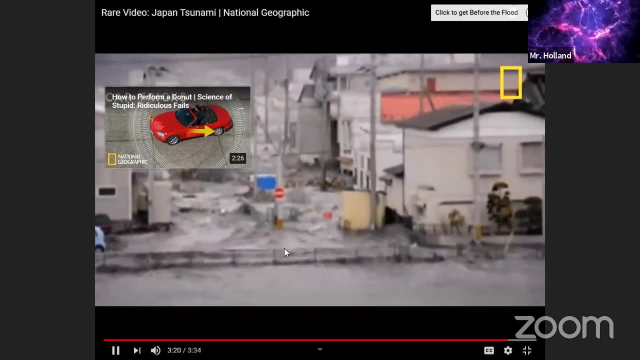 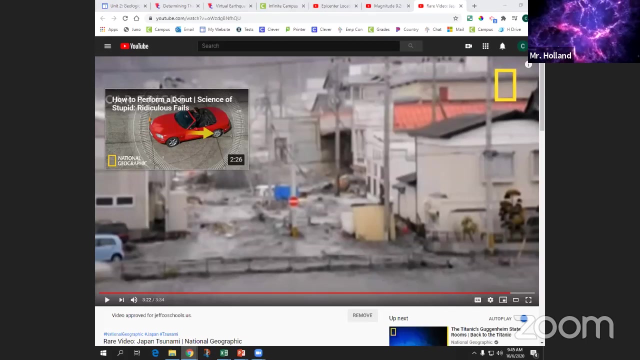 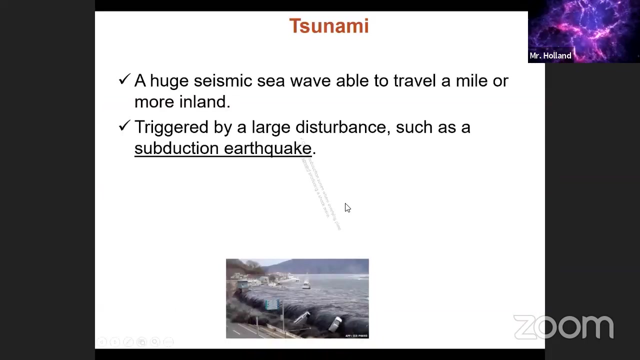 New technology left an enormous amount of visual evidence for study in years to come and can perhaps help us better understand the power of earthquakes and tsunamis and prevent what they're doing. The subduction zone area that causes a tsunami happens because of the springing upward effect. 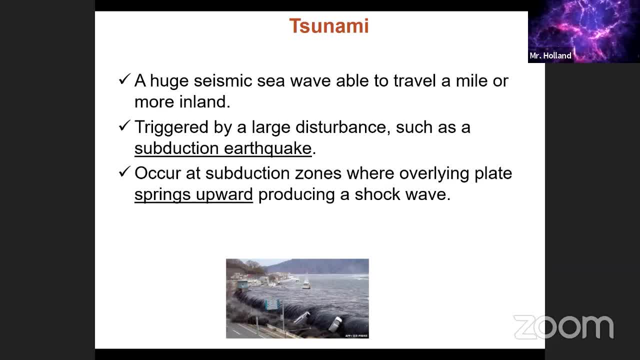 You have the continental place that's going up, You have the oceanic crust that's going down. When they jump past each other, it creates an up-down movement, which is that side-to-side wave, that transverse wave, that initiates that tsunami. 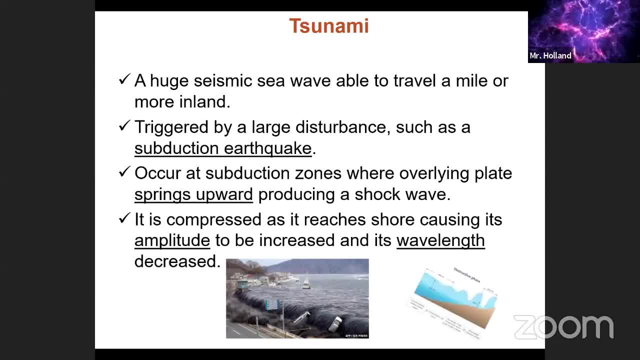 It is compressed as it reaches shore, causing its amplitude to be increased. That's its height. As the wave slows down because of the friction with the ground, it gets taller and taller and taller, and the wavelength from crest to crest gets shorter and shorter and shorter. 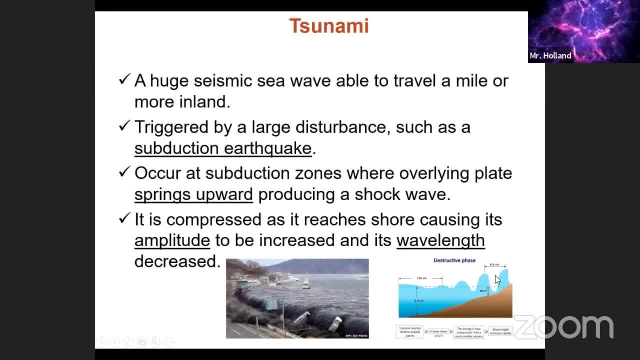 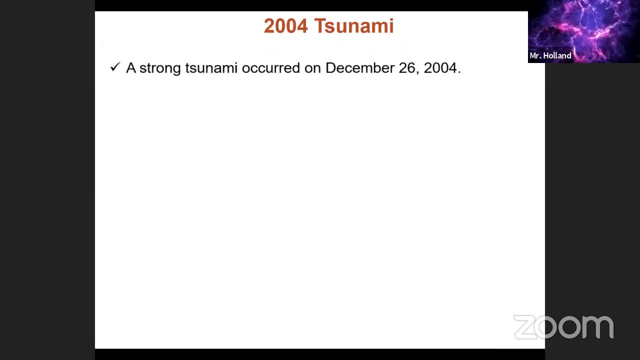 They get closer together. So the waves get closer together and higher, up until they finally reach on land and flood the land. Questions about that tsunami effect. The most devastating tsunami happened in 2004.. December 26, 2004,. that's Boxing Day for that part of the world, in Indonesia. 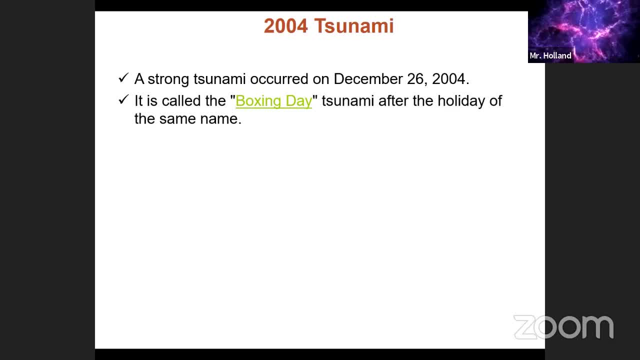 So they named this the Boxing Day Tsunami. the day after Christmas, It was generated by a 9.1 subduction zone earthquake off the coast of Sumatra. Again, Alaska was a 9.2. This was really close to that 9.1.. 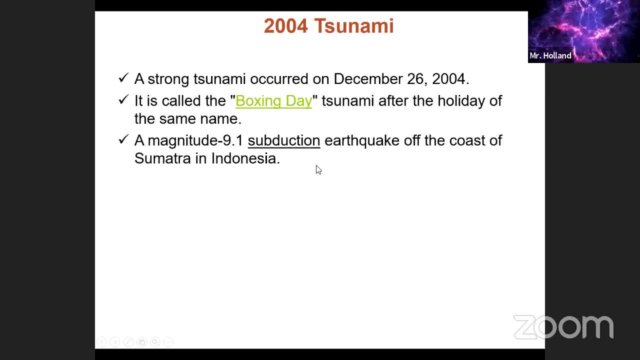 This one being a little bit different, because it was a much more populated area. People living on the islands there, low-lying areas so much more impacted by flooding. It released more energy in that earthquake than all the bomb blasts of World War II combined. 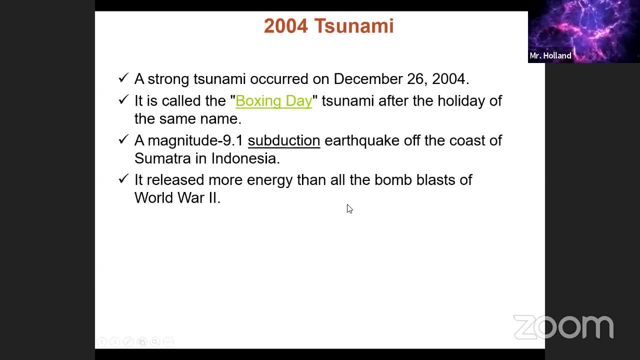 Huge amount of energy released in a 9-point earthquake And it caused a tsunami And it caused 2,075 deaths. It was the deadliest tsunami ever. We hear about places like New York City that was having quite a few deaths in a day. 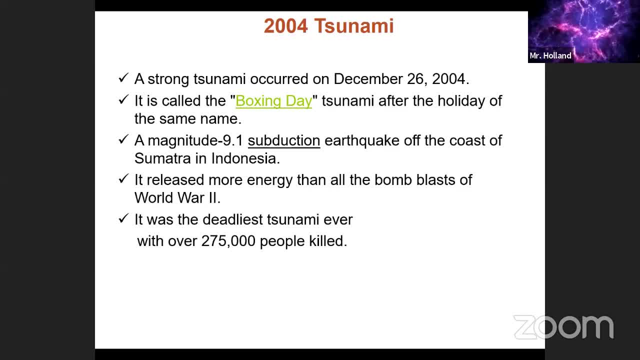 And the bodies of tens of people were building up because they used to have morgue space to put them. So they brought in refrigerated trucks And they put the bodies this summer in refrigerated trucks so that they would preserve them and they wouldn't start to rot. 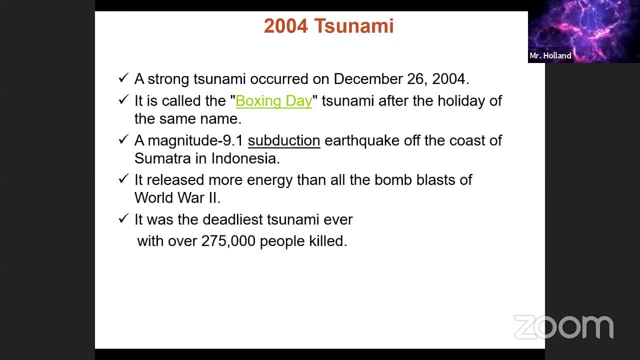 In this area 275,000 people. they had no place to put anywhere near those bodies, So what they had to do was stack the bodies along the roadways, the beaches, anywhere they could find Several bodies high. 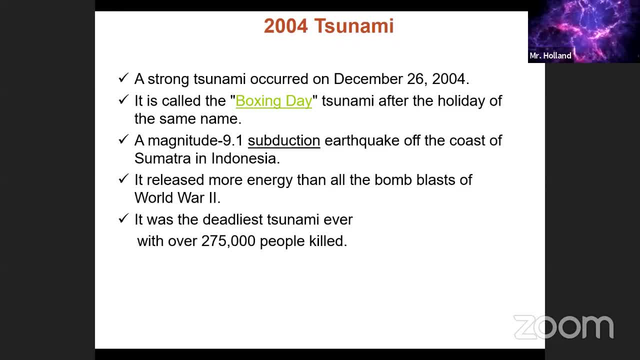 And they just left them out there for weeks and weeks until they could finally process all of those people that died. People that were there described the smell as being unbearable. The rotting flesh itself led to all kinds of different diseases And caused many other problems to go along with the damage from the flooding itself. 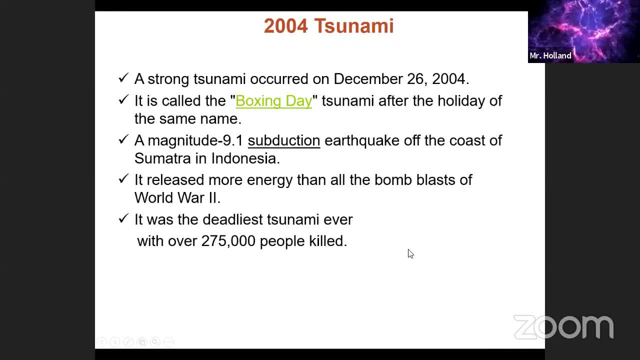 But it was by far the biggest event And at the time it was fairly significant and all over the news for quite a while. This tsunami right here was studied quite a bit. There were a lot of documentaries put together. There's one four-part series or mini-series out there about this one that walks through step-by-step of what it did and how it worked. 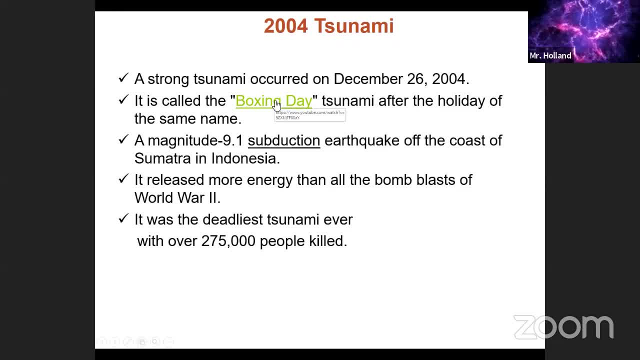 If you're interested in it. it's a pretty good series. This Boxing Day link right here coming up- There it is. There's about a 10-minute clip of that series that puts a lot of information together. It's a pretty good clip to watch if you're interested in it. 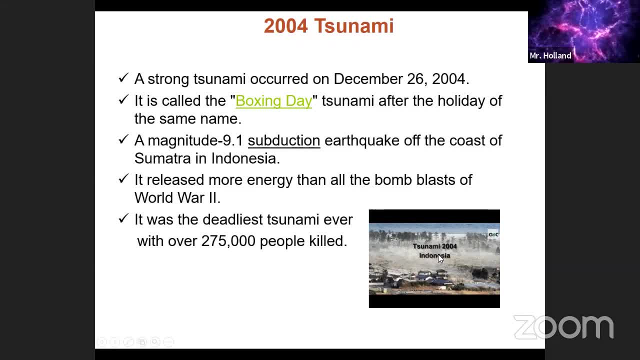 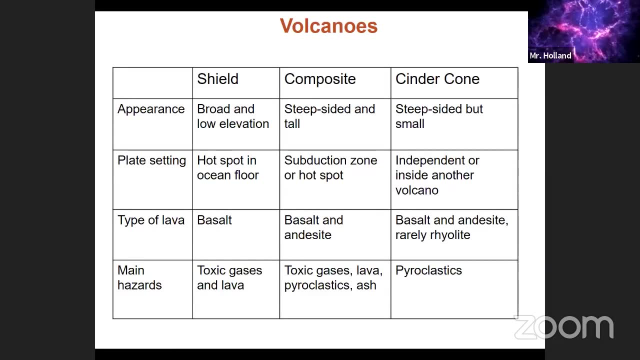 It shows the tsunami wave right here coming up over the coastal region where those trees are right there It's the height of the trees along the beach as the wave moves inland. All right, volcanoes, Number three in our natural disasters. You need to be aware of the three different types of volcanoes. 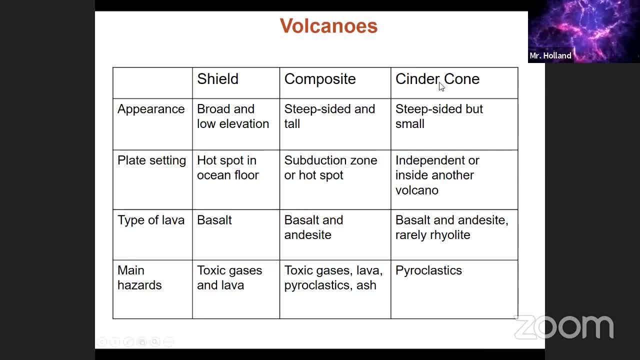 We have a shield volcano, a composite volcano and a cinder cone volcano. The look of them is the easiest way to distinguish one from the other. A shield volcano is very wide and broad compared to a low elevation. Elevations are around 4,000 feet at their highest point. 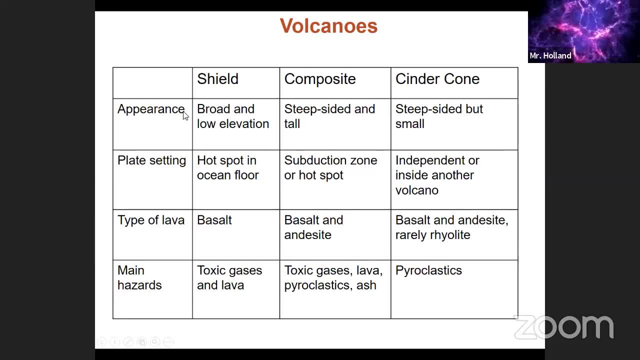 But they are many, many, many miles across. A composite volcano has a very high elevation. A composite volcano has fairly steep sides And it's fairly tall. We're talking 10,, 11,, 12,000 feet of elevation. 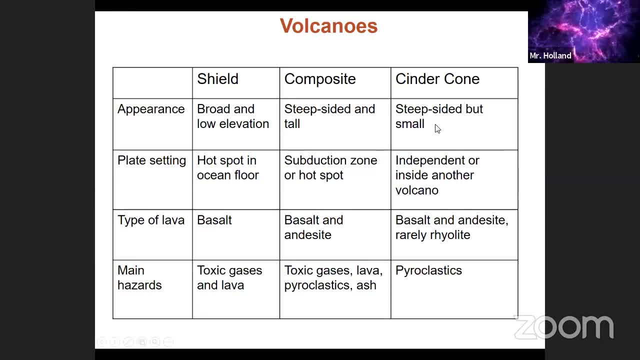 And then finally, the cinder cone. These are the baby volcanoes. They have steep sides, just like the composite cone, But they're much smaller, only about 1,000 feet at its highest point. usually The setting, and when they occur, controls the type of volcano. 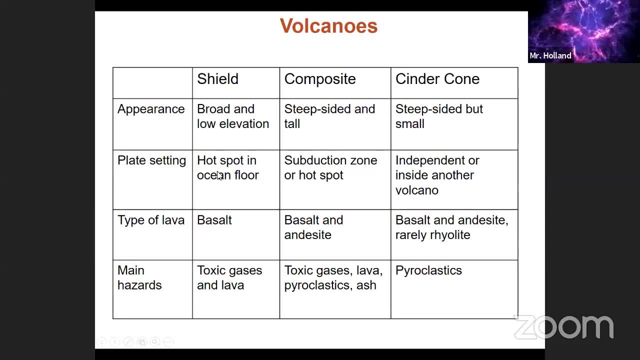 Shield volcanoes form over hot spots in the ocean floor. Hawaii is an example of shield volcanoes And that's how they form. Composite cone volcanoes can form there as well, or also in subduction zones Along our west coast, Washington, Oregon area. that volcanic activity up there with Mount St Helens, Shasta Rainier, all those volcanic mountains up there, happen because of subduction zones. 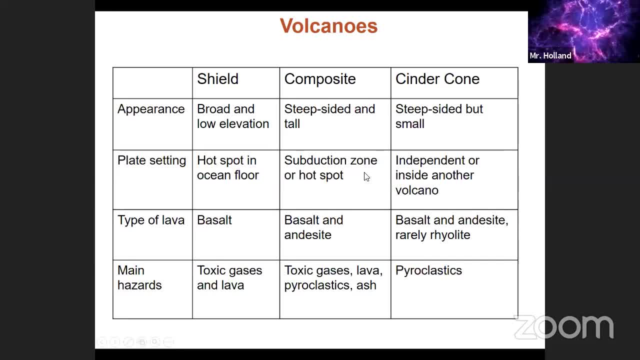 You have the Juan de Fuca Plate, which is a little itty bitty plate, broken off of the Pacific Plate, Subducting under the North Sea, Subducting under the North American Plate, Creating that seismic activity and releasing the magma up into the volcano. 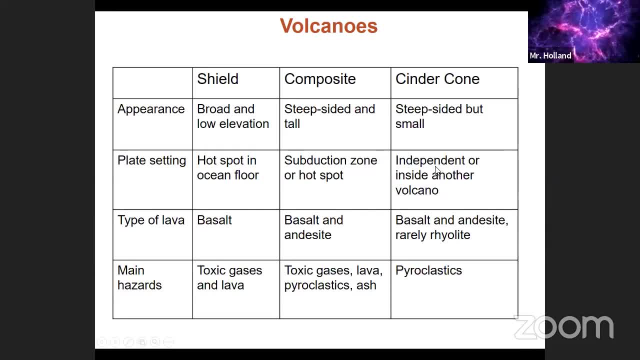 Finally, the cinder cones. They can happen basically anywhere there's a weakening in the crust and you have a magma chamber down below. They can grow off the side of volcanoes, in the middle of a volcano or completely separate from a volcano. The way they explode is controlled by their lava type. Shield volcanoes are made up of basaltic lava. They make basaltic rock. They're oceanic crust. Basalts are very, very thin magmas. They don't hold gases very well. 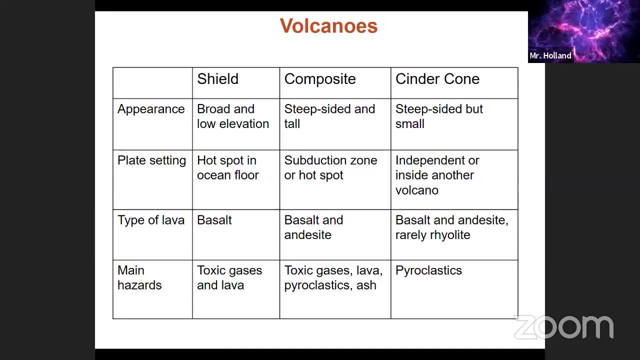 So as gases bubble up in the magma, they just come right out into the air. They don't and aren't held in the magma, So they're a very kind of mild eruption. If we have a composite cone, this is a mixture of some basalt and andesitic lavas. These are thicker. The thicker the lava is, the more it works as a lid holding the gases in The gases held in there until they explode. And when they explode they take the magma with it up into the air, creating the pyroplastic flows and explosions. 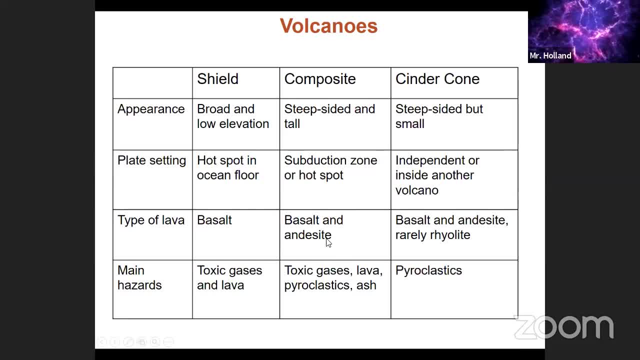 Pyro, meaning fire, Plastic meaning particles and pieces. If we get to the cinder cones, these have the thickest of magmas: Basalt, andesite and some rhyolite in there. Andesite is the thickest of rock magmas. 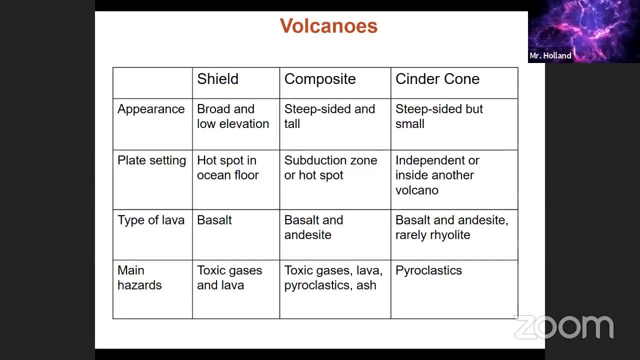 This holds the most amount of gas or the most explosive, but they're fairly small. They shoot up in the air and the fragments of pumice and scoria just fall right back down on the mountainside that's being created as the volcano grows bigger and bigger. 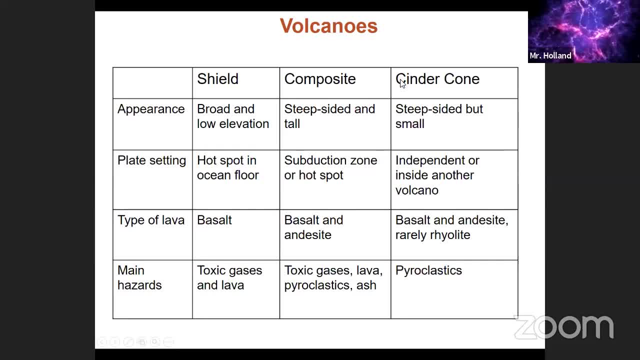 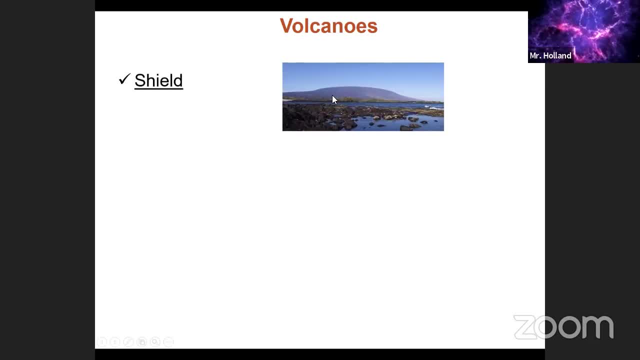 Questions about Enos III. at this time, The easiest way to remember him is by seeing pictures. A shield volcano kind of looks like this. This is a Hawaiian volcano. I think this one's Kilauea Side view shows how wide it is compared to how tall it is. 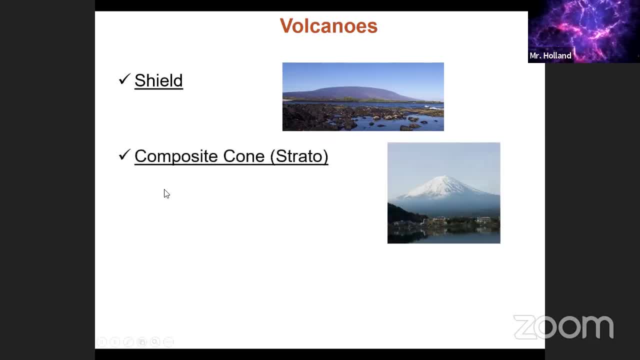 Much wider than it is tall, As opposed to a composite cone, also referred to as a stratovolcano. They tend to have steeper sides compared to their width, Much taller in stature, so much taller that the tops oftentimes go up so far where they're cold and they're snow-covered and icy. 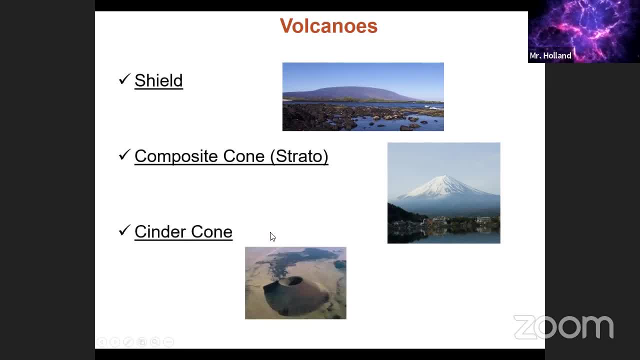 The last one, the cinder cones. These are the baby volcanoes. They pop up, just happen to be wherever there happens to be magma chambers. They shoot the magma up into the air. The lava falls back down as pumice and scoria and creates these really loose-packed sides of the volcano. 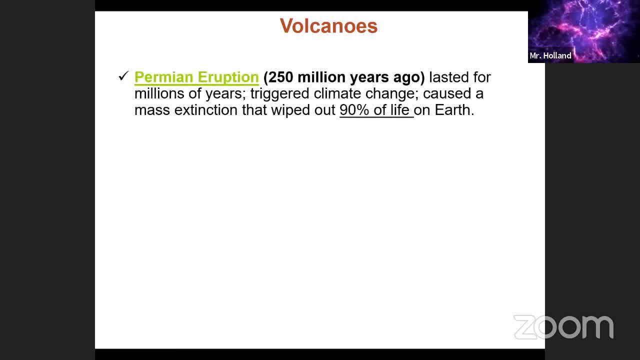 Three big eruptions you should be aware of. The first one goes back a long time. This one is significant because 250 million years ago, it is credited with causing a climate change event that killed off over 90% of all life on Earth. 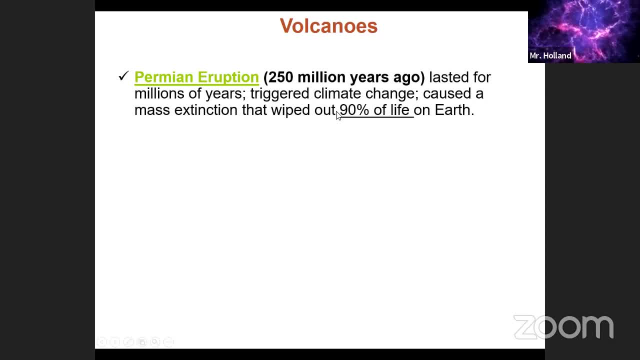 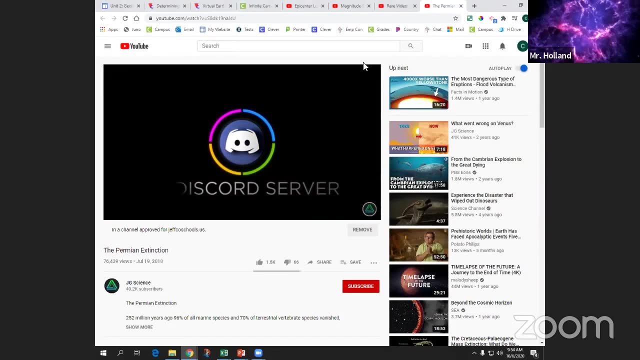 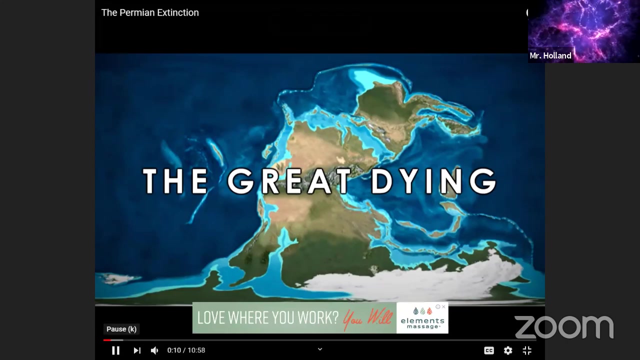 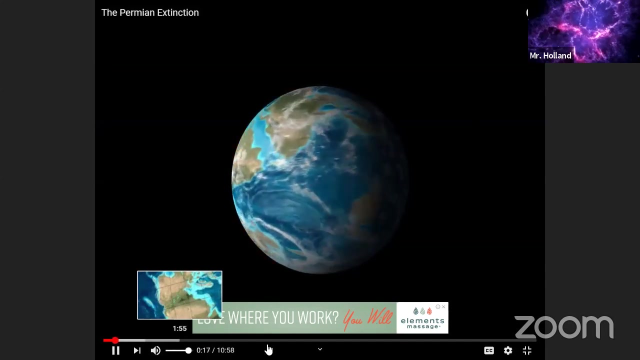 Life was killed off, wiped out And then, hundreds of thousands of years later, many more different life forms took its place. Go ahead and watch a brief video clip of the Permian eruption- This portion of it. About 250 million years ago, here on Earth, something went horribly wrong. 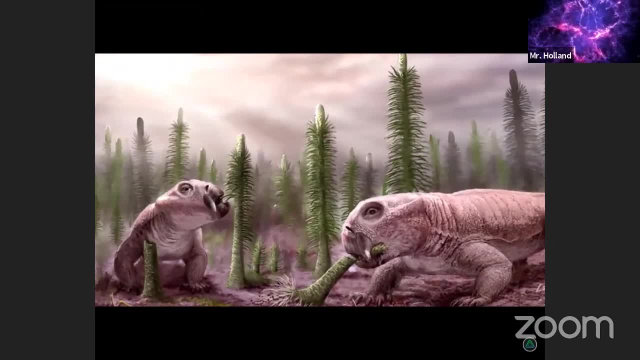 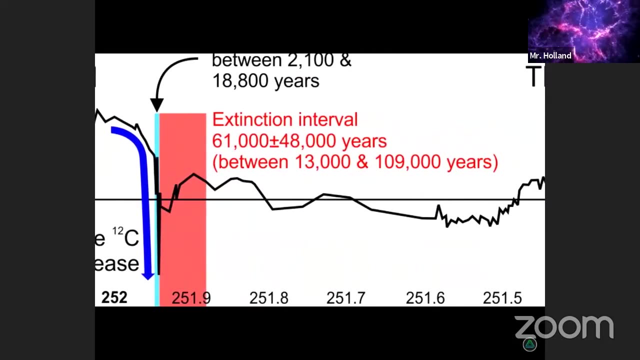 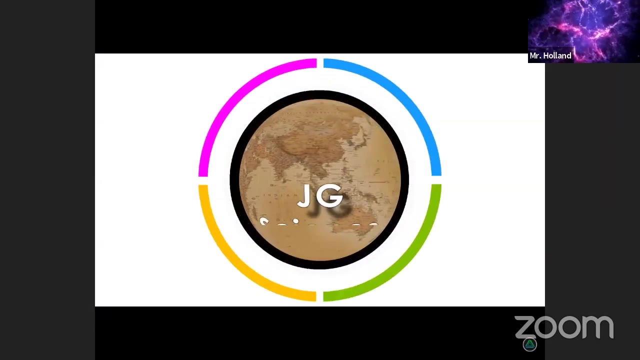 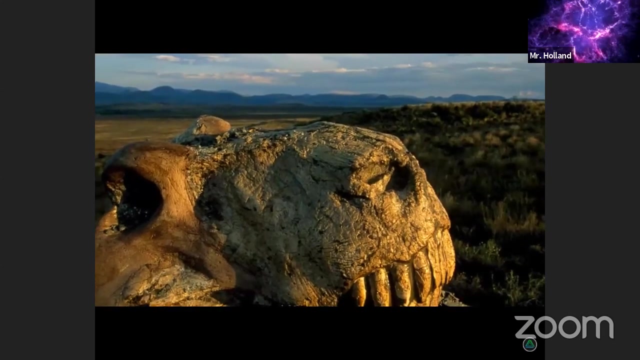 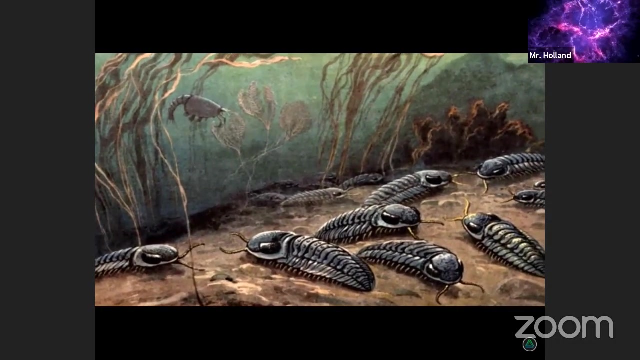 After life had been developing to new heights throughout most of the Paleozoic era, 250 million years ago, up to 96% of all marine species and 70% of all terrestrial vertebrate species died. The reason as to how 57% of all biological families and 83% of all genera became extinct is something we still aren't too sure about today. 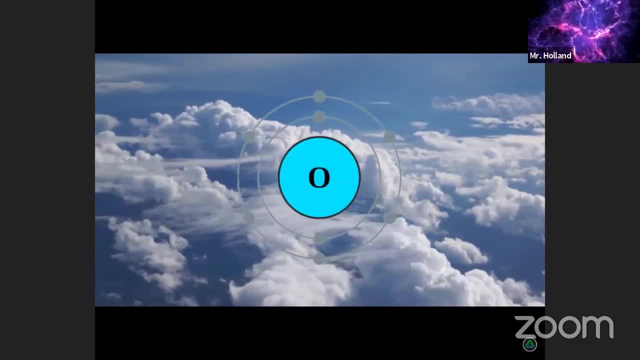 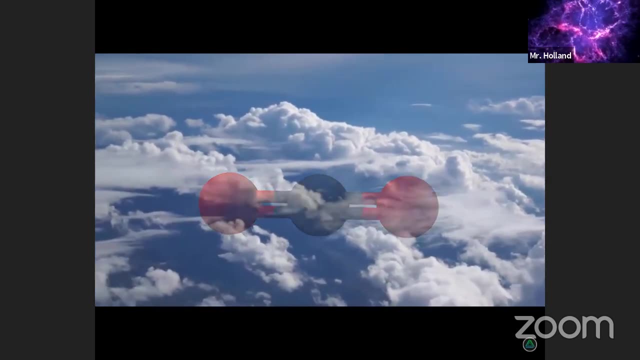 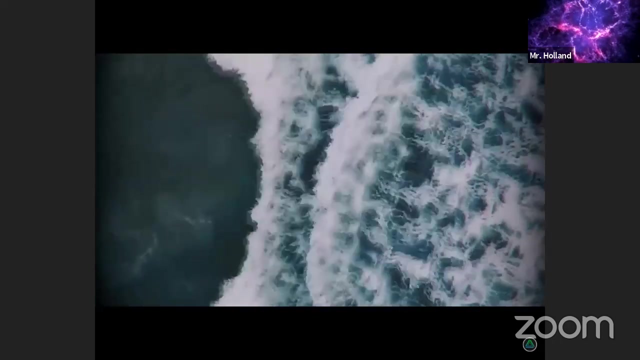 At the start of the Permian period, the Earth's atmosphere was rich in oxygen at 23%, while carbon dioxide levels were around 900 bar per million, about over two times the current levels. The average surface temperature was about 16 degrees and sea levels were at 60 meters below their present. 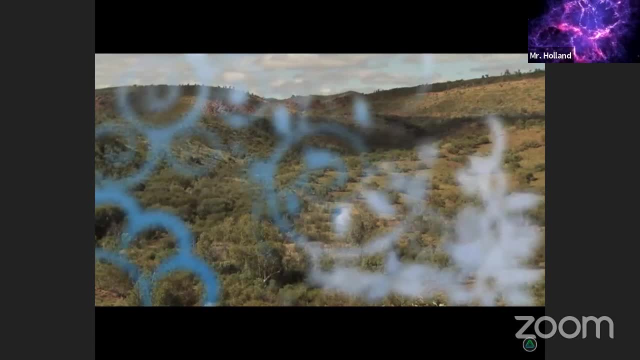 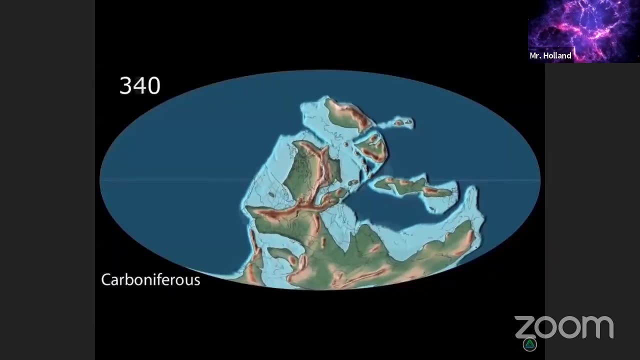 The climate in the Permian period was quite varied. At the start of the Permian period, the Earth was still on an ice age, which began earlier in the Carboniferous period. The most prominent and noticeable change the Permian brought was the formation of a new supercontinent, Pangea. 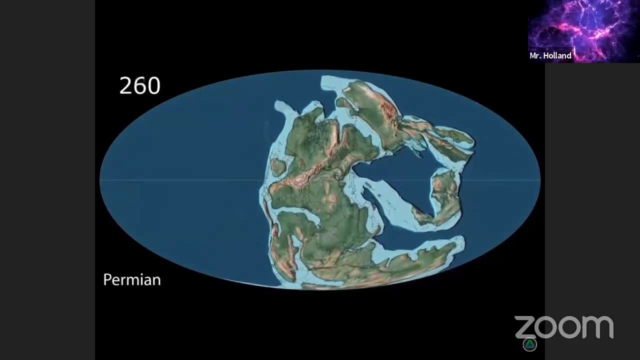 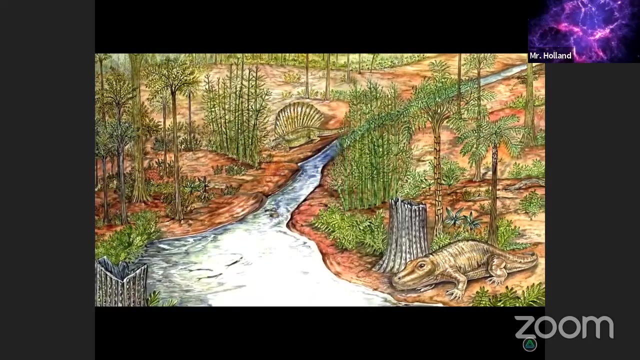 Glaciers were seated around the mid-Permian as the climate gradually warmed Due to the formation of the supercontinent Pangea. this was the main change during the Permian. The formation of a supercontinent created vast amounts of desert land on Earth. as the rain clouds weren't able to reach that far inland and soon the land dried. In a few thousand years Pangea dried out and a vast desert, larger than any ever seen on Earth, would form. To be specific, on Pangea, there formed two deserts as Lombwana and Laurasia merged together in the early Permian. 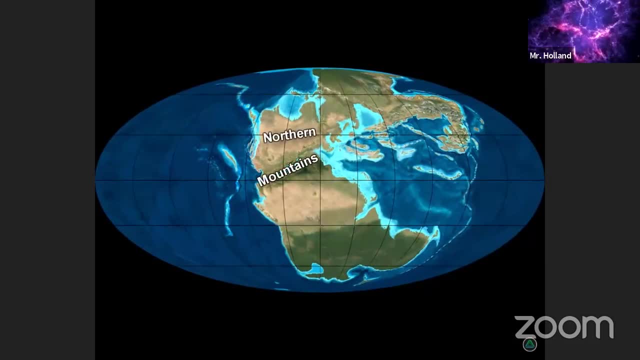 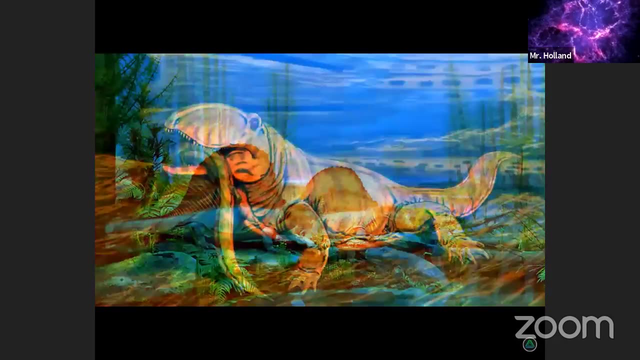 a mountain range formed between them, separating a northern and a southern desert. The Permian saw the completion of a saga that had been going on since the Carboniferous: the rise of the Reptiles. Reptiles like Demetrodons dominated the early Permian. 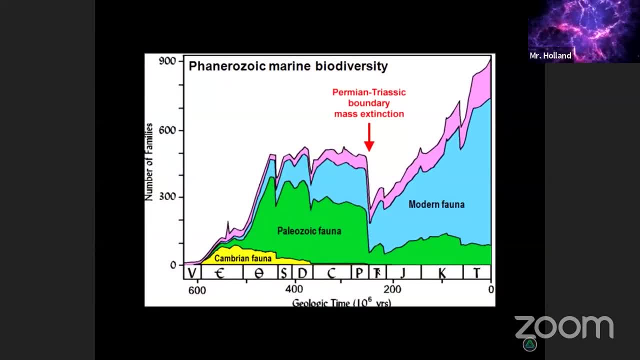 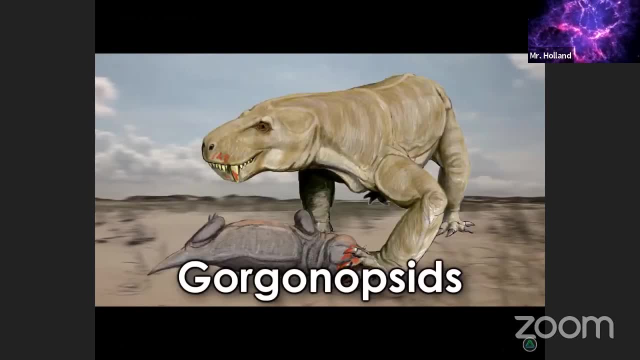 While they diverged more towards the end of the Permian. the new dry desert environment was perfect for Reptiles to thrive in. Scutosaurs, Decynodons, Carbonoxids and others thrived there. Despite harsh conditions, life remained doing well. 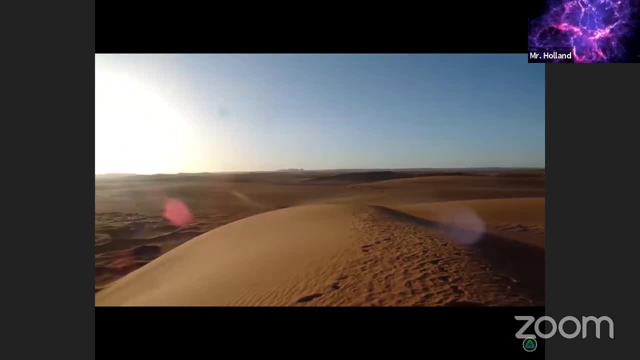 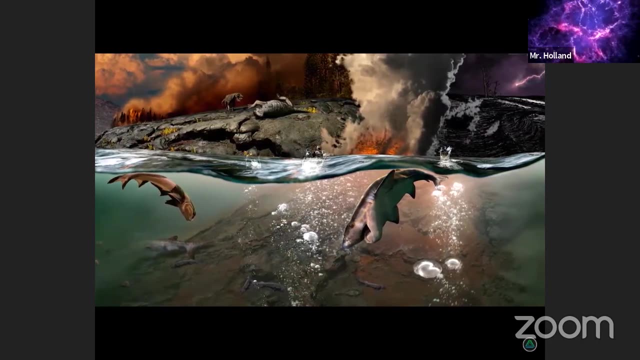 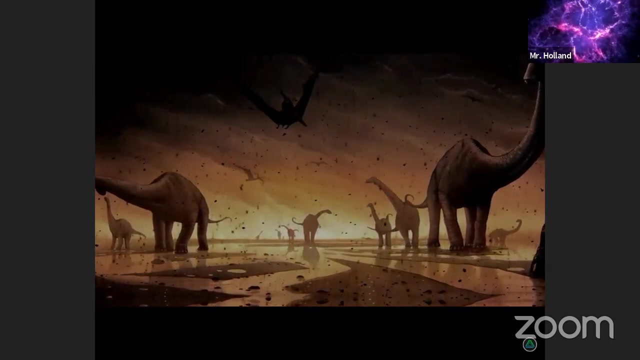 Then, 252 million years ago, on the end of the Permian and start of the Triassic period, all of this collapsed in the greatest mass extinction life on Earth has ever seen. Unlike the meteor that wiped out the dinosaurs 66 million years ago, the cause for the Permian extinction was less clear. 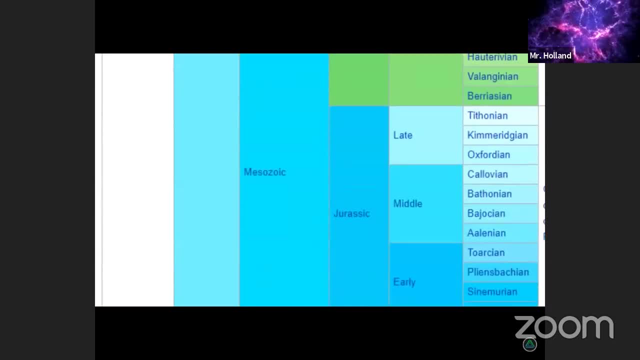 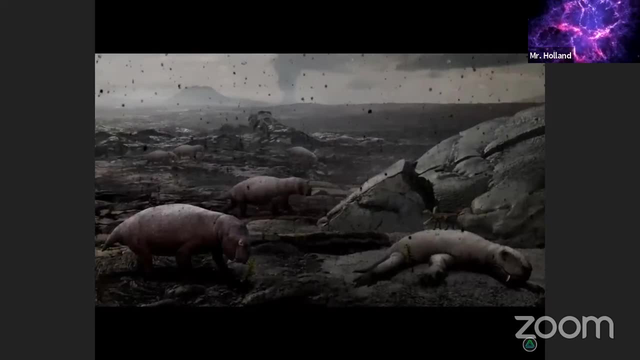 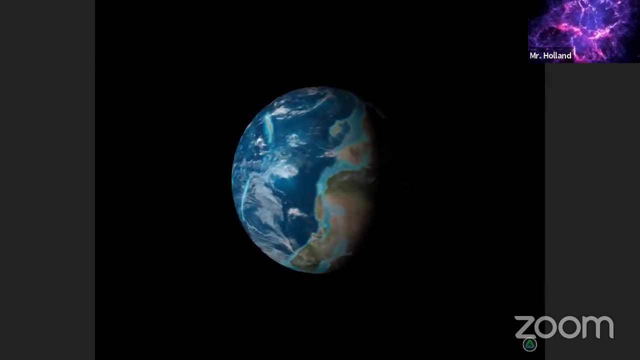 Not only because it happened far longer ago, but also because, in all likelihood, there wasn't a single cause. The Permian extinction likely started with one Kickstarter event that put into motion a tragic sequence leading to the Great Dying. The sequence had its trigger- a puzzled scientist- ever since the first evidence for the event was first discovered. 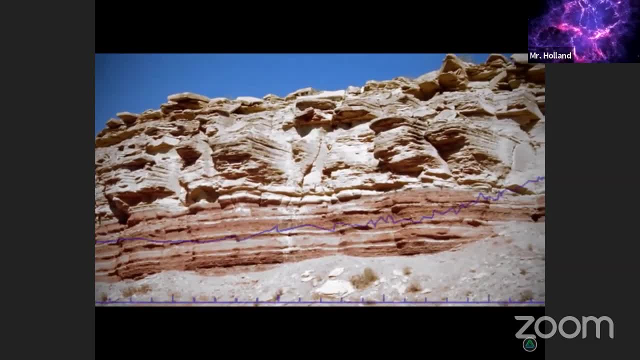 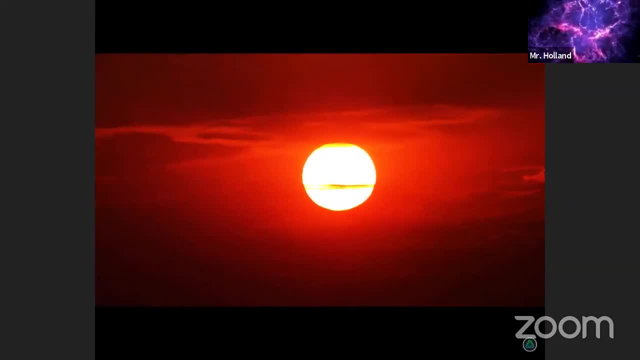 One of the first clues we got was from Cementary Rocks pointed to a rapid increase in the Earth's temperature. at the end of the Permian The temperatures might have risen by as much as 11 degrees centigrade in a short amount of time. 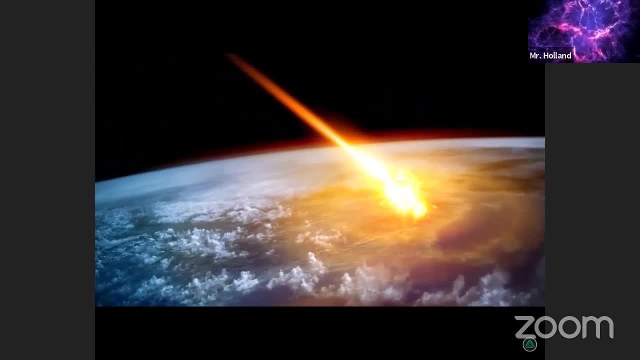 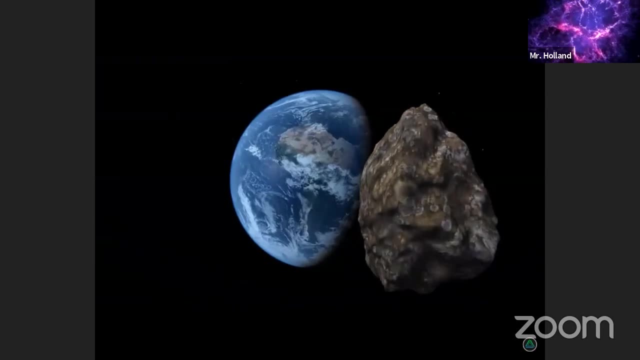 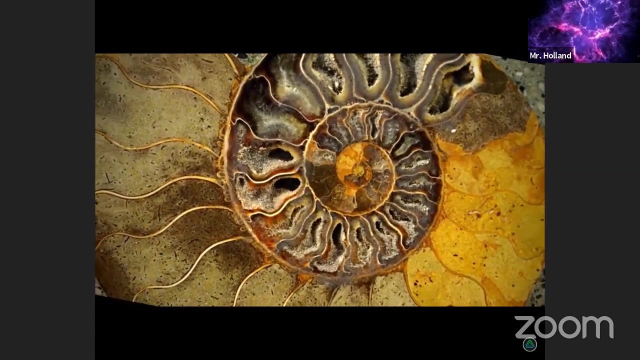 This was already evidence against the asteroid system. The asteroid impact would have brought the Sun and caused temperatures to fall rather than rise. On top of that, an asteroid impact would cause an extinction really fast, While the fossil record suggests the Great Dying was smeared over at least 150,000 years of time. 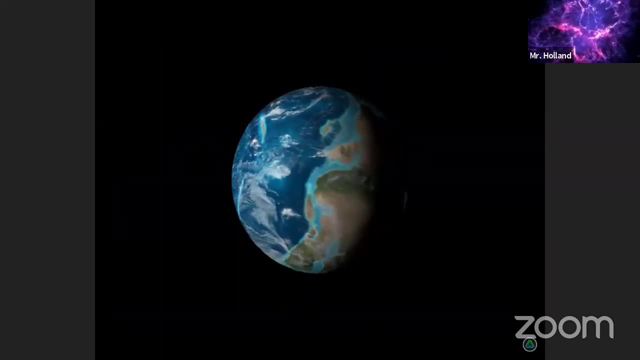 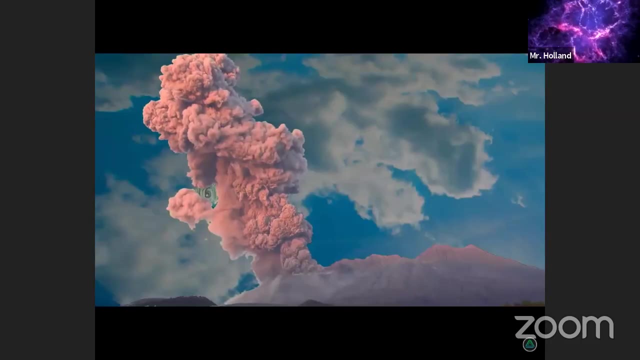 the next most obvious target could be something not from space, but from the Earth itself. Volcanic activity has proven to be capitalistic. Before a volcanic cause, the Permian extinction would have taken place. After the Permian extinction, there would have to have been some unseen magnitudes of it. 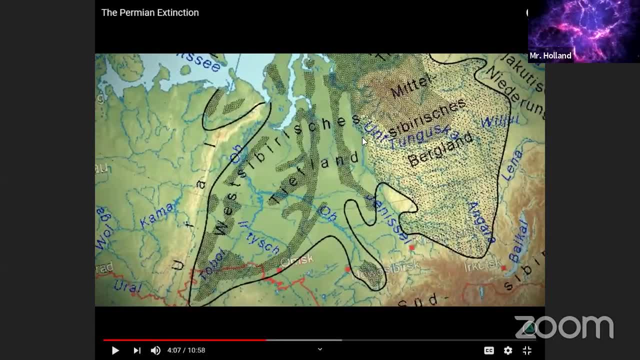 Enter the Siberian Cracks. Siberia now is a large region of Russia. This entire area here was believed, at least by this researcher, to have turned into a giant volcano. The entire area filled with just molten rock magma It was spewing out onto the ground. 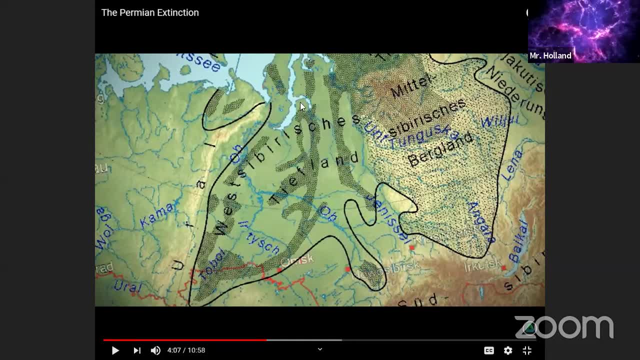 And as it did, it was putting up a lot of gases to build it, And his hypothesis is that these volcanoes at the time are what initiated the sequence that began the climate change that wiped out almost all life on Earth. We'll go ahead and stop it there. 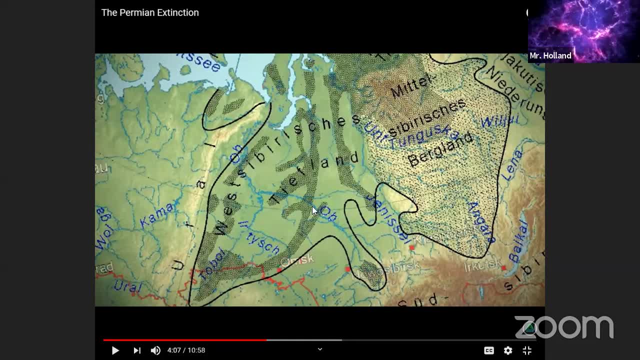 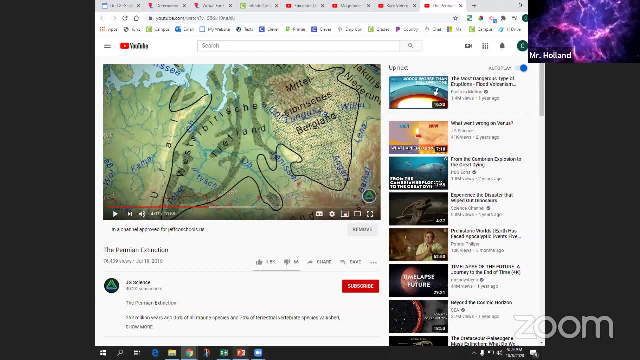 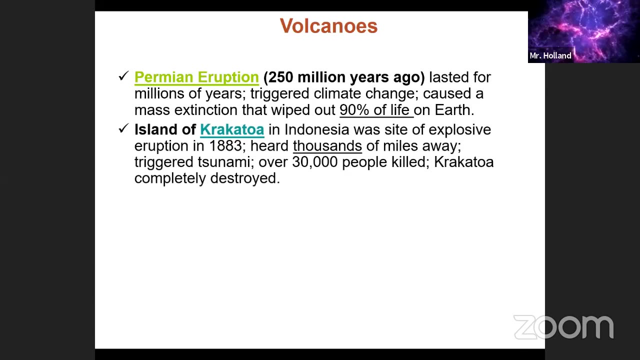 It goes on. He just goes into more of the detail as to why he thinks that was the case in supporting his hypothesis. The next big earthquake was called the Great Dying. It was a big earthquake. It was Krakatoa. Krakatoa is kind of an interesting one in that the island of Krakatoa in Indonesia basically completely got destroyed. 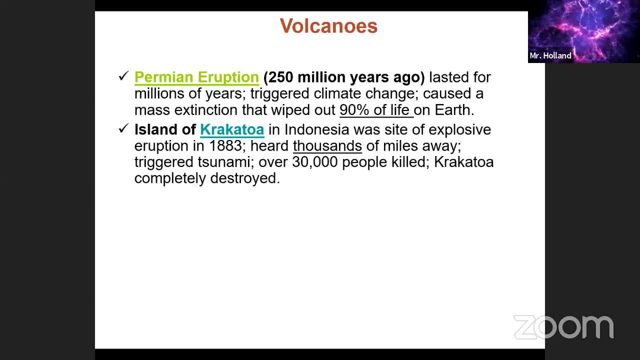 The volcano erupted. It shot the island up into the air into little pieces and it rained back down into the ocean, disappearing. It was also heard thousands of miles away, which at the time there were no sounds that could be heard that far. 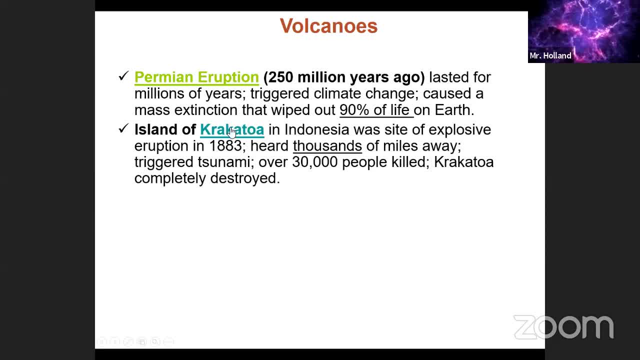 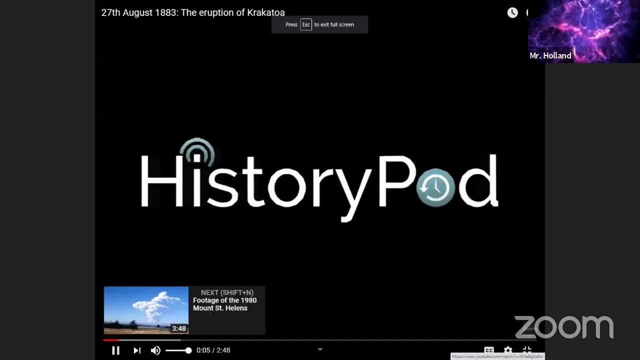 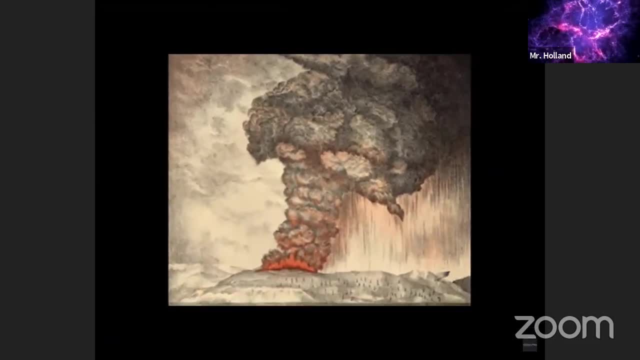 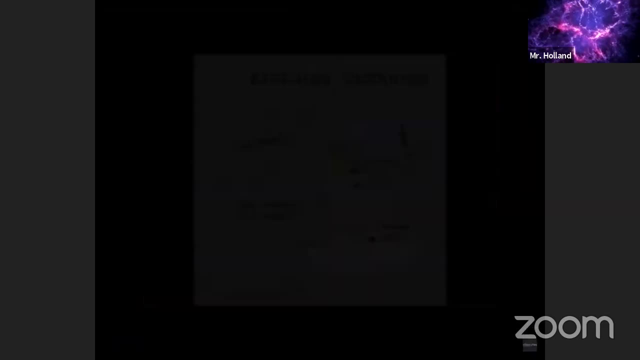 And it was kind of impressive. Let's see what we have. This is all reenactment. There was no footage, I don't think at the time. Hello and welcome to History College. On the 27th of August 1883, one of the most destructive volcanic events in modern history occurred when Krakatoa's eruption reached the climate. 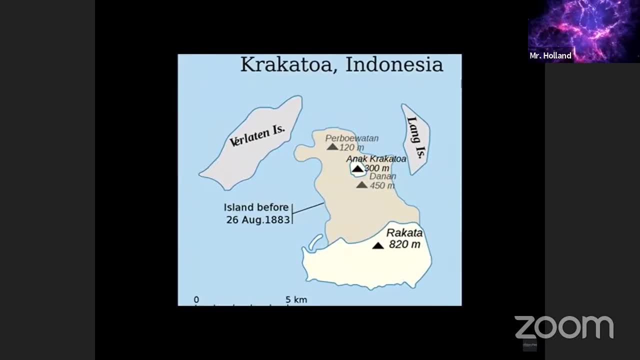 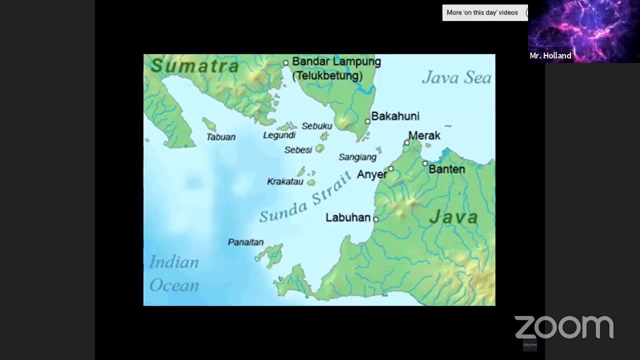 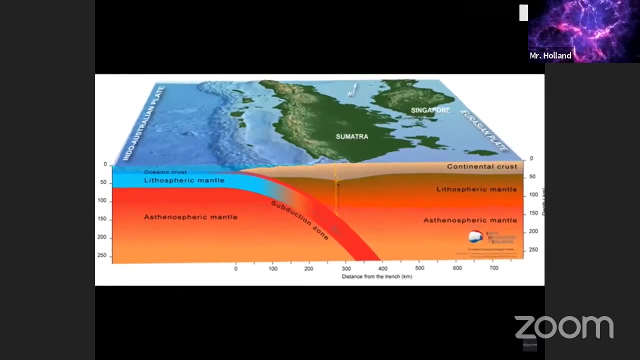 Krakatoa consists of a mostly sunken caldera that lies within the Sunda Strait between the Indonesian islands of Java and Sumatra. Situated on the subduction zone of the Eurasian Plate and the Indo-Australian Plate, the island and its surrounding archipelago were formed by previous volcanic eruptions. 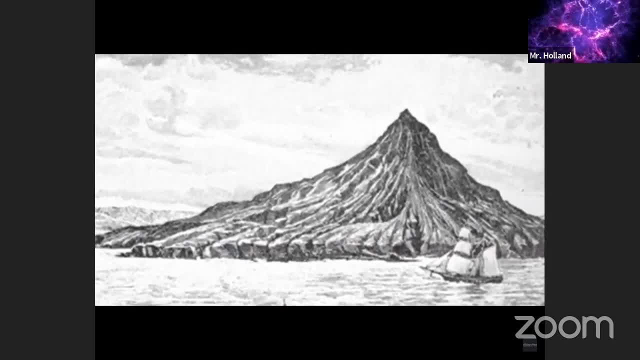 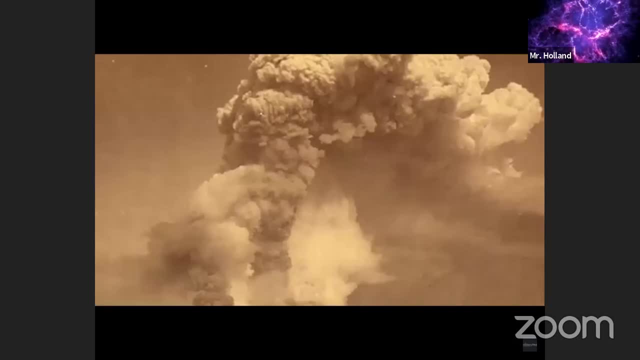 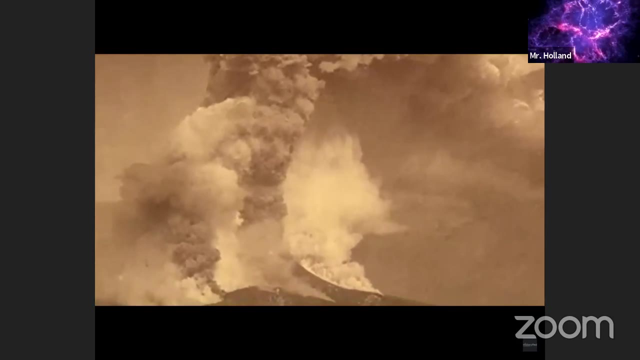 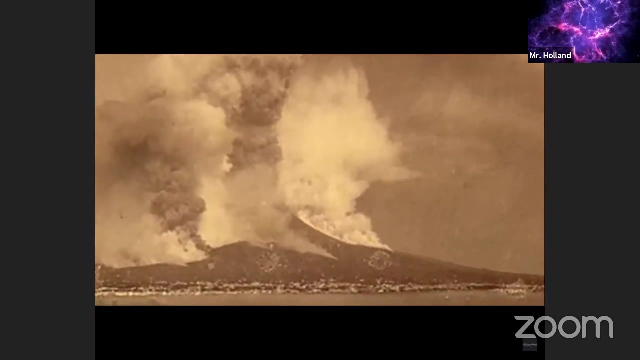 In May 1883, clouds of ash and steam were seen venting from the volcano by the captain of the Elisabeth, a German warship. The intensity of the volcano's activity varied Over the next three months until on Sunday, the 26th of August. the eruption became significantly more violent and debris was thrown an estimated 15 miles into the air. The earlier celebratory mood of people on the nearby islands soon turned to fear, as hot ash and rock began to fall. The eruption reached its climax the next day Over the course of five and a half hours, beginning at 5.30 am. 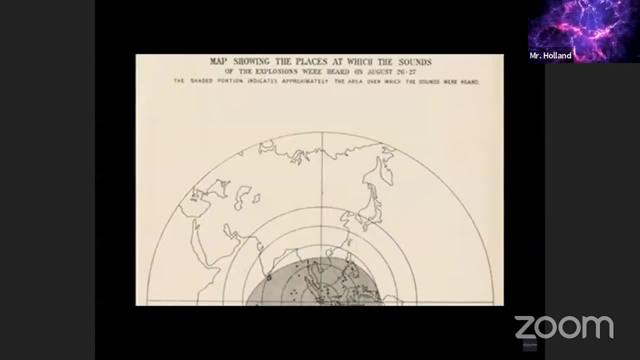 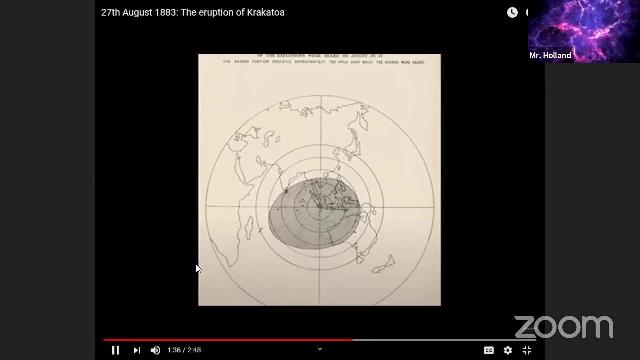 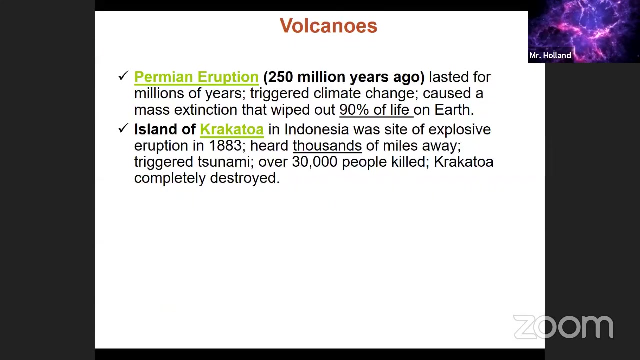 four enormous explosions occurred. The third of these was the most powerful, with the sound being heard up to 3,000 miles away in the Indian Ocean. Let's stop it there. The third and final eruption I want you to be aware of is probably one of the more famous ones: Mount Vesuvius. 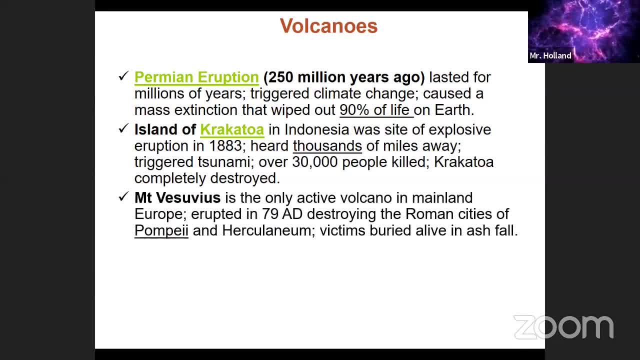 In Italy, the town of Pompeii was completely buried by this volcanic eruption in 79 AD. The people at the time were having their morning breakfast When the eruption happened. this ash cloud came out, traveling at super, super fast speeds- 100 miles an hour. 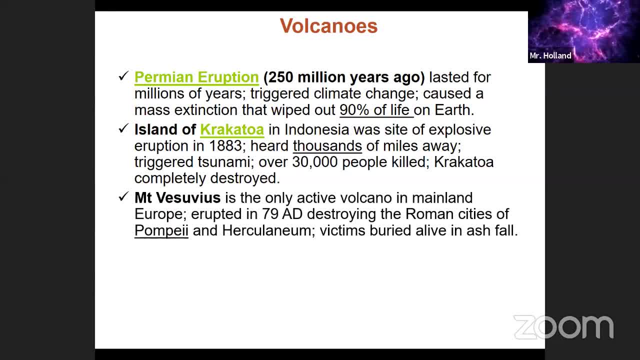 and it overtook the people before they could even react. They were buried in the ash rock, locked in the rock record, and have since been excavated by scientists, where you can now go to this village and visit as a tourist, and you can see the fossilized remains of the people that were sitting down for their morning breakfast. 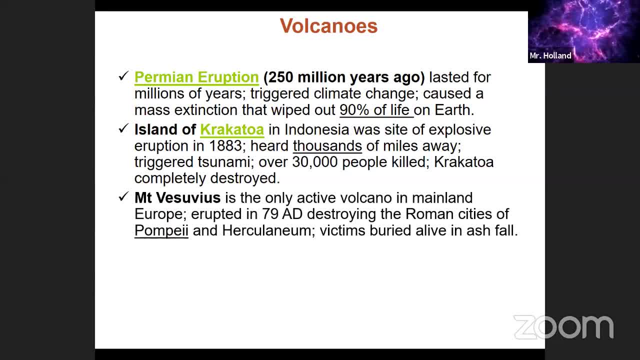 There's a dog begging for treats at the lower portion of the table. Others were in their beds still because they were asleep. It was morning time And they've unlocked what the life was like in 79 AD because it was completely trapped in the rock record. 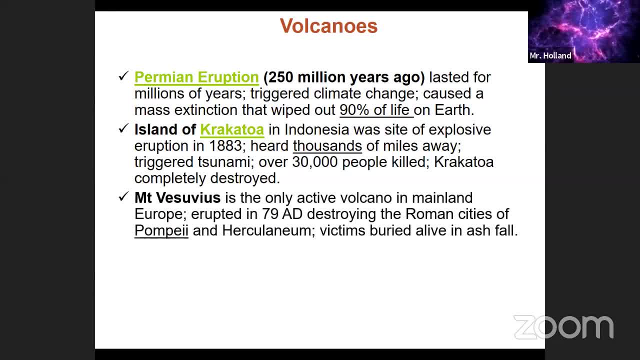 So, historically, it's kind of a cool area to see what life was like and what people did at the time. For them at the time, though, it ended instantly with that eruption, because their village was right next to Mount Vesuvius. All right, the Ring of Fire. 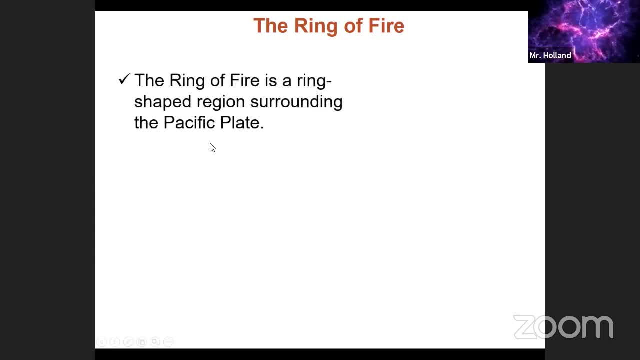 This right here is an impressive and important part of the Pacific Plate, because around the Pacific Plate is where a majority of seismic activity occurs. It goes up the coastline of South America, North America, across to Eurasia and down along the Pacific Plate boundary. 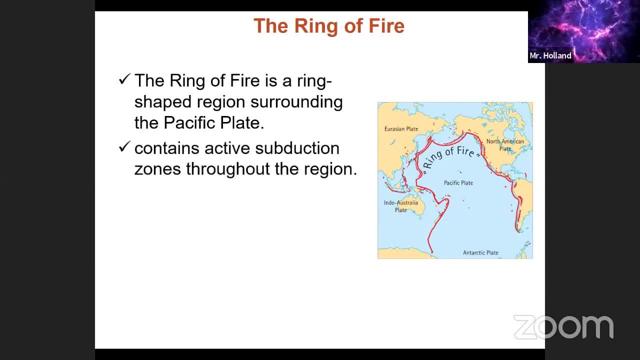 This is important because there are subduction zones on either side of this plate along our coastline- South America and the other side. Because of that, there's a huge amount of seismic activity. It is the home to 75% of the world's volcanoes and 90% of the world's earthquakes. 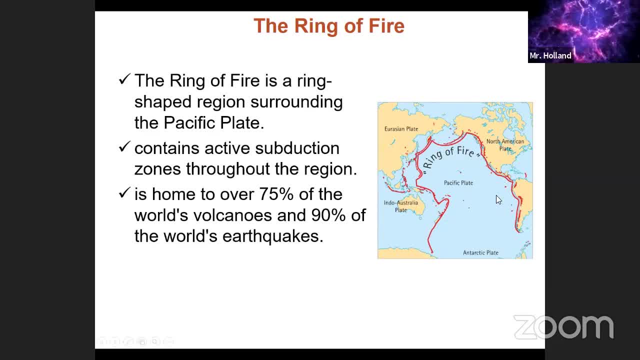 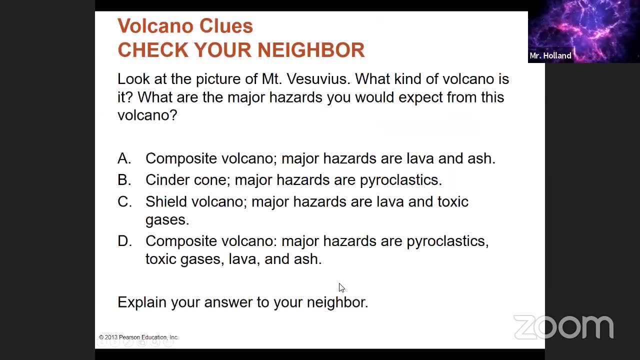 Hugely seismic in this general area right here. So that's why we say when most of this stuff happens at plate boundaries, it's because of the Pacific Plate boundaries, where the subduction zones are, of why that is. Our last natural disaster is the hurricane. 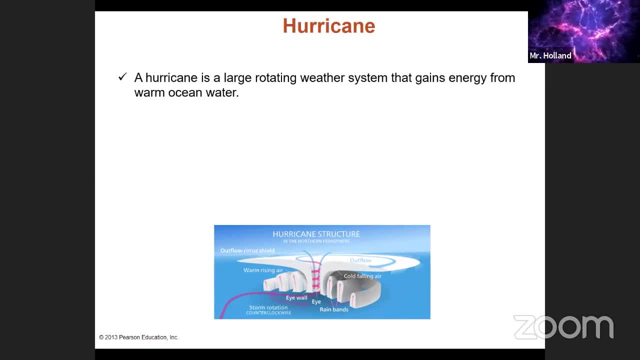 The hurricane is a large rotating weather system that gains energy from the warm ocean waters. If you don't have warm water, you don't have a hurricane. You've got to have the warm ocean waters to create the hurricane. You need winds that are sustained of 74 miles per hour. 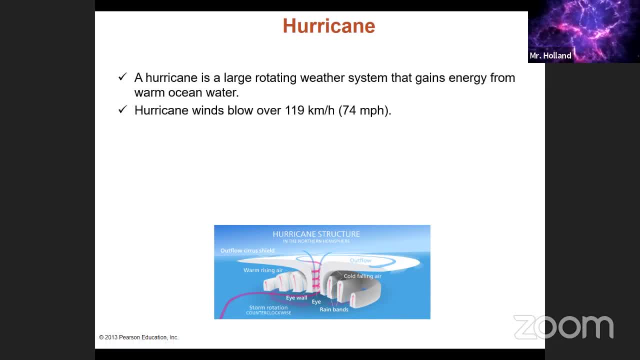 192 kilometers per hour consistently is what is required for a hurricane, For example. here we get winds that can give you as much as 100 miles per hour gust, but then it slows down right afterwards. These winds continue and don't slow down. 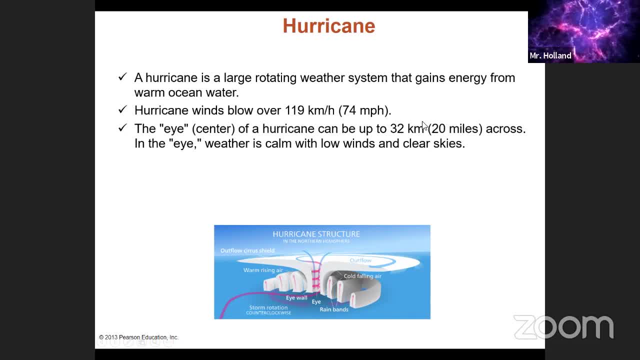 The eye of the hurricane, which is the center, can be as much as 20 miles across 32 kilometers. It is a very calm region of the storm: almost no winds, no rain, sunny skies. It's a very nice place to be. 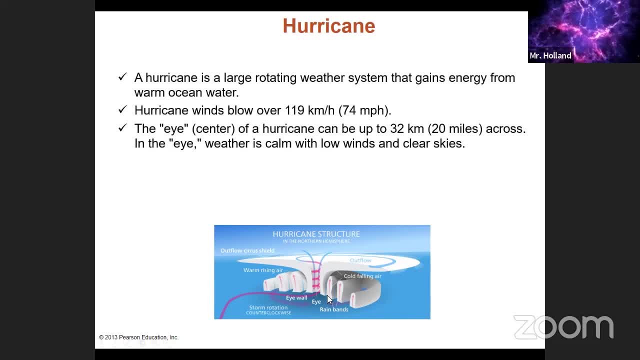 However, right next to the eye is the eye wall, and the eye wall is the most dangerous place to be. Vastest winds, most rain, most destruction and damage happening right here. The storm surge is what causes the majority of deaths in a hurricane. 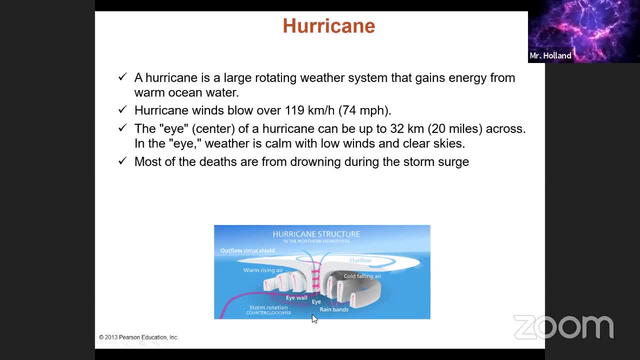 This hurricane swirls around in a counterclockwise fashion. So as it approaches land, just like this tsunami pulls up the wave bigger and bigger and bigger, right before it hits the coastline, the hurricane does the same thing Because, as it's swirling in a counterclockwise fashion, as the hurricane hits, 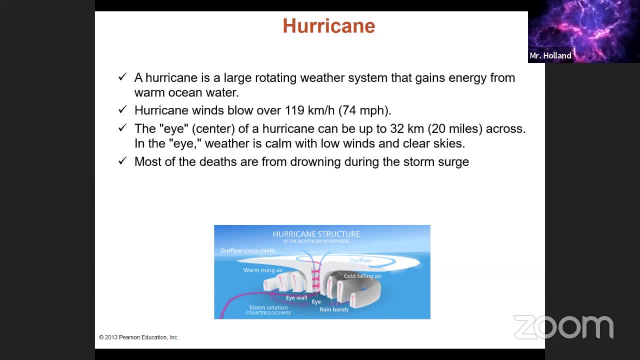 you're on the east side of the hurricane. It's pushing the ocean current and water up onto the land. It's called the storm surge. The other side is the opposite: It's pulling it away from the land and it has a low, low tide there. 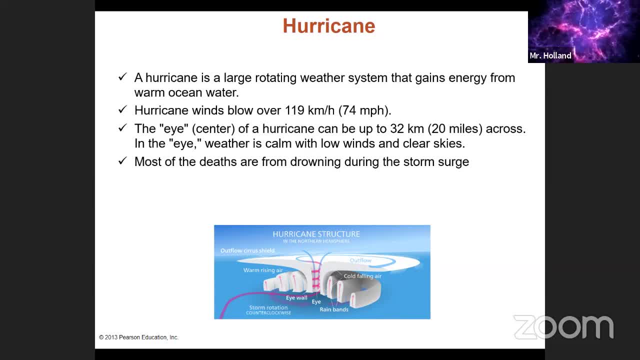 So if you have a high tide at the same time the hurricane hits, it is extra devastating because you've got the high tide beginning higher ocean and you have the surge on top of it. Hurricanes, once they come on land, will weaken rapidly. 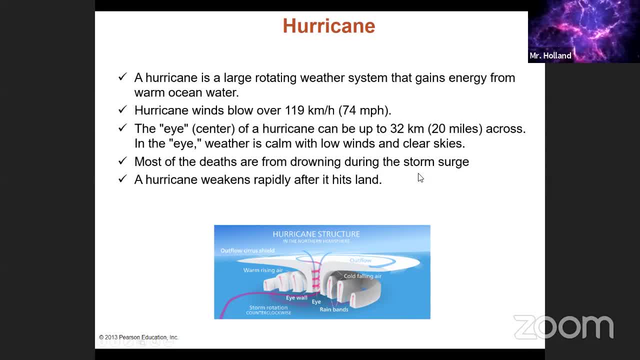 They don't take long for them to go down to a tropical storm, a depression, and then they're gone Because they no longer have the warm ocean currents and water to fuel them. They have to have that warm ocean water. The intensity of a hurricane is measured through a Saffir-Simpson scale. 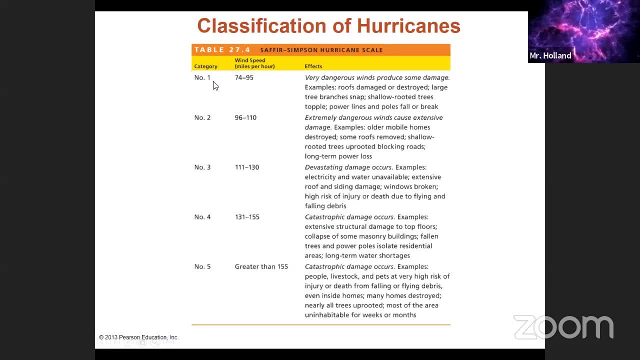 You probably haven't heard that name before, But you've heard of things like Category 1,, 2,, 3, and Category 5? The biggie On a five-point scale. it's all based on the wind speeds that are sustained within a hurricane. 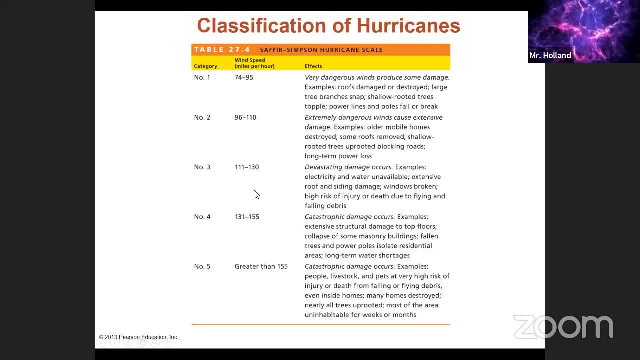 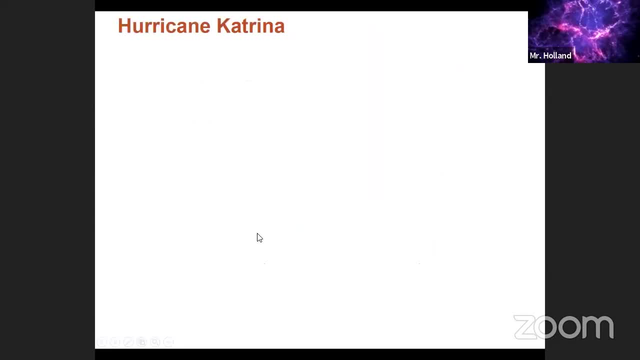 Constantly blowing- not just gusts, But constant wind speeds- dictates the size of the hurricane. as far as the category, Katrina is probably the most famous hurricane, Primarily because it happened to Florida in the United States. It was a very costly, the most costly hurricane. 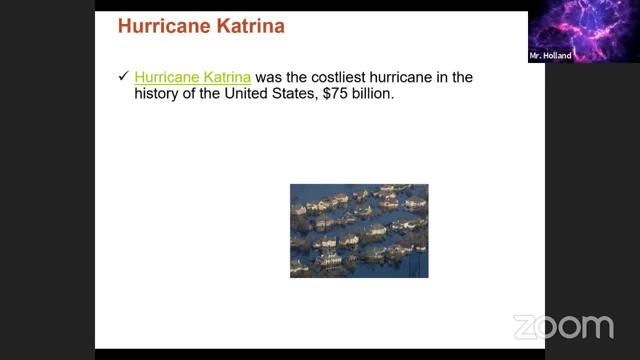 It's been updated now to be about- It's about to be- a value of $125 billion of cost for that hurricane. Over 1,800 people were killed during this time period And the winds at landfall were 125 miles per hour. 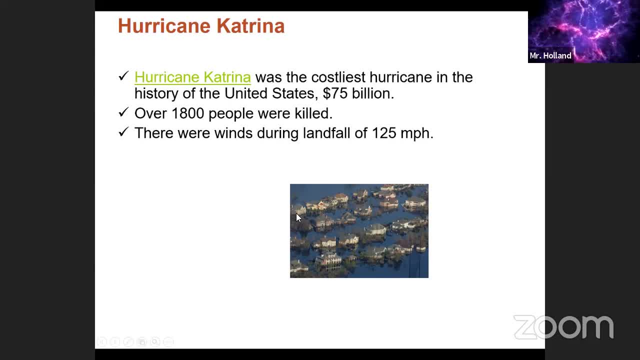 When it was a Category 5 approaching land, they were 175 miles per hour. So very, very strong winds coming right at you, Coming right at New Orleans, And since New Orleans is mostly 80% underwater or, excuse me, below sea level, 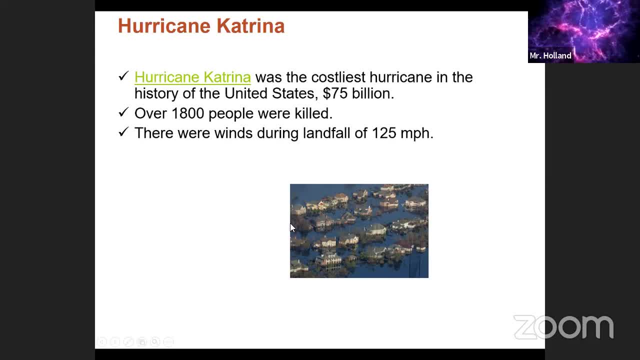 as the levees broke, the sea rushed in and flooded almost the entire city Up to someplace, as they said, 20 feet deep with ocean water. New Orleans is surrounded on one side by a lake called Pontchartrain, The Mississippi River, on the other side, further down. 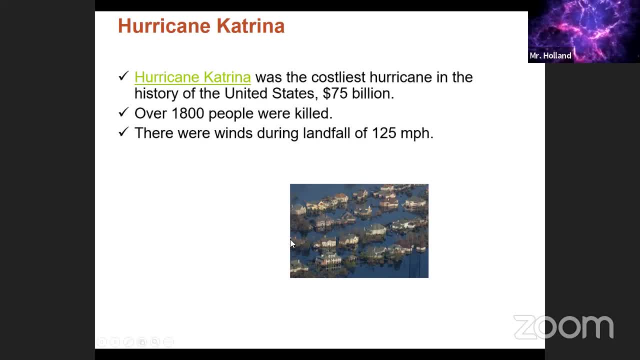 All the water around it just filled it up and caused the damage. People that could not get out of the town were sent to the Astrodome And there was an overwhelming amount of people there. They didn't have enough food or water supplies for them for a couple of days. 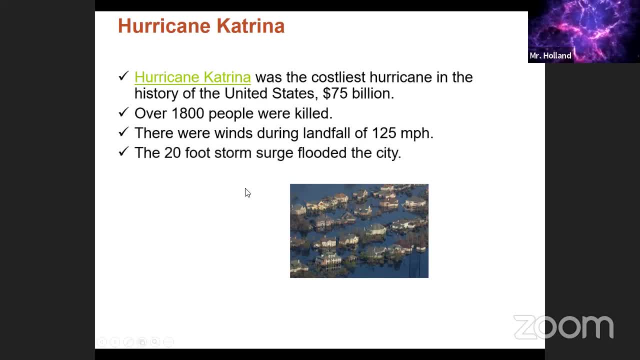 It was just a bad, bad situation. This one had a 20-foot storm surge. That's huge for a storm surge. The ocean was 20 foot higher on the east side of it hitting than it normally would have been, And that extra 20 foot of water to something that's built below sea level. 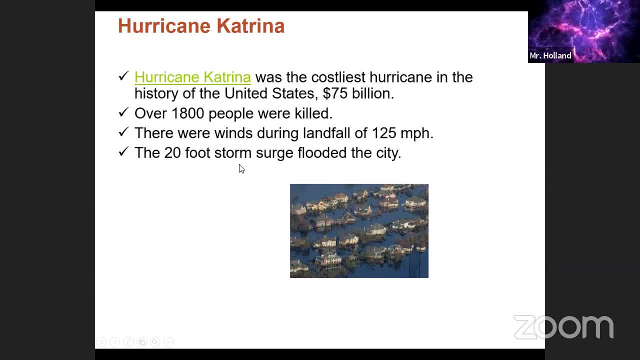 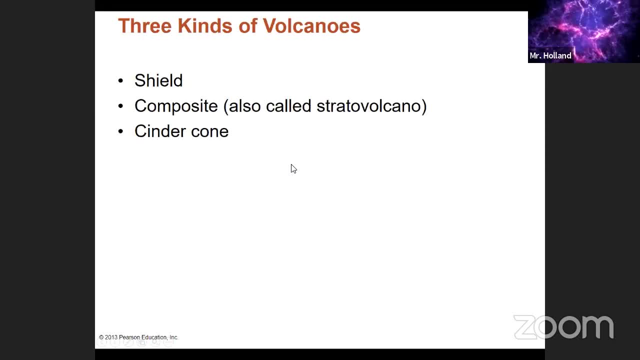 just caused the severe damage to take place. It couldn't withstand that extra amount of ocean. I think that's the end. All right, that wraps it up. That was a long class period. Usually these will be spread out over a couple of days, with breaks and things. 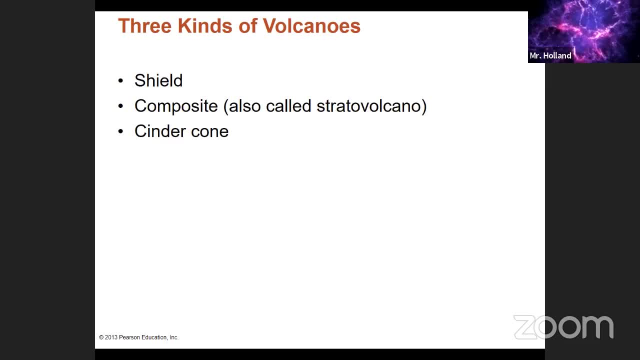 I just want you to know that one day is not good. Go ahead, Matthew. Thank you. Well, 3 days- we said 3 days here, Obviously always again that same time. very fast, you did a good thing. 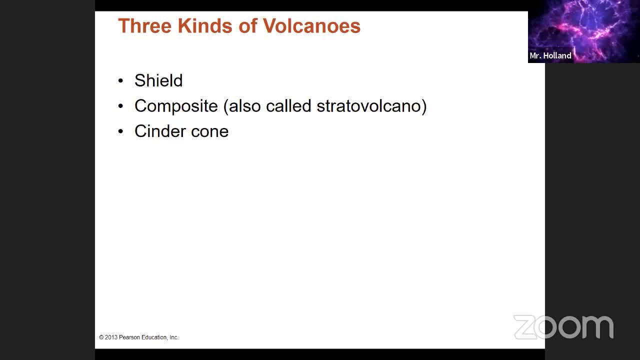 You were a pretty good person And you already go ahead and take these things and take out 5 of these things and put them in your own, Get it through your mouth And all these things are kind of hard on the looking kind of way. 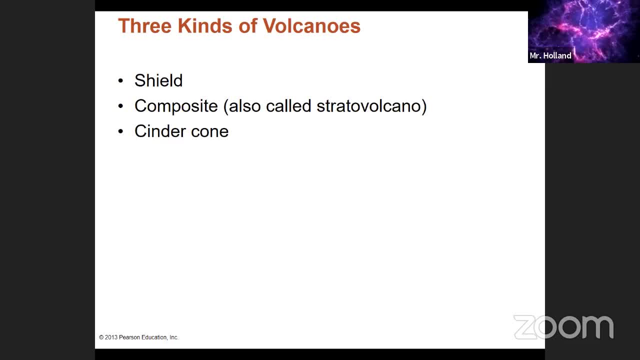 because for most people who have video stuff and you can't watch the video with these things, I mean I do like iPad, Oh, and a box So you can take a picture of it. Oh, okay, gotcha see that box. that was good for that guy. okay, good. 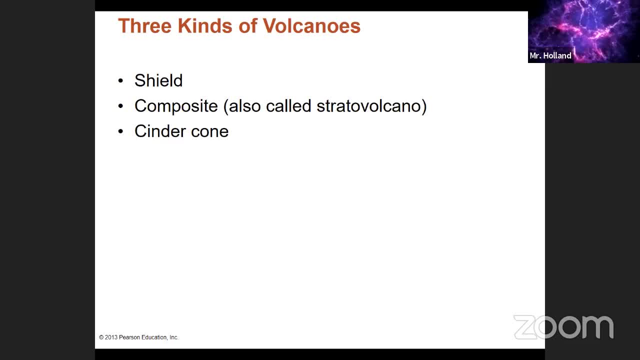 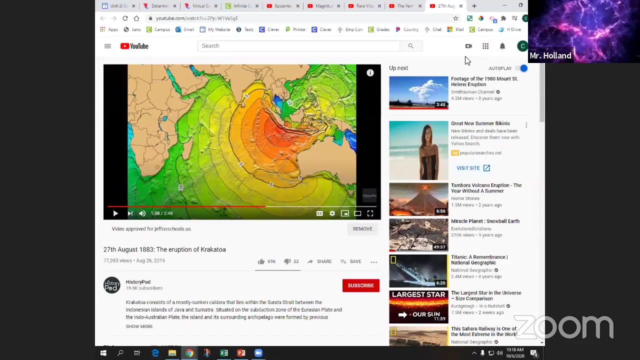